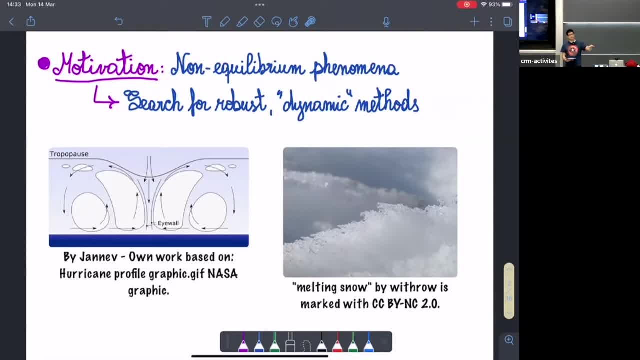 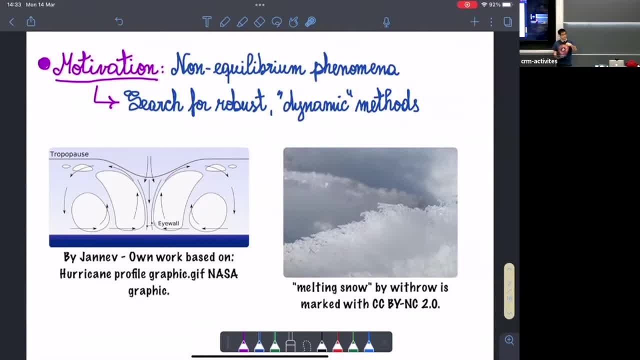 Okay, so the non-equilibrium situation is: it's reversed to this invariant state—was exponentially fast, but the secret is on the constant, on the exponential. there, Right, The constant is astronomically large, So it's not really getting there in the timescale. 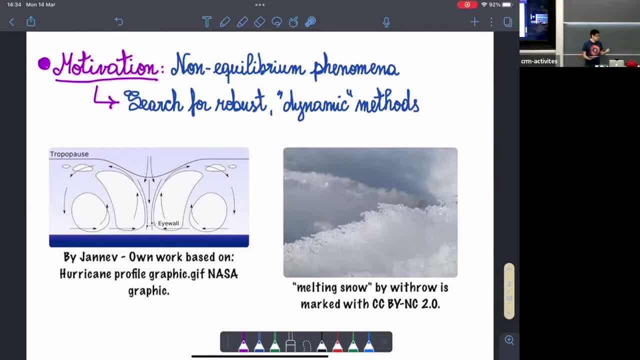 at which we are interested in. Now. that one nice example of an equilibrium situation. there are other examples, So here in this graph I put two examples. So the first one, Uh-huh, So that it's a hurricane profile, okay. 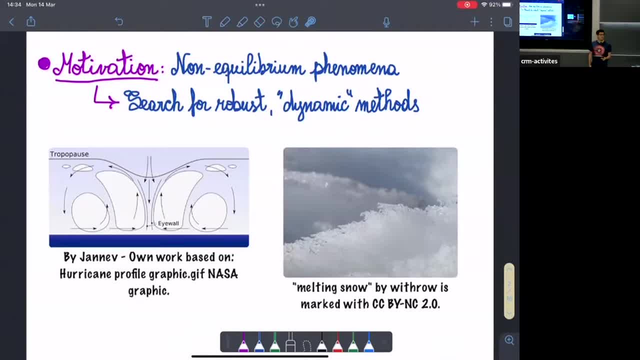 So it's a two-dimensional slice of a three-dimensional hurricane And it turns out that from the, in a very vague sense, a hurricane is the stationary object. okay, Because what hurricane is doing is that it's connecting. you see there, the tropopoles. 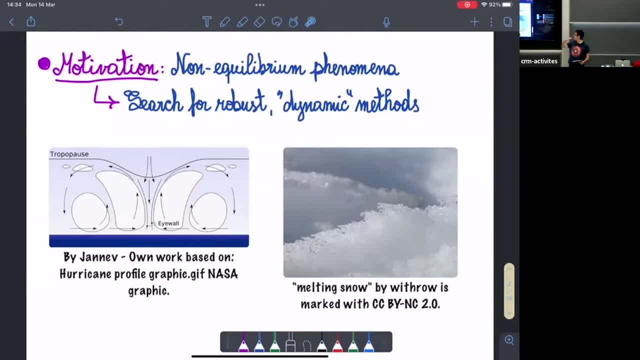 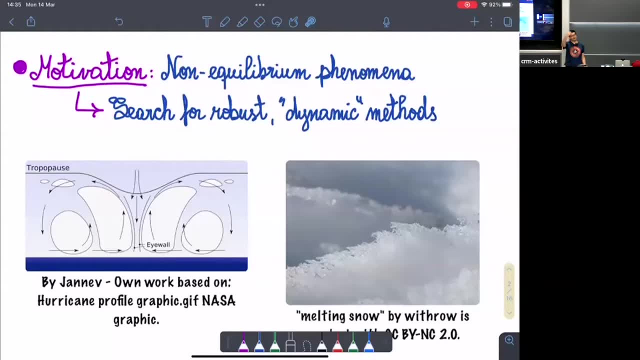 and so it's like at the beginning of the stratosphere, with the sea. So the sea is a heat reservoir and this hurricane is like a tube connecting these two guys. okay, But instead of having this picture, we have in mind about 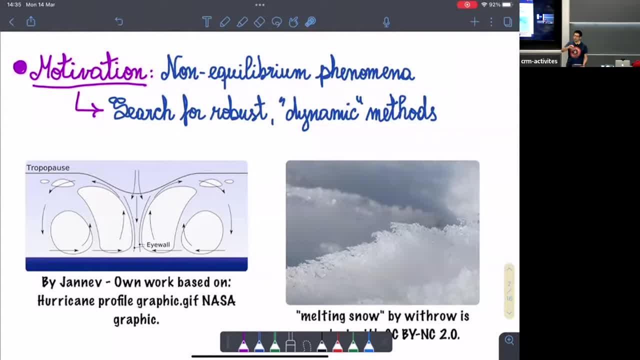 for example, a bar connecting a coal to hot and heat flowing in a natural gas, a nice and order way from one to the other. what we have is a hurricane, okay, Which is a very not the order way to connect these two heat reservoirs. 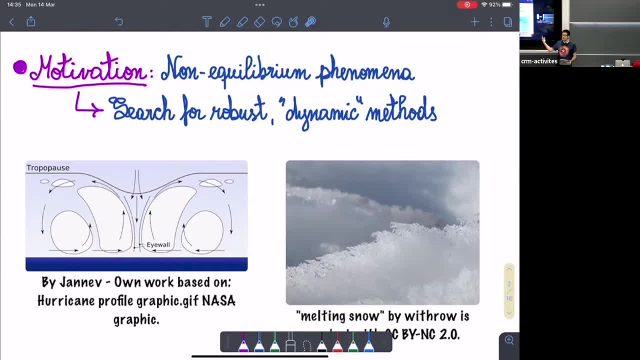 And what happens there is that, of course, instead of having an ice tube connecting these two guys, you have a hurricane, because a hurricane is more efficient. Okay, So that's the. that's something that somehow we need to understand, that. 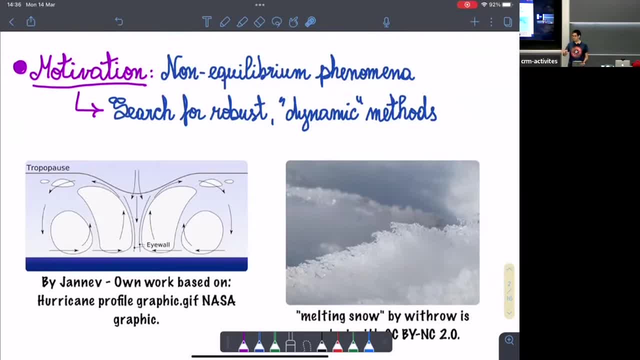 non-equilibrium stationary states, okay, things that are stationary but not in equilibrium. you know, this is a very vague sense. So a hurricane is clearly not in equilibrium, right? Because, okay, it's a hurricane And these objects, they have this tendency. 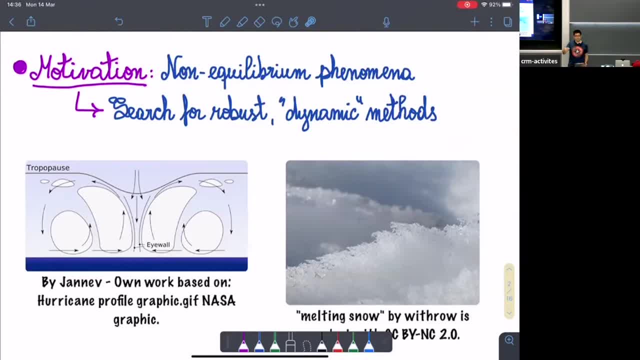 to do the job better than equilibrium stationary states, And this is those type of things are the things that we would like to understand. Okay, So I put here another example of a non-equilibrium stationary state: melting snow. So this is something we experience every day here in Montreal. 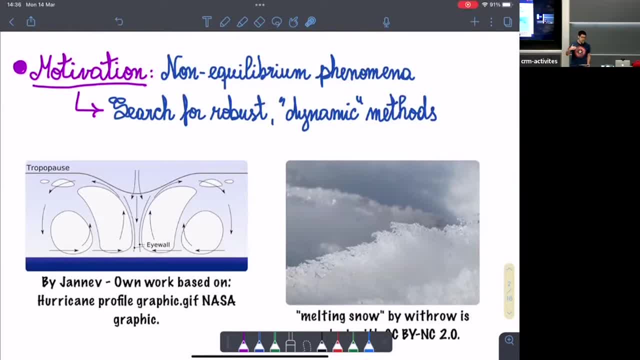 And it's again. it's not like melting ice, right? So you have ice and then ice melts and it's soft, nice order. You get some liquid getting out the heat, et cetera, And then you can put an equation to that. 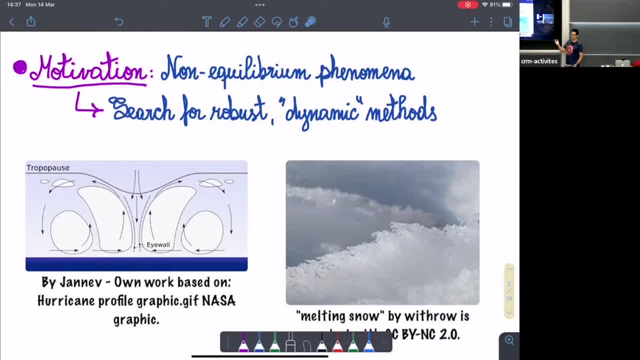 Okay, You can do that at PDE. So people call it the Stefan problem. maybe That's just kind of well understood. But here you have snow, and snow is different. It's more complicated, Okay, So non-equilibrium phenomena are everywhere. 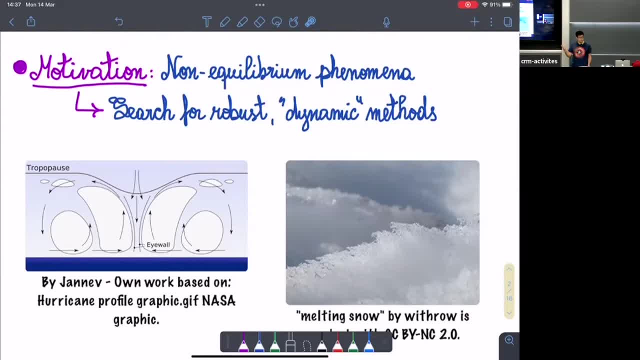 in the real world and are poorly understood from the point of view, from the mathematical point of view. So we really want to understand that And, as a mathematician, what you do is that you start to simplify your problem until you get something that you can actually solve. no, 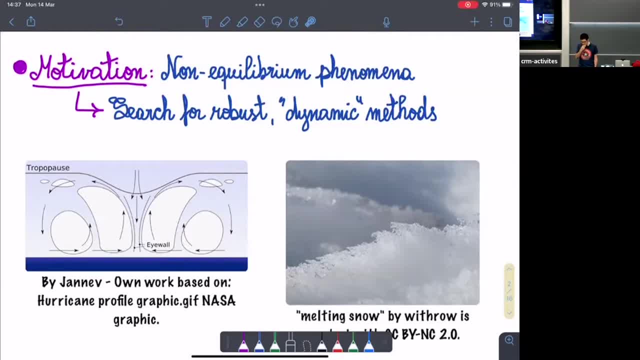 And that this is our aim- is to give an approach that somehow makes sense for us as mathematician to this non-equilibrium phenomena. Okay, So we're in this search for, in a sense, robust and dynamic methods. Okay, Because something which is more or less clear is that dynamics- 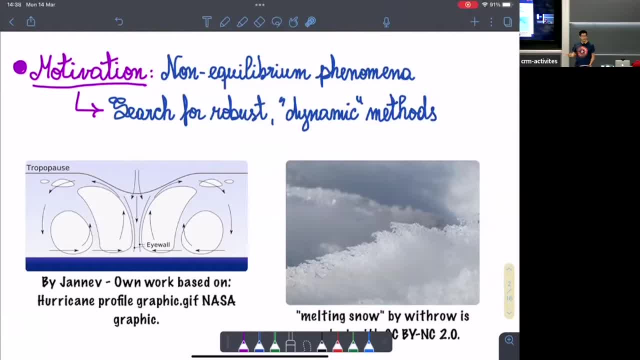 dynamics, aspects of non-equilibrium phenomena are important. you cannot just describe the stationary states of these guys and get the information you want. you see, we've already seen in Christina's talk about this- kinetically constrained models- that the stationary states are extremely simple, just a product of Bernoulli measures, so something which is absolutely well understood from that. 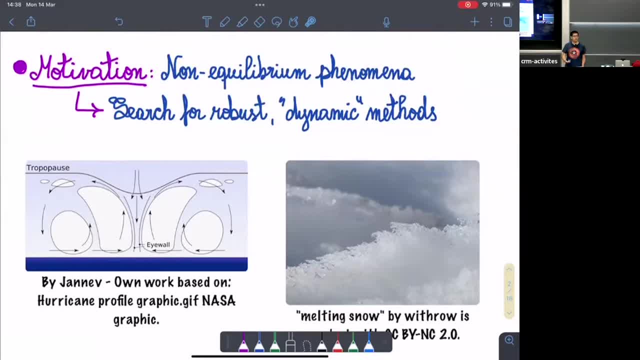 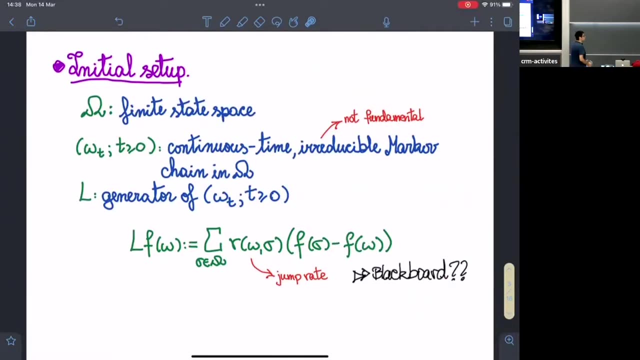 point of view, but the dynamics, it's a completely different business. okay, so well, we have these two examples, and so, so let me go for the setup now. okay, so, what do I call a non-equilibrium system? okay, so, actually, what we are going, what I'm going to call an equilibrium system, is something: 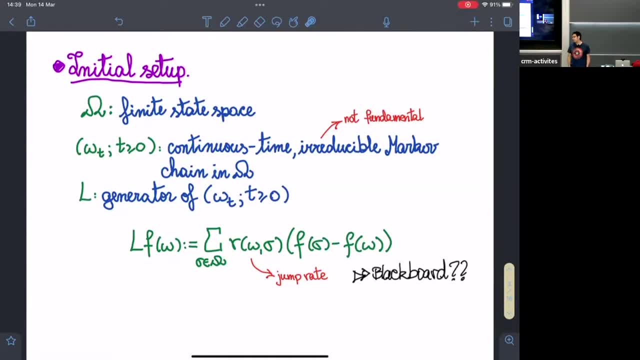 uh, very well known, for probably this is a finite state Markov chain. okay, a finite state Markov chain is what I'm going to call, somehow, a non-equilibrium system, and a non-equilibrium stationary state is the invariant measure of a Markov chain which is not reversible. that's going to be. this is going to mean for me. 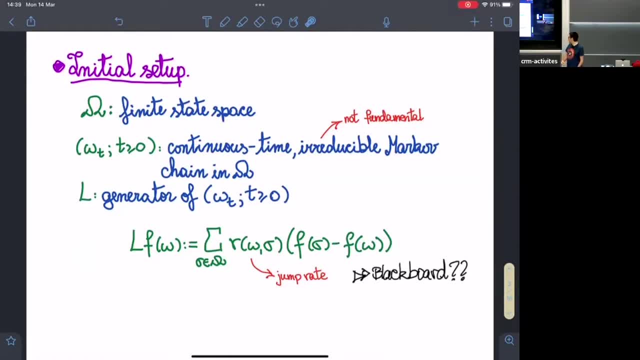 a non-equilibrium stationary state. okay, so maybe a quick, uh, I don't know. I hope people in the, in the, in the online, can see this, but this is. I just want to give a quick relational shock. what's the shock? ah, okay, thank you. okay, so let me just give you um. 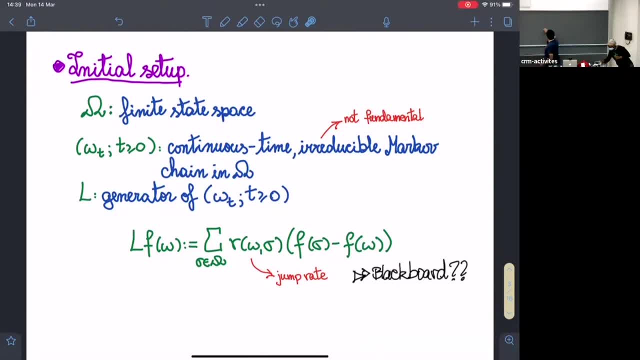 something a a quick, uh description of a non-equilibrium stationary state of a Markov chain. so so you have a Markov chain, so you, you have these points here, and then sometimes, because of the non-equilibrium stationary state of a Markov chain, you have a Markov chain, so you, you have these points here, and then sometimes, 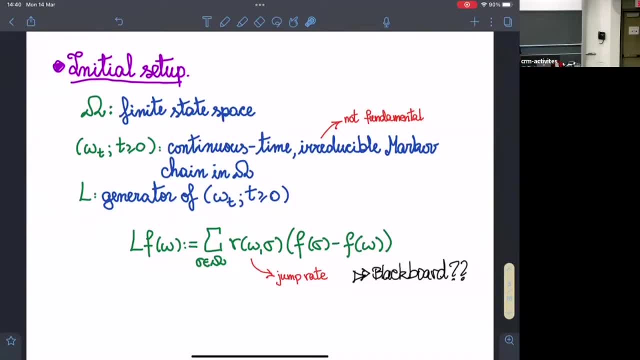 because this Markov chain is complicated, you don't know the invariant measure. but to actually show that the invariant measure is not reversible is easy, even if you don't know it. okay, because what happens is that if you find one loop, okay, one cluster circuit of allowed moves on your Markov chain, such that the probabilities 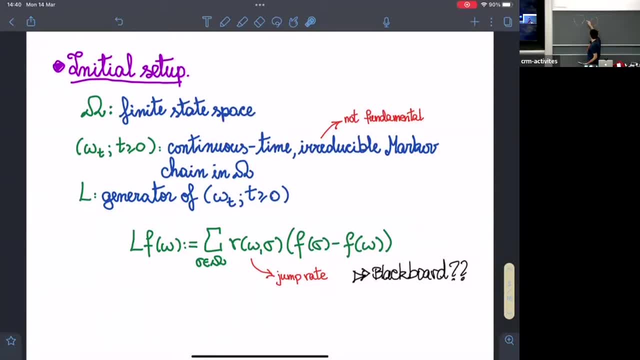 the product of these three probabilities here, for example, is different from the product of these three other probabilities here, then that implies that the invariant measure of your Markov chain is not reversible. okay, so non-reversibility is kind of easy to see, okay, um, so those type of situations, or the invariant 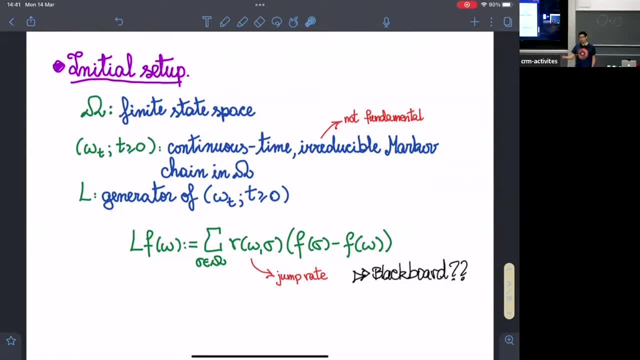 measures of Markov chains which are non-reversible, is what we are going to call non-equilibrium stationary states. and somehow, what? is that a sufficient condition? uh, let me see. so if this happens, then the, the, the, the measure is non-reversible, and if the measure is reversible, it satisfies this condition for two loops. it's called the. 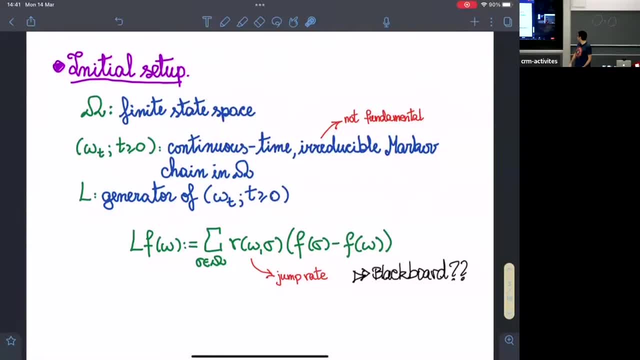 detailed balance condition. okay, so i don't know if that answers the question of for of Francesco, yeah, you go. so, ah, yeah, this is, that's an important remark. so this is supposed to be? um, just a moment, because, uh, some people at home have problems to see the blackboard. indeed, there is a line. 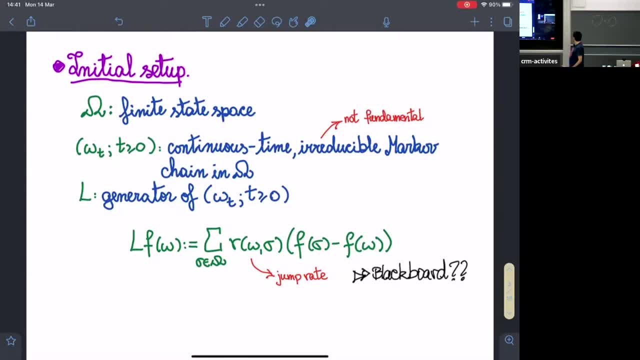 that you can move with the mouse and you can enlarge the, the picture with the uh, with the blackboard. i hope you have to pin the blackboard video yourself manually if you want to see the blackboard. okay, okay, okay, so, uh, please, yeah, yeah, okay, thanks, yeah, so okay. so that was for the audience, so 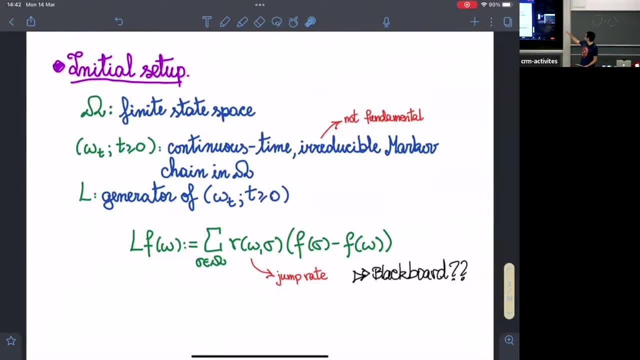 you can do it manually, you can. you can switch between the the two setups if you want to see the, the black or larger. okay, uh in, okay. so what i was saying is that the non-equilibrium systems are going to be Markov chains for us and a non-equilibrium stationary states. 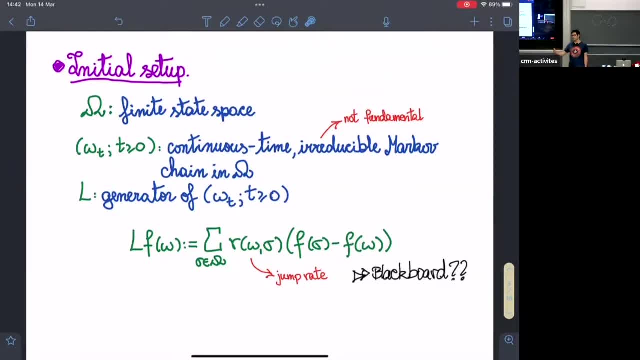 are going to be invariant measures of Markov chains which are non-reversible. so now we have a- at least we have translated this uh physical problem into a concrete mathematical problem, which is: we want to analyze Markov chains and we want to analyze their environment. okay, and 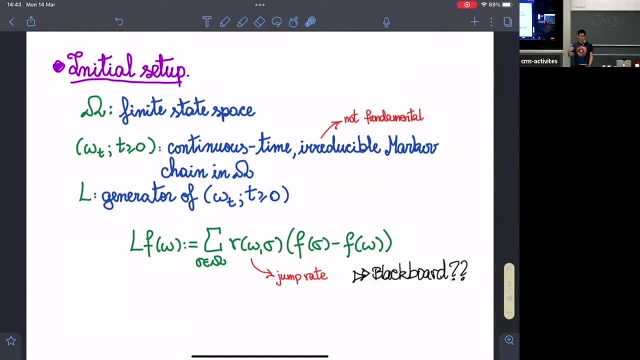 what i want to do is to try to set up some sort of a strategy that makes sense for any Markov chain, so in such a way that for your favorite Markov chain now you have at least a tool, one way to proceed that makes sense. This way to proceed may or may not be convenient for your favorite Markov. 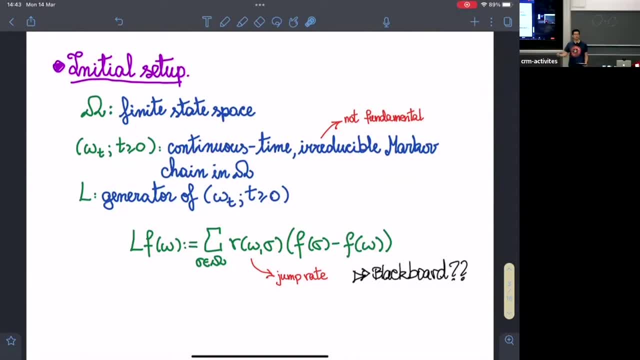 chain, but at least you have one more tool in your set of tools. okay, so now there is one more. so what is the setup now? So we have a finite state space, Omega. so No, no, no, no, oh sorry, yeah, So we have a finite state space. 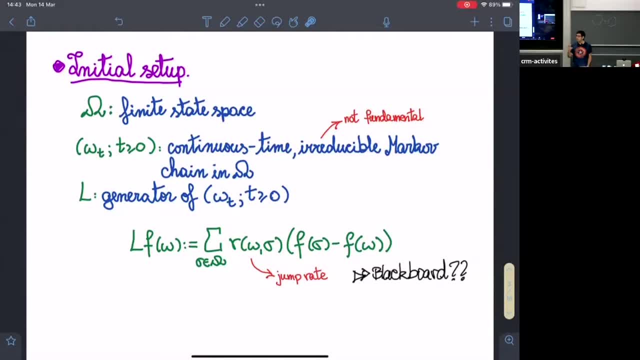 a finite state space omega. so here, in order to keep the technical problems to a minimum, i'm always talking, going to talk about finite state markov chains, because then you don't have to worry about infinities and and convergence and stuff like that. okay, so everything is going to. 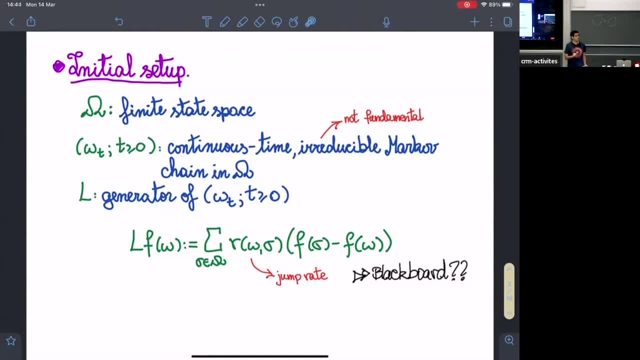 be finite, so everything is going to be well defined. so i have a finite state markov chain. now i'm going to call omega t, so this markov chain happens at continuous time and it has to be. i'm going to assume that it's irreducible, although it's not fundamental. 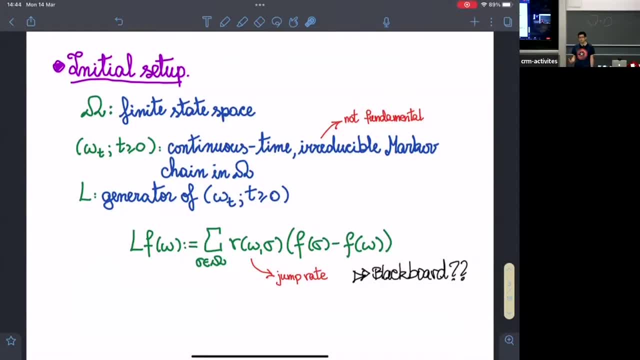 okay, so it might be not irreducible. in some situations and in some meaningful situations, markov chains are not irreducible and you can still try to apply this methodology that i want to introduce in this miracle, and so i'm going to call l the generator of the markov chain. okay, so, 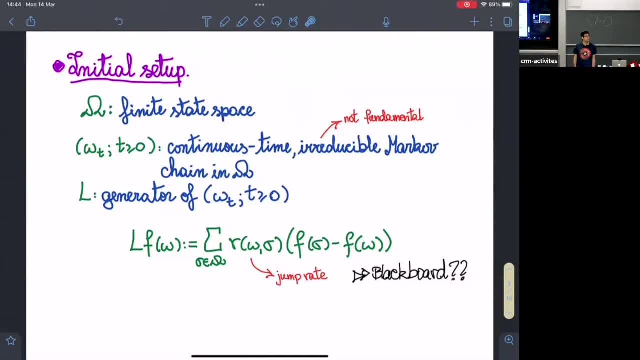 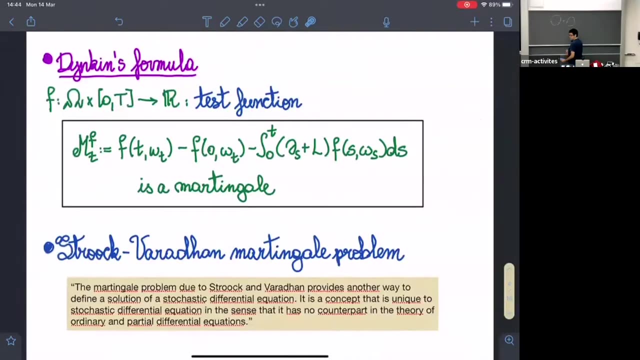 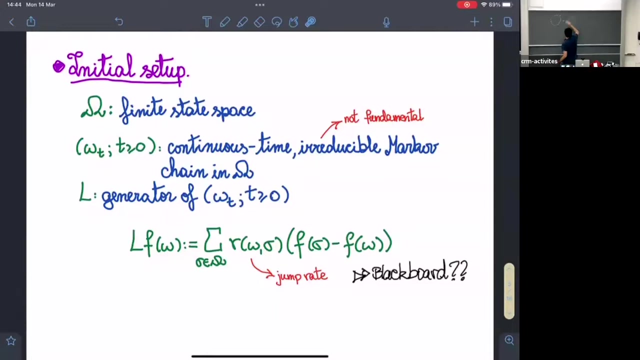 it's written there. so how do you, uh, how do you read that definition of the generator there? so, okay, blackboard, yes, blackboard, okay. so let's go to the blackboard and try to explain you. um, this is for later, so what does it mean? that l is the generator of your markov chain? 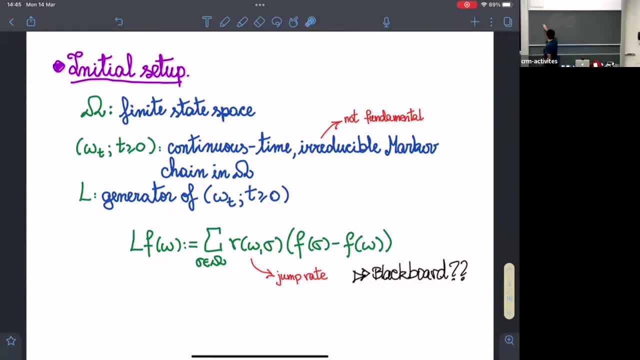 okay, so i'm going to uh take the advantage of being preceded by a christina and hendrik, which already talk a little bit about these things here, but uh, so let me show you how this generator thing works. okay, so you have a markov chain, so funny state. 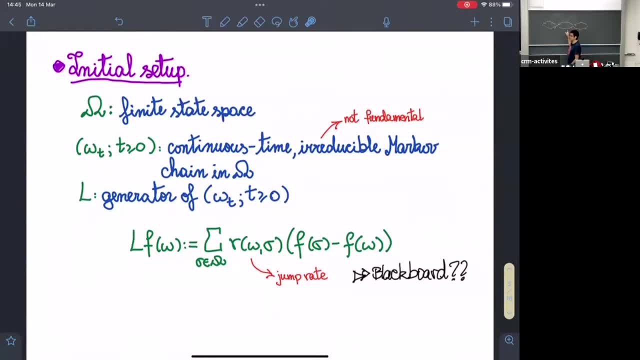 and what i drew here is the adjacency graph of the markov chain. okay, so here it means that, well, this is like a uh, it's a random work, so it's uh, you can go, uh, between neighbors maybe, or it could be another thing, and then you put numbers here. okay, so you. 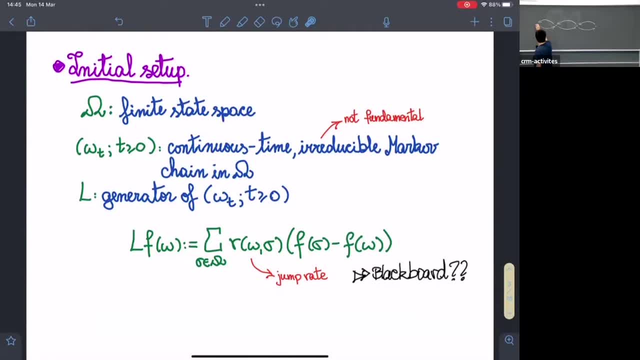 get, you can put here: uh, so if this is, um, if this guy is sigma and this guy here is omega, here you have a rate- sigma, omega- and here you have another rate, which is omega, sigma, which are different. okay, so what happens is that, um, if you are a sigma, 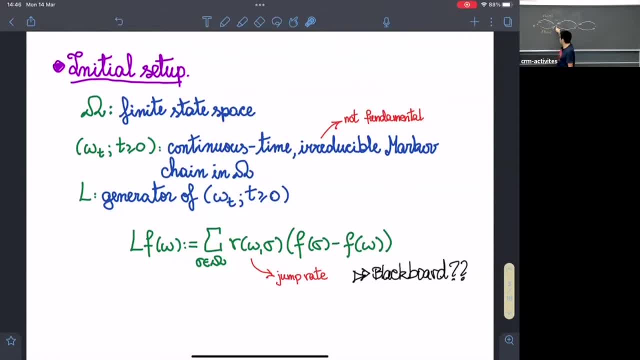 you live to omega with this rate, okay, and if you are omega, you live to sigma with this rate, and maybe here you have sigma prime and what happens is that you live from omega to sigma prime at a different rate, okay, so those are these numbers that you put on the generator. that's what they. 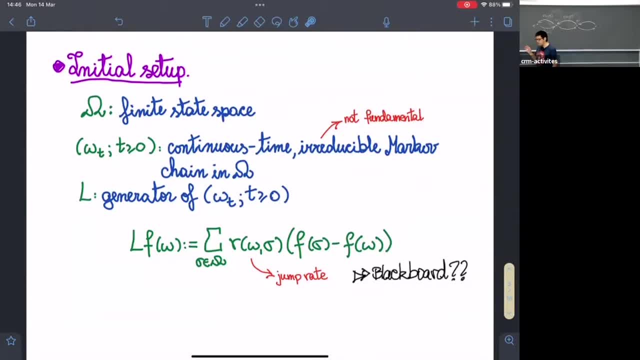 mean, and let us remember, if you don't like continuous time, you just can think about discrete time in discrete time. these are probabilities, no, so they have to add up to one and they tell you so that you are here and in the next step you go either here or here. 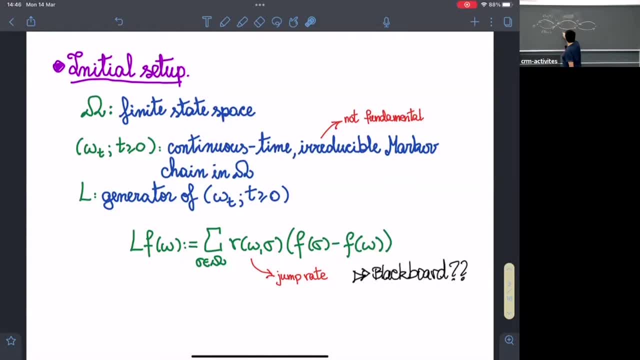 uh, so this is not. it's downstairs here is going to be out of omega, sigma prime, according to my design. so you go from omega to one of these two guys with probabilities which are you given by these numbers here. okay, so this is that discrete time mark of chain and those are the 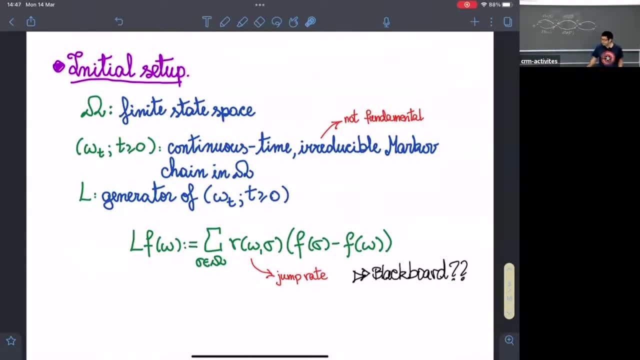 numbers are in continuous time. uh, what happens is that, instead of having um discrete steps, you have continuous steps that are given by, uh, Poisson clocks. okay, and what happens is that, at each one of these arrows here, you put an independent Poisson clock that will tell you what, when to jump, and the rate of this Poisson clock that is given by these. 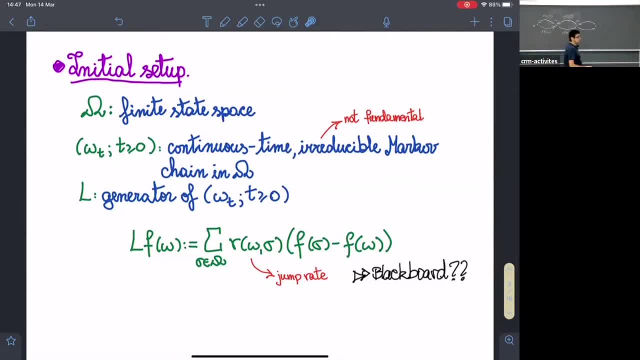 r's. if you don't like that as well, you can think in a in another thing, which is that omega D is actually omega of N of T, okay, where omega of N is a discrete time mark of chain and is an independent Poisson process, and that gives you omega of N. 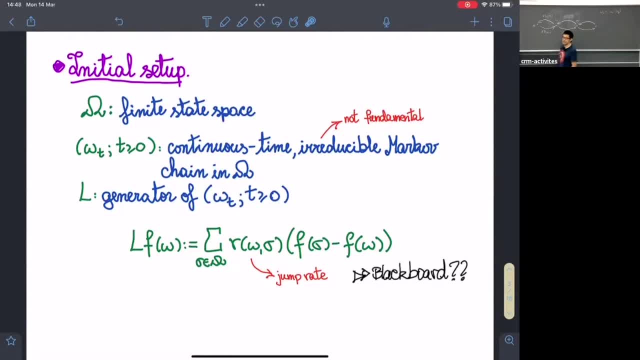 home process to your continuous time mark option. okay, So I hope that you understand what these R's are. So I guess that in the discrete time case are the probabilities at which you jump from. is the probability at which you jump from omega to sigma. 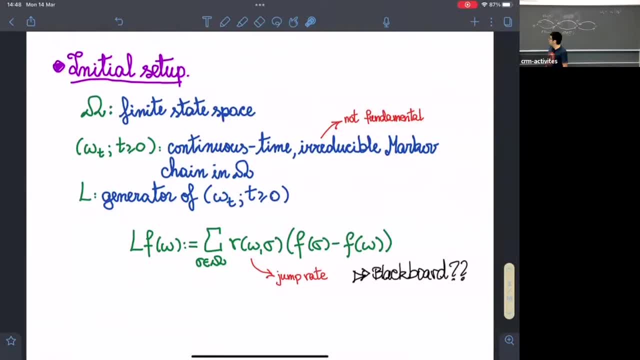 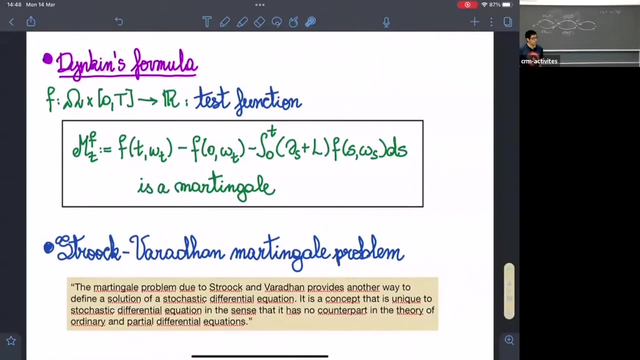 in that case, there, and in continuous time, is the instantaneous Poissonian rate at which you jump there. okay. And why do we define the generator? Because actually the generator is a convenient way to do computations, okay, So let me show you now the computations. okay. 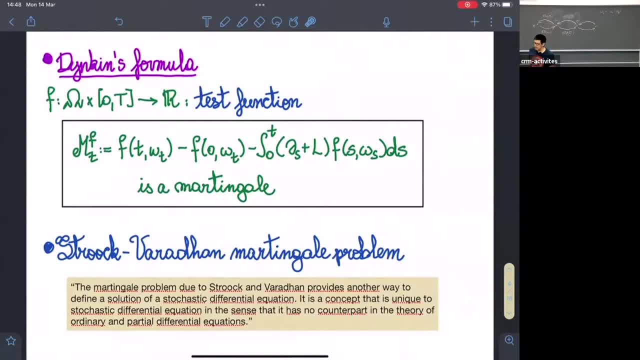 So what I want to do now is that everything that I'm telling you here is kind of elementary but a little bit non-standard in the sense that it's not what you see usually in a basic code of Markov chains. okay, So it turns out that you can formulate all 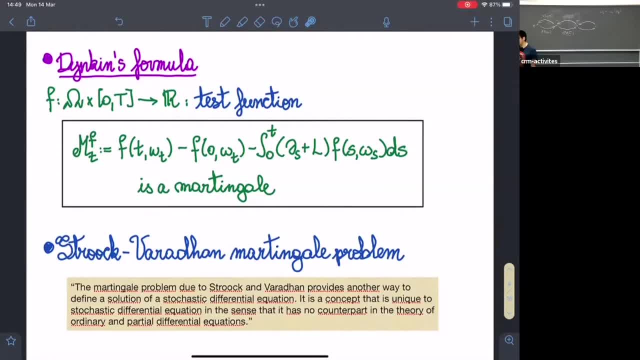 you can define, formulate all theory of Markov chains just using martingales. There is, this is done through what is called the Dinkins formula. okay, So Dinkins formula is what I wrote. there is the following: 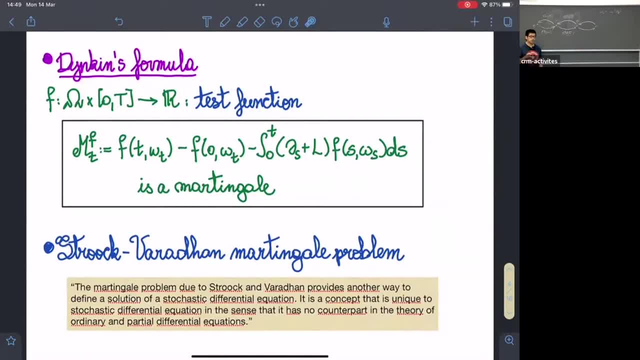 So for any function, f, which is a function, obviously, which is a function of f, which is a function of f of your configuration, of your Markov chain. So it could depend on time as well. I put there the dependence on time. 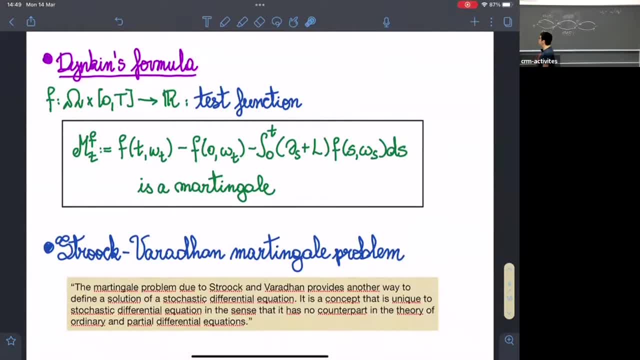 because in many situations it's very convenient to take also a function that depends on time And what happens is that if you take that process there, define this process empty of f, turns out to be a martingale okay, And you see that the generator is down there. 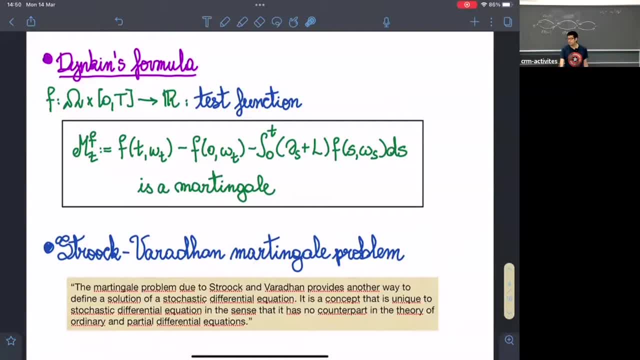 inside this integral. This is just a. it's just a formula that gives you a bunch of martingales out of a Markov chain. okay, It's called the Dinkins formula. Sometimes Dinkins formula is called something else. 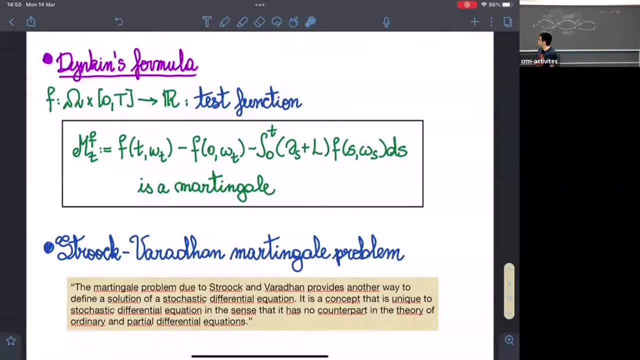 but it's equivalent to this one. And here, and this is an important thing, this is a sort of change of paradigm By the so-called Strouk-Varadans-Martingale problem. So, Strouk-Varadans-Martingale problem. 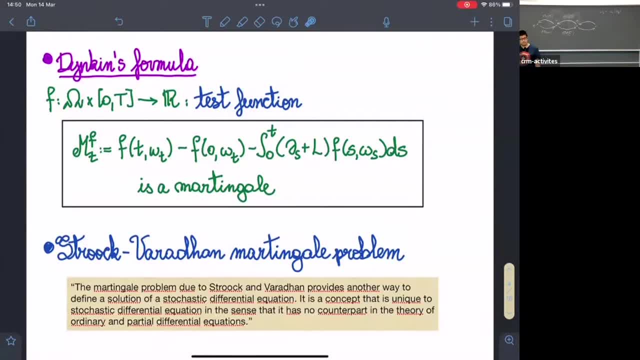 tells you the following: that a Markov chain, or what A process omega t is a Markov chain if, and only if, all these guys are martingales. okay, There's maybe a typo. the second omega should be an omega zero, I guess. 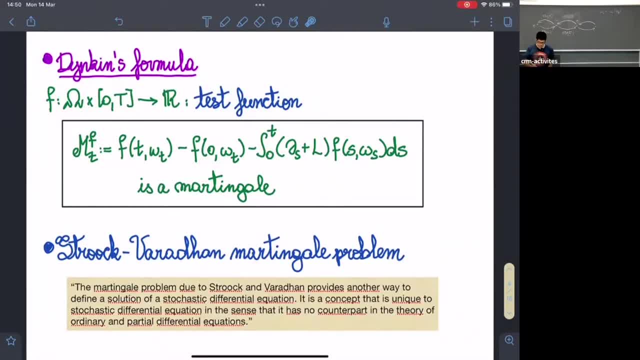 Yeah, Yeah, probably, yes, thank you. Okay, let's correct that. Yeah, that's right, thank you. So the Martingale problem of Strouk-Varadans is a different way to look at a Markov chain. okay, 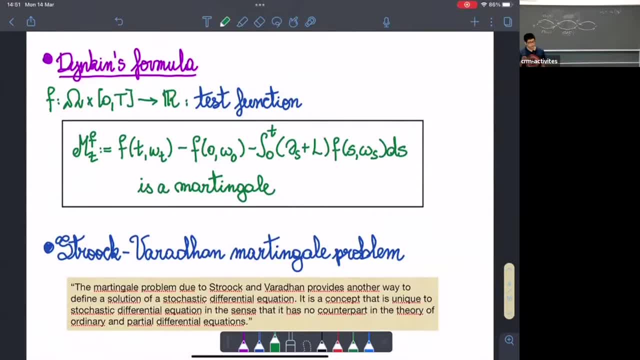 So I'm going to repeat it again because it's an important thing. So a process: omega t is a Markov chain if, and only if, these guys are martingales, okay. So it's a different characterization of a Markov chain, which means that all information 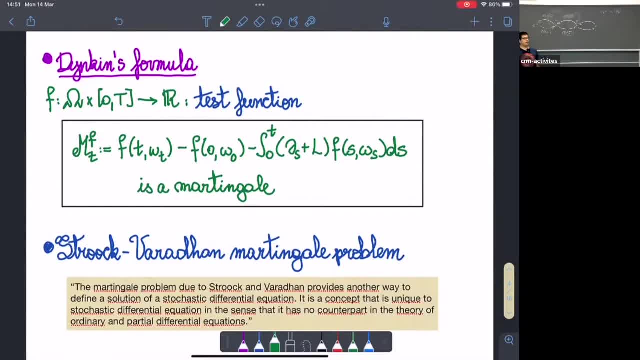 that you can take out of a Markov chain using the usual methodology. that is is taught, for example, in a basic course on Markov chains. you can also do it with Martingale theory. Okay, So okay. so here I took a random quotation from Google. 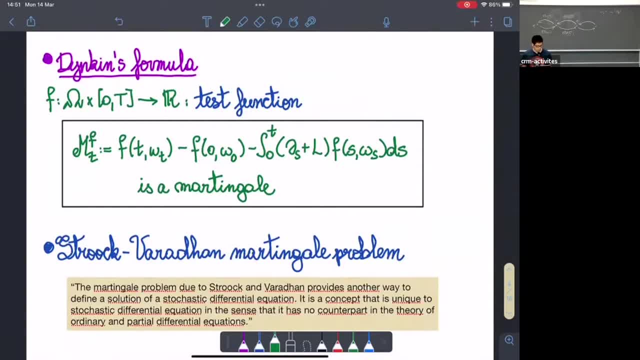 so I just put on Google Martingale problem and took the first nice quotation I found which says: so the Martingale problem, due to Strouk and Valadon, provides another way to define a solution of a stochastic differential equation. 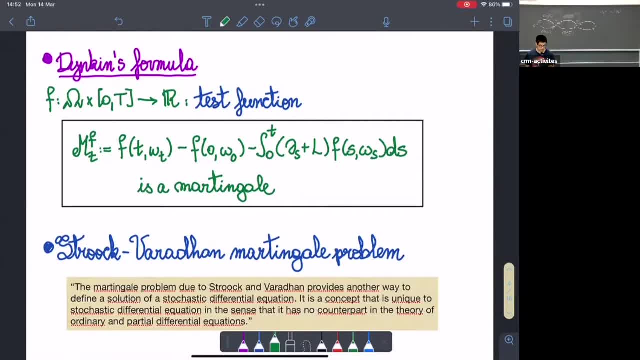 It is a concept that is unique to stochastic differential equation in the sense that it has no counterpart in the theory of ordinary and partial differential equations. Okay, So well, here you should change a stochastic differential equation by Markov chain, and it's the same thing. 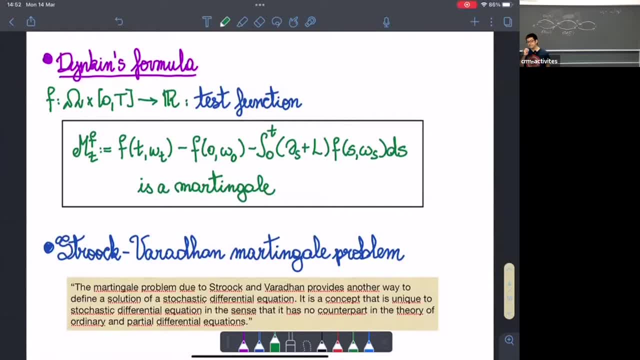 So that's interesting about Martingales is that Martingales don't have a somehow a counterpart in in differential equations. Therefore are they have a probabilistic flavor that made them amenable to probabilistic computations, although they are an analytical tool. 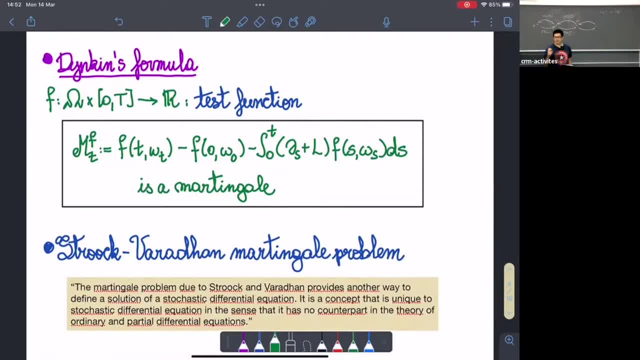 Okay, So this is. that's the whole thing. So when you use these Martingale problems, you open the door to combine analysis and probability in an effective way. Maybe you don't know this, but you know this. Maybe you don't want to do that. 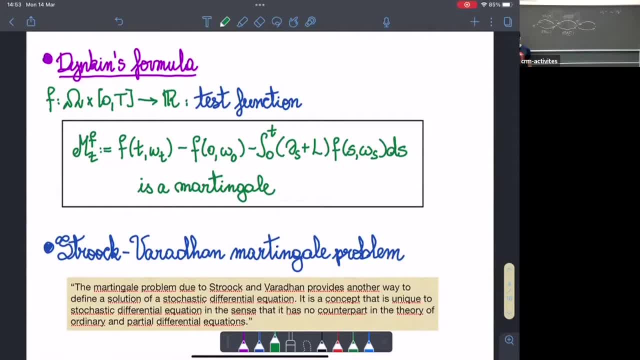 because you are. you're very bad at analysis and really good at probability, and that's perfectly okay. But maybe you are half and a half. You are kind of good in probability and kind of good in analysis, and then you do Martingale problem. 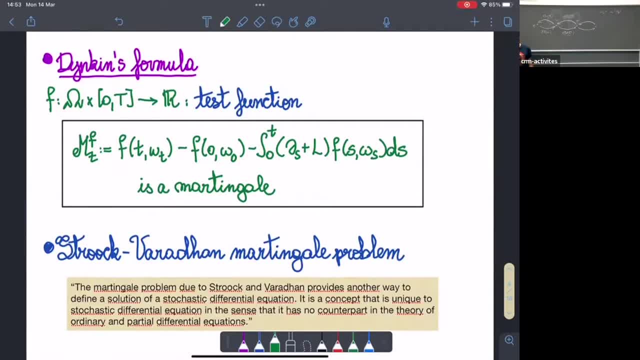 and, and, and, and, and, and. it looks like you are much smarter than you really are. So, Milton, sorry, there is a question in the chat. Okay, Concerning Dinkins formula, which is the set of test functions. 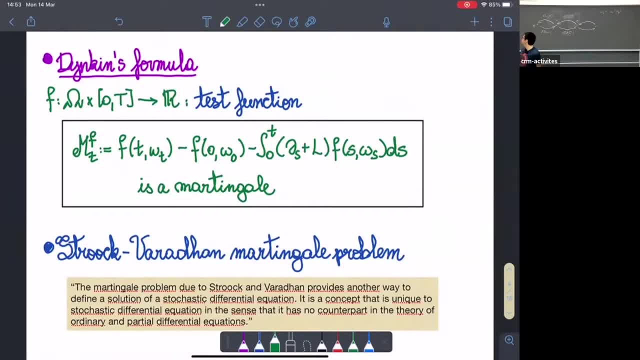 Okay, So any. So it's a discrete. so it's a discrete system. So the only condition you need is differentiability in the time variable. Okay, And for the if and only if condition, if you're interested, you are, you don't really. 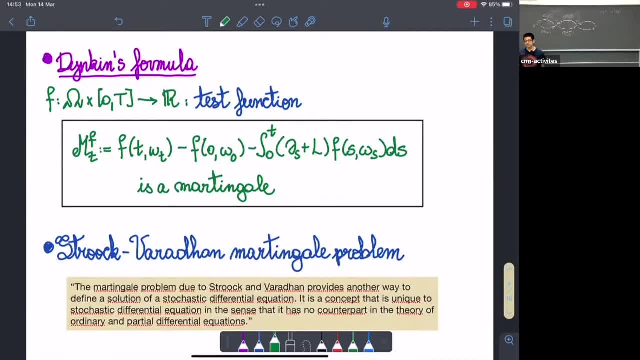 you don't even need the time variable. So you take just functions which are constant in time and you have that these guys are martingales for all these functions. then you characterize your market. So once again, omega is finite. 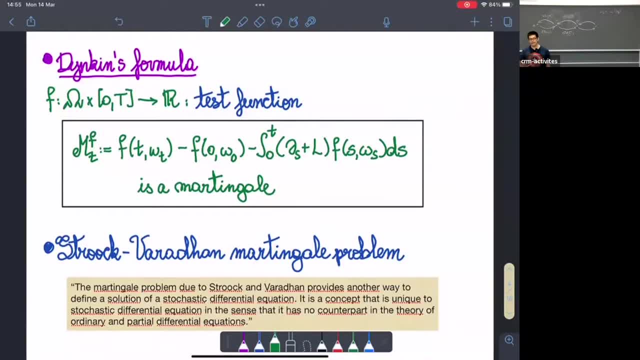 So I can forget about all the technical issues, right, About domains and operator. No. So, in particular, L is a matrix, F is a vector and everything is nice, Okay. So I just wanted to tell you about this change. 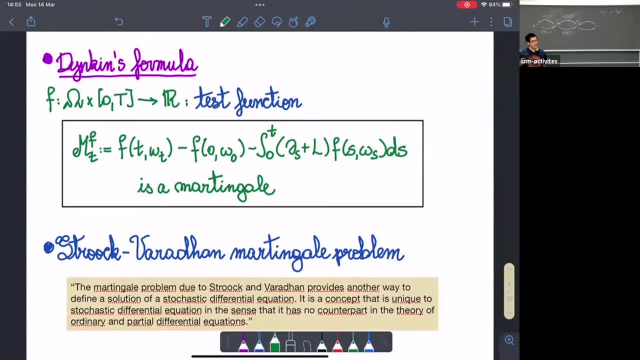 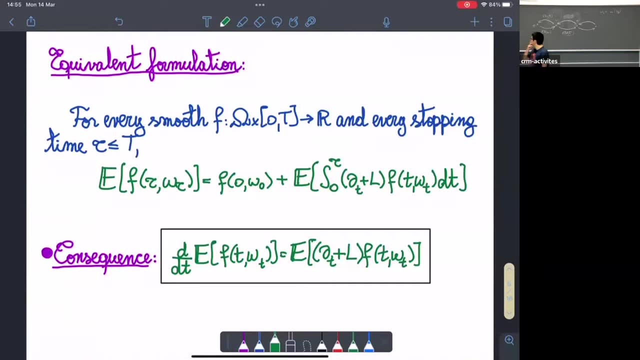 of paradigm, which is the switch from a, from the usual theory of Markov chains, to the theory of Markov chains through the prism of martingales. Okay, So just because in a for people that are more used to stochastic calculus, in stochastic calculus, 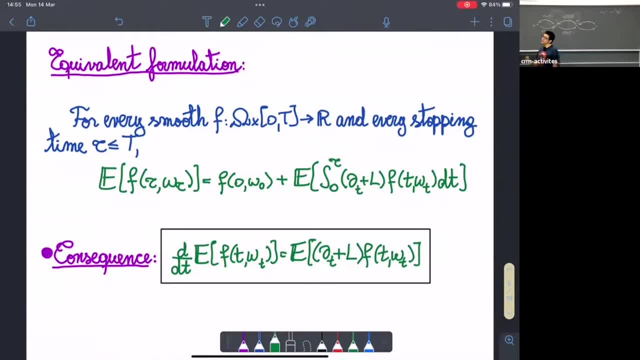 Dinkin's formula is also is actually referred to this formula that is here. That is says that instead of talking about processes, we talk about expectations. So the expectation of F at time tau, it's equal to the initial condition. 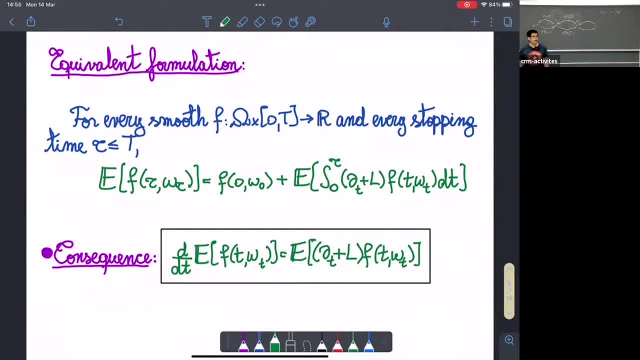 plus the expectation of that integral there And the secret now that tau is stopping time. So if this is true for any stopping time and for any function F, then you say that the your process satisfies the martingale problem. And there is this all equivalence. no, 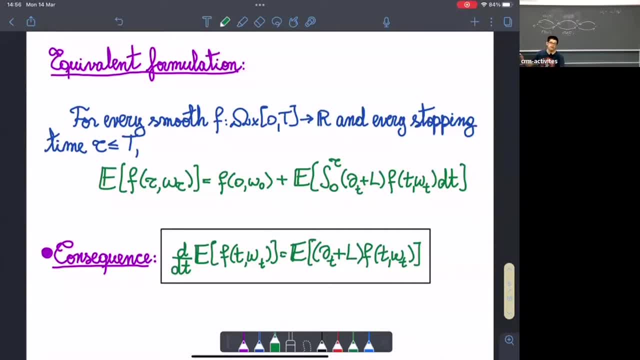 So a martingale is a martingale if, and only if, it satisfies the optional stopping theorem for all the stopping theorems, Okay. So that's why these two things are equivalent And there is a consequence okay, which is sometimes very useful because it allows you. 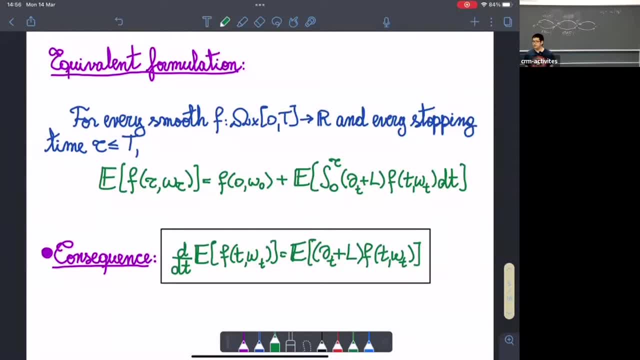 to compute some non-trivial expectations of functions of your process that the derivative of the expectation of a function of your Markov chain. this is what I usually call an observable. Now that goes on From physics to call it an observable right. 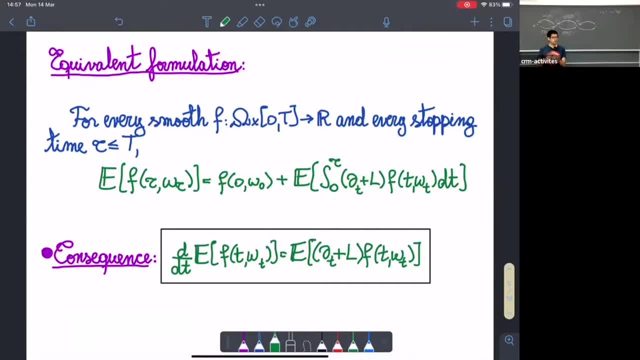 The expectation. if you differentiate the expectation of the observable for Markov chain, what you obtain is the expectation of a function which is just the generator applied to the observable. Okay, So if there is a time dependence, you have to add a time derivative in your formula. 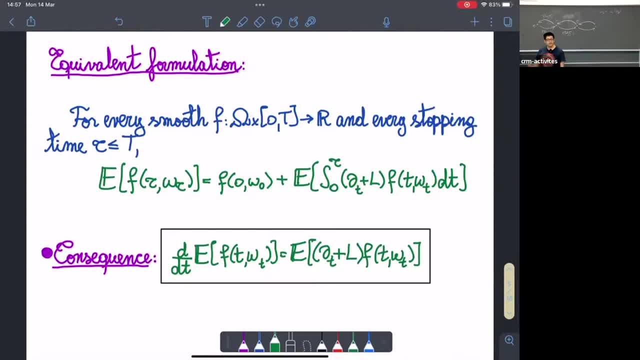 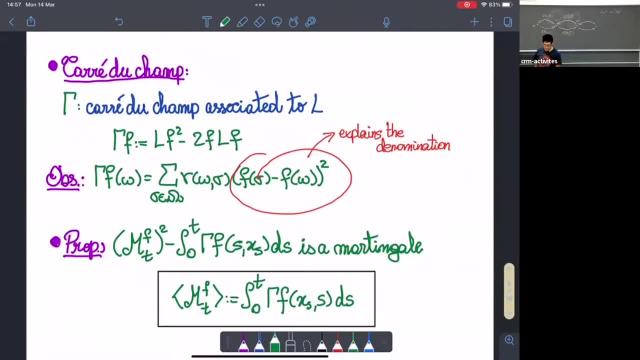 but that's, that's what it is, And- and this formula is very useful- many content, So now okay, So now let me define something which is at first sight very mysterious- And then, when you get used to it, you still find it very mysterious- which is called the 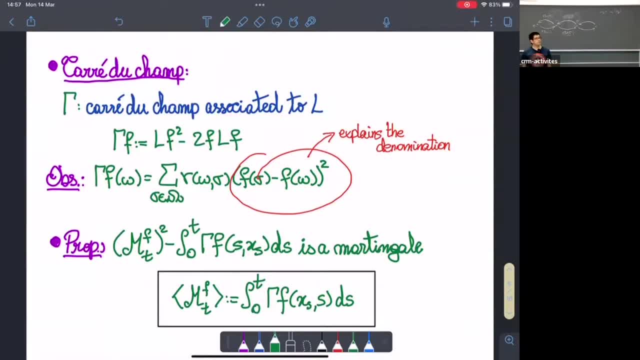 Carre-Duchamp. Okay, So what is Carre-Duchamp associated to L? So there is actually a family of operators. Okay, So these guys appeared in algebra actually. So you have a linear operator and then out of this linear operator you do some bracket construction that I don't really. 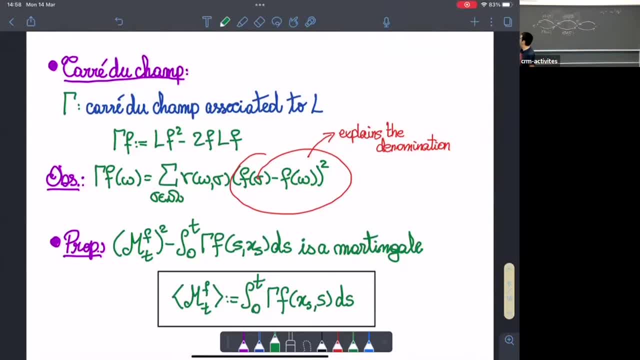 understand very well. And then suddenly you get this Carre-Duchamp operator, which is a bilinear operator. So here is a quadratic operator. Okay, So instead of linear it's quadratic in F. So by polarization you can also define a bilinear operator like a gamma of F, comma G. 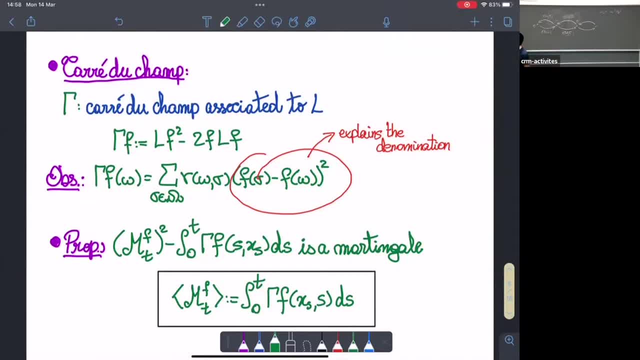 And you may imagine that there are also- this is going to be something like gamma two- there is a gamma three, four, five, et cetera, which are multilinear operators that make sense as well, And in our context, we're going to be contented with describing the Carre-Duchamp, because it's the 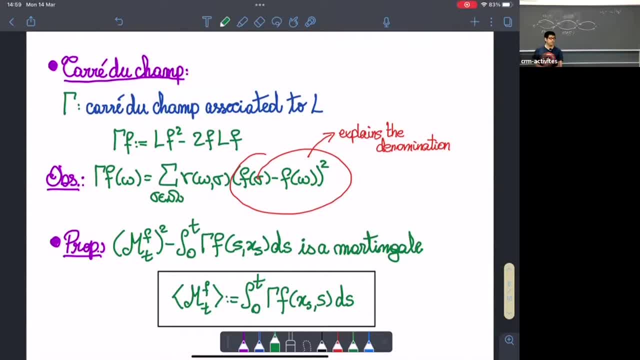 linear operator. So there is a formula. So there is an explicit formula in terms of the rates, of the probabilities of our Markov chain, which is given by that. So from here you see why it's called somehow the Carre-Duchamp. Okay, So that means it's like the square of the 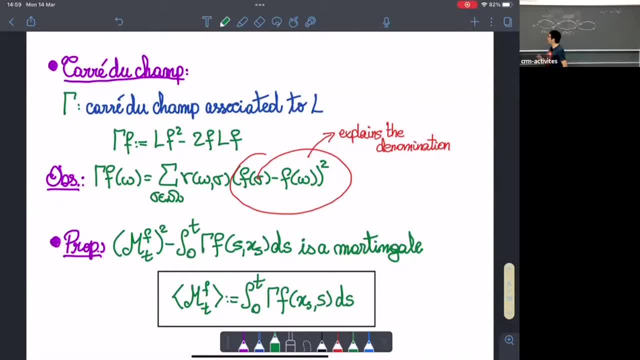 derivative. That's what you have to think about. Okay, And so the generator is somehow it's like the derivative of your function F along the trajectory of your Markov chain. This is kind of what the, the operator, is, And this guy here is the square of that derivative. Okay, So you take the square. 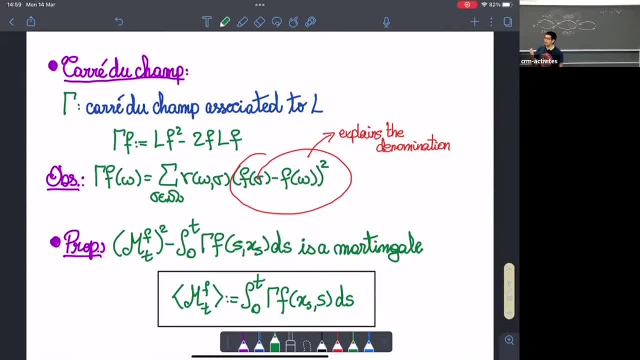 of the increment you do and you multiply by the probability of seeing actually seeing that increment, and you then you sum over all possible guys, And, and that, that that gives you this operator, Carre-Duchamp, and, and, and it's a and it's a function right. 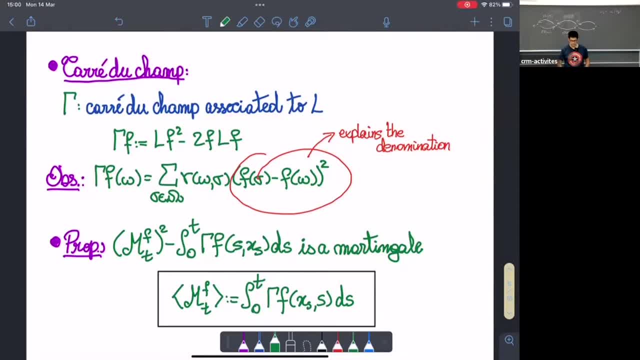 Now the comment: it should be the symmetric part of R, naught R in gamma, isn't it? So So, So, So That's actually another thing, is that's the Dirichlet form. So the Dirichlet form is the integral of this guy with respect to the invariant measure. 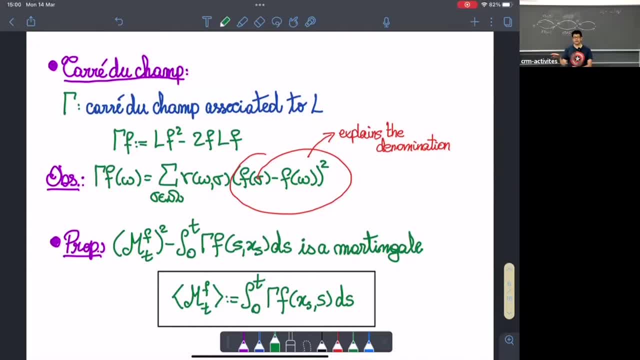 And when you do that you lose the, the, the anti-symmetric part of of the guy, but at, but here it's better to keep it okay for the, for what it's a, for the computationals, and I'm going to. 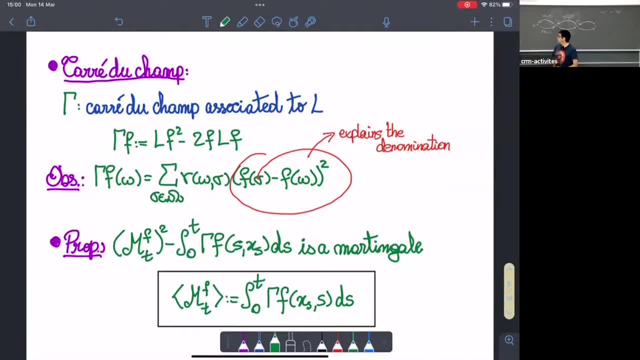 Okay, So that's the. that's the thing, Um, And in our context, it's important not to take symmetric part of anything, because we always will have in mind that we want to try to treat non-equilibrium situations okay. 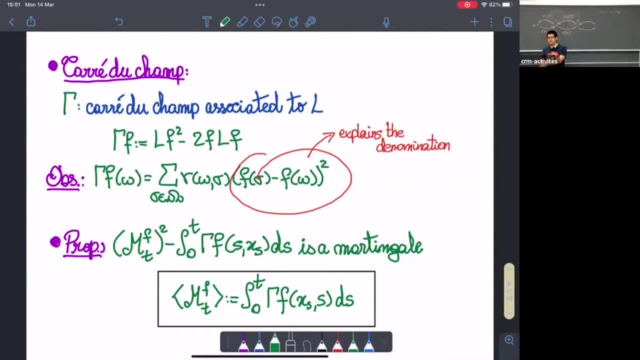 Non-equilibrium stationary states, non-equilibrium systems, which means that we don't really know the invariant measure. maybe Maybe we know the invariant measure, but it's too complicated. We don't want to use that information. So we want to really try to develop a sort of methodology that avoids to look at those guys, because that's too much information for us, for them. 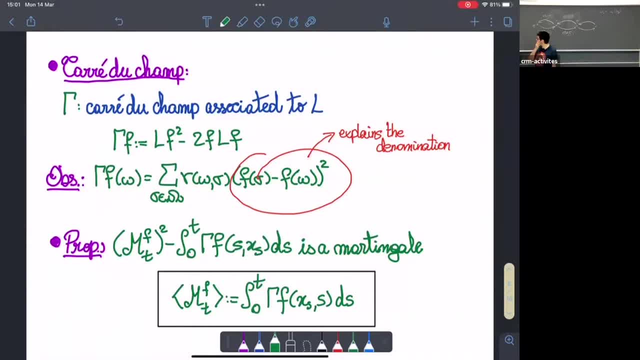 Okay, so this is a proposition, This is something that one can try to prove. is that that guy? there is a martingale. So we start with a martingale MF of T, which is usually called the Dynkin martingale because of the Dynkin formula. 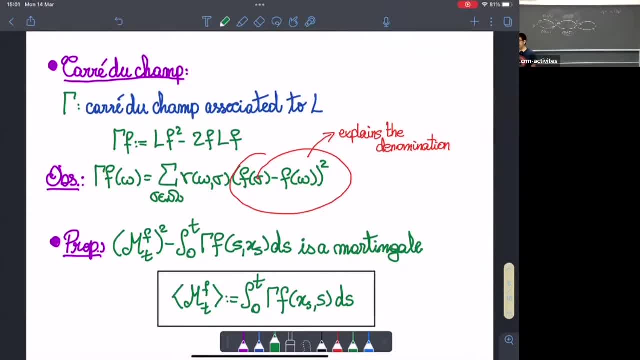 And well, you square it and then you get a sub-martingale. And now that you have a sub-martingale, you have to take out something to make it into a martingale again, And this something that you take out is exactly that guy there. 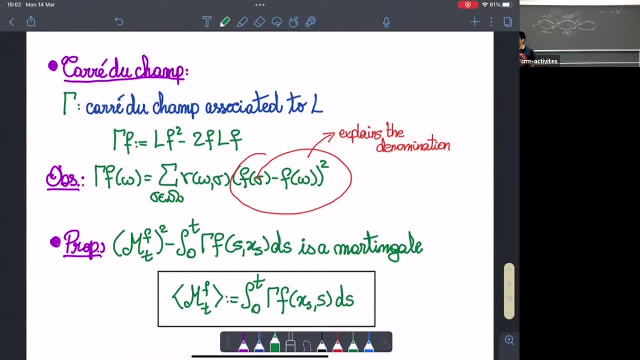 And that's what people call the predictable quadratic variation of a martingale. okay, So already. so, Hendrik already gave you a definition of the predictable quadratic variation. And in a comparison, there is another quadratic variation, Which is the usual one that the one treats, for example, in Ito's formula, which is the limit of squares and stuff like that. 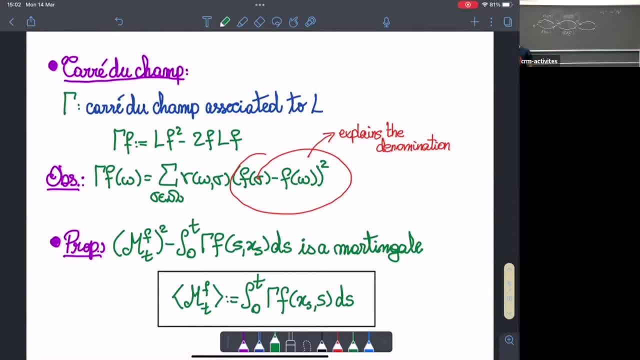 So this is not what we're going to do here, because this is not what actually works. well, What works is to do this predictable thing okay. So for us, the definition is that This predictable quadratic variation is what you need to take out of the square of the martingale to make it into a martingale again. 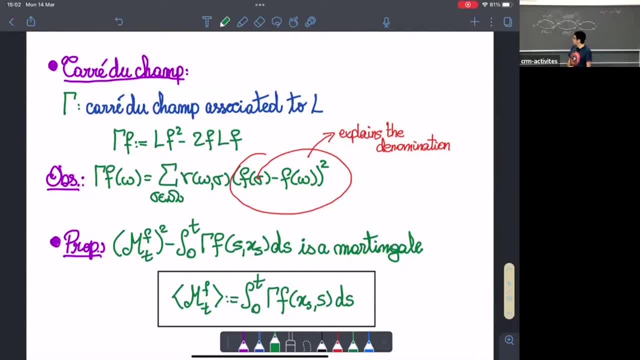 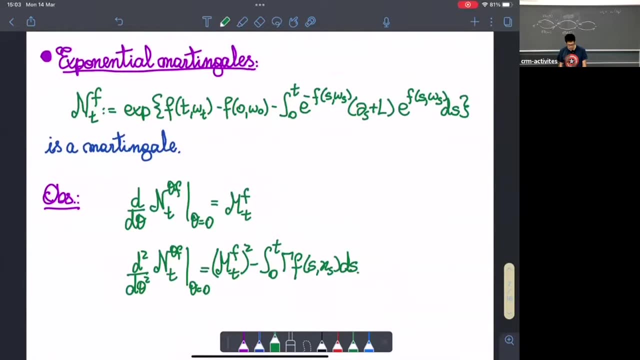 I've been always puzzled about these formulas, So I always try to find a way to understand where these formulas come from. and well, this is the one. I don't know if this is a really good one, but this is. I like it okay. 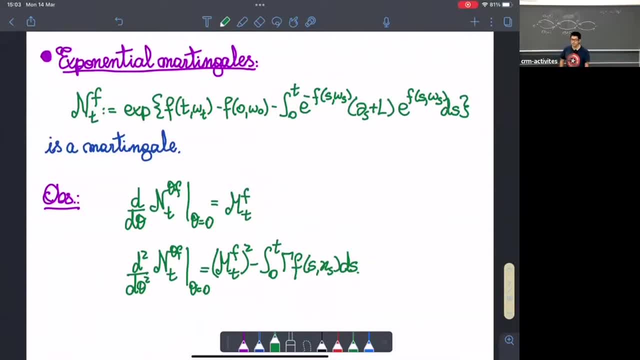 So it makes me a little bit more comfortable with these formulas. so it's about exponential martingales. okay, So it turns out that If you have a fraction, Okay, If you have an observable of your Markov chain, that guy, there is a martingale, okay. 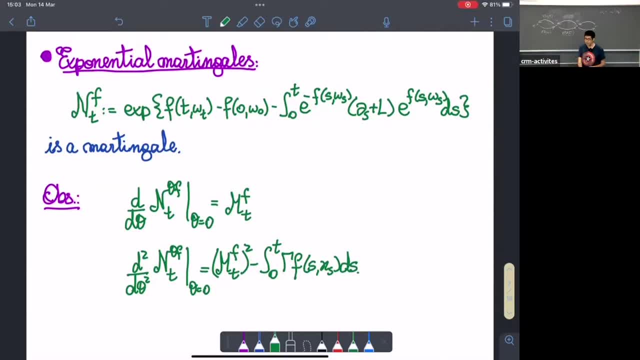 And you may or may have not seen that before, so let me let me quickly write something here on the blackboard. So if you have a, let me take a Poisson process, okay, So this is just a Poisson process. 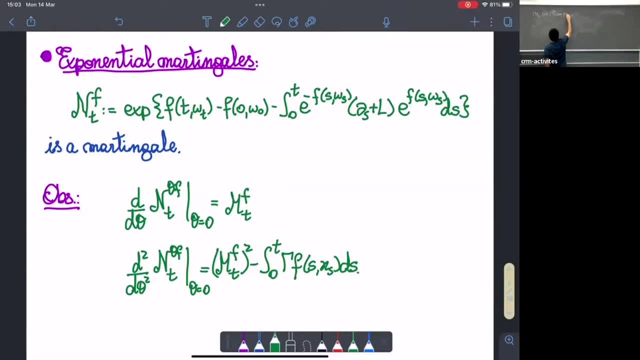 The usual Poisson process with rate one, nothing fancy, And then one can construct explanations. So you can take e to the theta n and you have to discover what you have to take out of this guy to make it into a martingale. 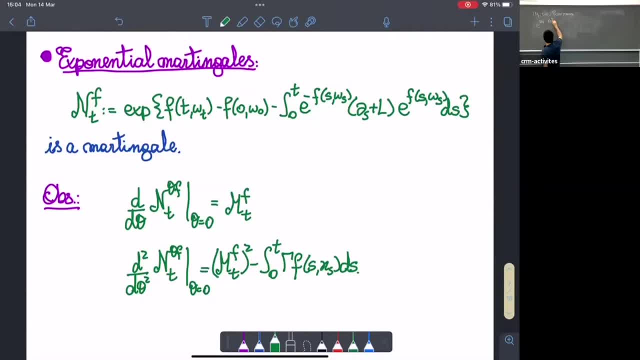 And what you have to take out. you can check that it's e to the theta minus one t. So this guy is. So maybe you are more ambitious and now you want to do something like this. So you want to do, instead of theta, you may want to do theta of t n of t, okay. 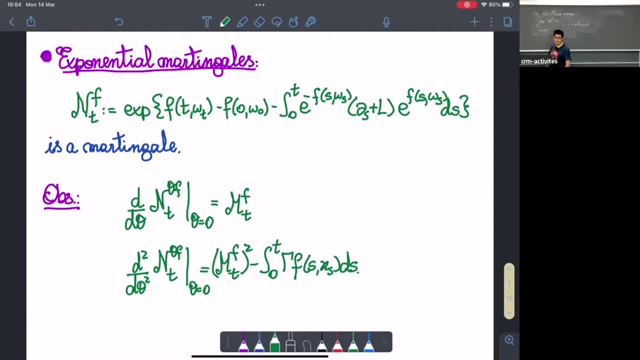 Okay, Okay, And now what you have to take out? Well, what you have to take out is actually: well, it's there, no Markov process. the usual Poisson process is an example of a Markov chain, so you can apply that formula there. 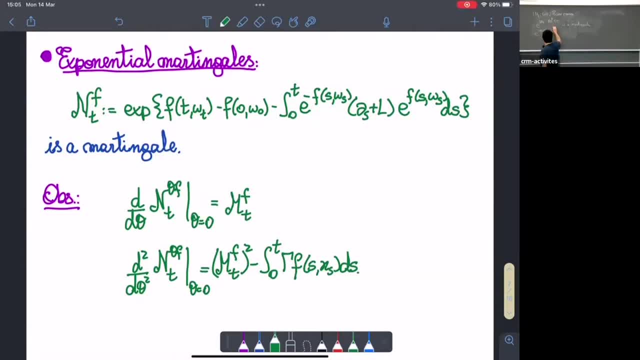 So what you have to take out is the integral between zero and t of e to the minus theta, s and s times. So this is the time, The time derivative plus the generator. So this guy is a martingale, and then you can use it in computations and you will find the formula. 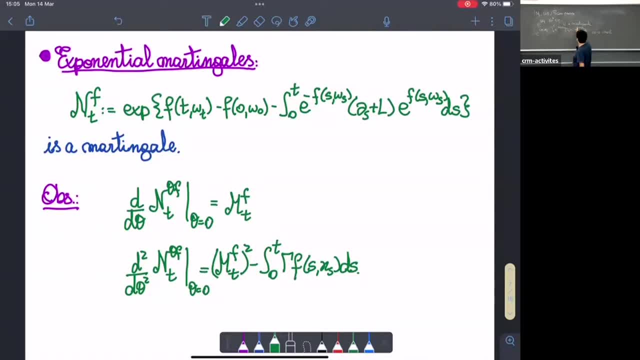 Let me see What is the formula. So you divide, then you take the derivative, So it's probably something like. I don't know You have to do the computation, But the point is that from a Poisson process you can compute this martingale. 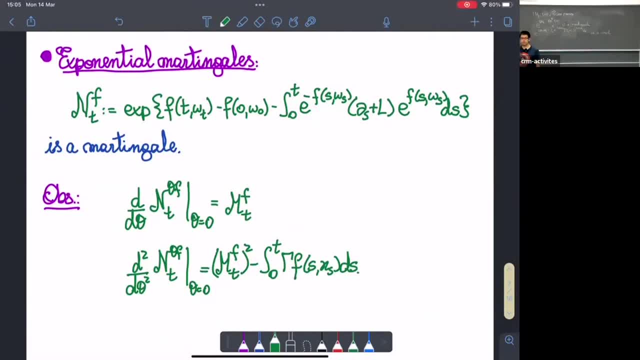 and now you can understand a Markov chain as a bunch of Poisson processes go around in закrinier. That's where the martingale erf Keeps yep parallel because of this construction about the clocks I mentioned before. So there is one Poisson. 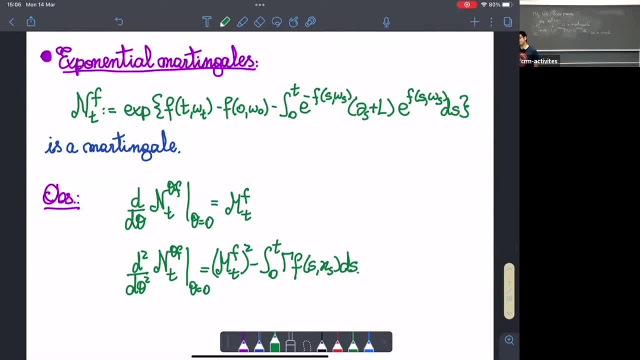 process at each one of the arrows of the adjacency graph of the Markov chain, And each one of these Poisson processes gives rise to one of these martingales where this theta of t here is actually what: It's zero if the Markov chain is not at the right position and it's one if the 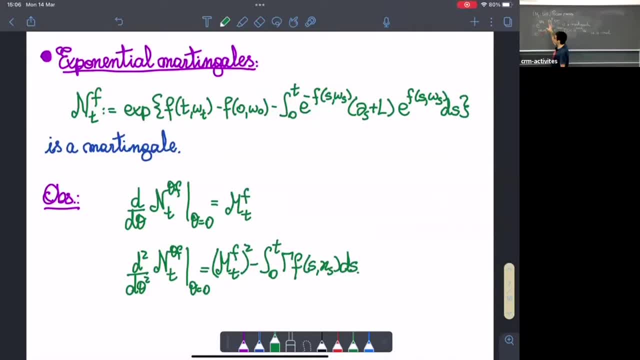 Markov chain is at the right position. You can combine all of those guys and get that exponential martingale there. So this is just a formula that you can try to prove. Because of the comparison with the Poisson process, I found this formula more believable than the other. 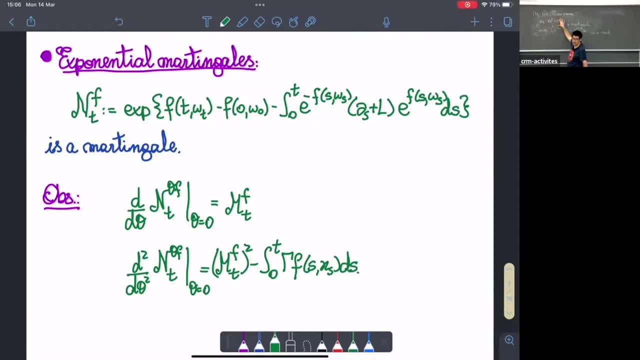 ones I gave you, especially the Carre-Duchamp formula. And then what happens is that you can recover the martingales I told you before using this exponential martingale. How do you do that? So you put a parameter on the function f, You put a theta and you multiply f by a constant theta. 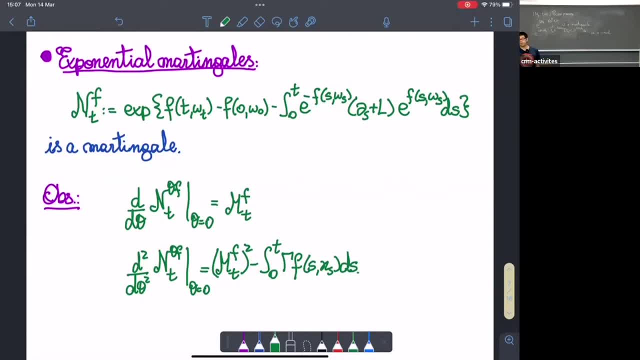 And now you have a family of martingales which are parametrized by theta And you can take the derivative of those martingales And the derivative is also with respect to theta, is also martingale. Just because the state space is finite, you can exchange. 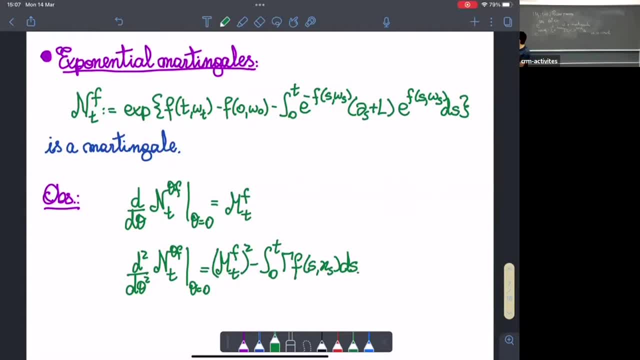 all the exponentials and derivatives that you want. And then when you take the derivative, the first derivative, if you evaluate it at theta equals zero, gives you m of t, the Binkin martingale. And the second derivative gives you the one that gives the Carre-Duchamp. 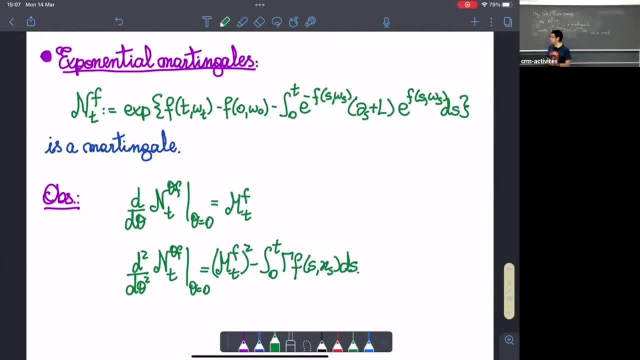 So this is a way in which you can understand this. Carre-Duchamp, It's just the second term in a series expansion of martingales. So if you're interested and you have patience, you can take the third derivative and get another martingale with compensators. 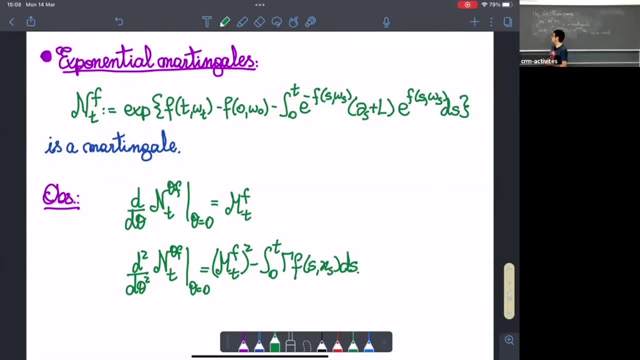 And you are going to discover a gamma three out of it. And you take the fourth derivative, you want to discover gamma four, and so on and so forth. So this is one possible way to see that this: Carre-Duchamp is just the L and gamma are just the first and second terms. 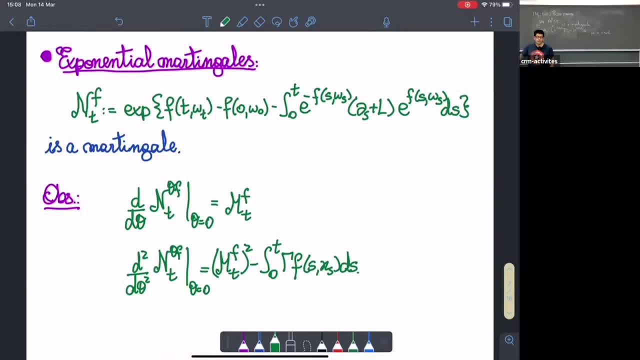 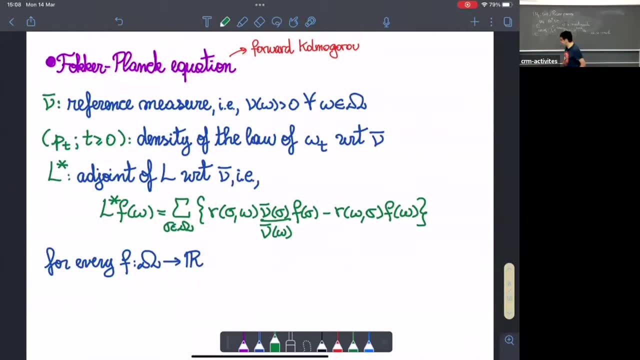 in a series of operators. that appears when you look at martingales of Markov chains. Okay, so now Fokker-Planck equation. So what is Fokker-Planck equation? Remember, or you learned from a basic course on Markov chains that there is something called the. 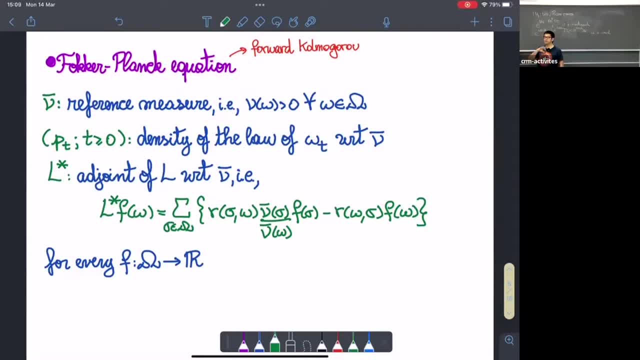 transition probability group. So there is this P T of x and y, which is the main object that you use to construct Markov chains, And that object satisfies some equations, okay, So what people call the forwardcol molecule of equation and the backwardcolon molecule of equation, And so 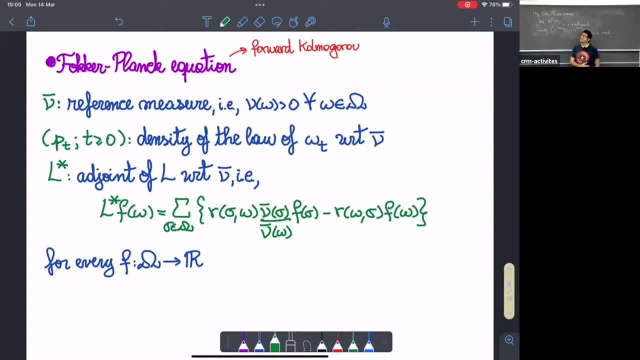 the? No, I don't remember. So the fiction in the karşending matrix: Um is Um, so… И сейчас тут есть еще三個. forward Kolmogorov equation is what we call the Fokker-Planck equation. right, And somehow the 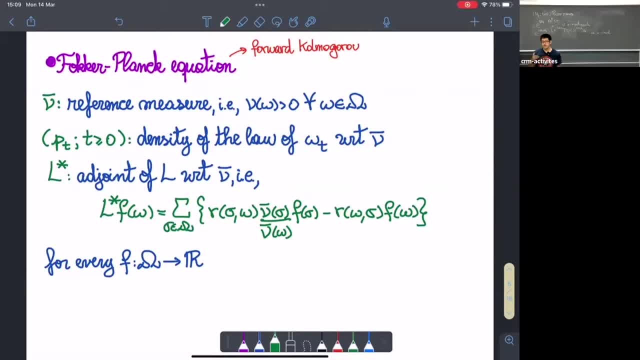 forward. Kolmogorov equation is the most difficult one because it does not involve the generator of your Markov chain or your transition probability matrix. in the discrete case, It involves the joint of that and that can be complicated. So let's try to understand that, okay. So 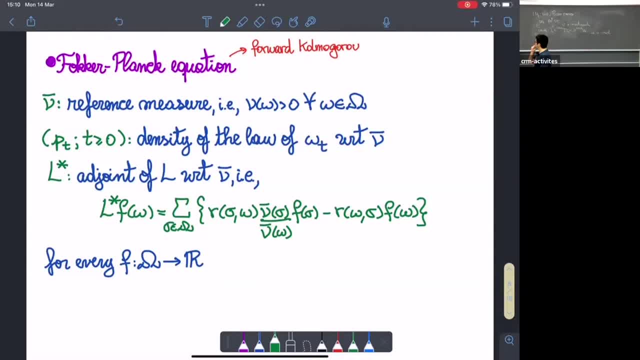 what is the Fokker-Planck equation? Okay, so the first thing that you need to fix is a reference measure. okay, So you have your space and usually, depending on the geometric properties of your space, there is a natural reference measure that you want to take as a base for your. 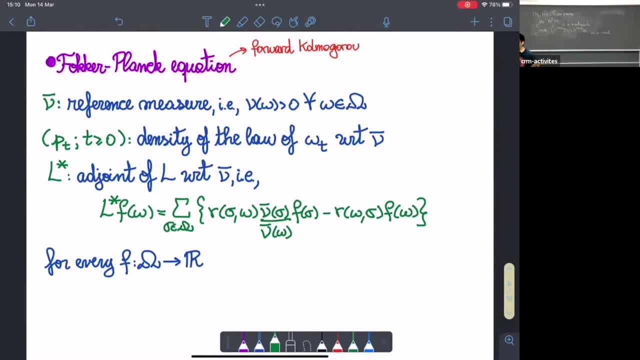 computations, For example in the real line. when you look at the diffusions on the real line, the natural reference measure is just the Lebesgue measure. The Lebesgue measure is not always a probability measure, but that does not really create a lot of problems. okay, So if you're not happy, 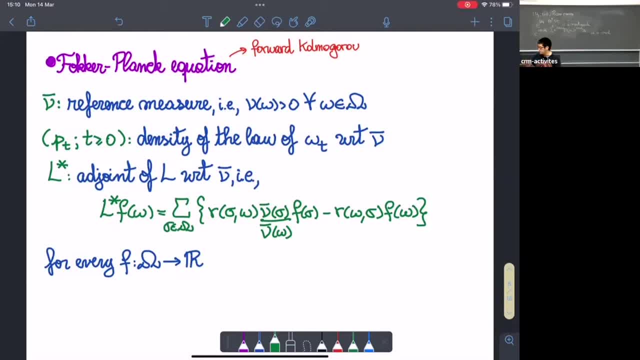 with that. you just take a portion of the Euclidean space, a compact portion of the Euclidean space, then you can define the Lebesgue measure as a probability measure, because you can just divide by the total volume And what people do is that they use that as a reference. 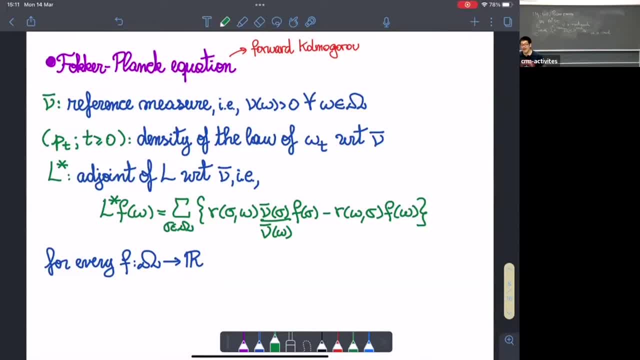 measure because, well, it's the…, it's the one that… it's the nicest one right From…. if you really want to take into account the geometric properties of your space, that is the nicest possible measure. When you are on the Rheumat blueprint chain, there's not always an obvious choice for reference. 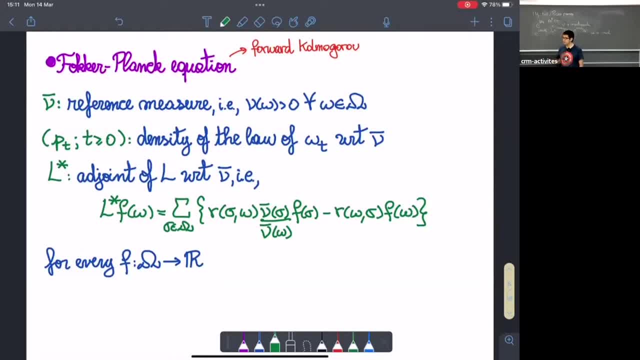 measure right, Because there's not always geometry involved. no, Sometimes there is something else in the blueprint in that location. but for this reason it's gonna be to second. Sometimes there is geometry, you know. for example, you are looking at the random walk on the integer lattice and there the counting measure maybe is a nice reference measure. 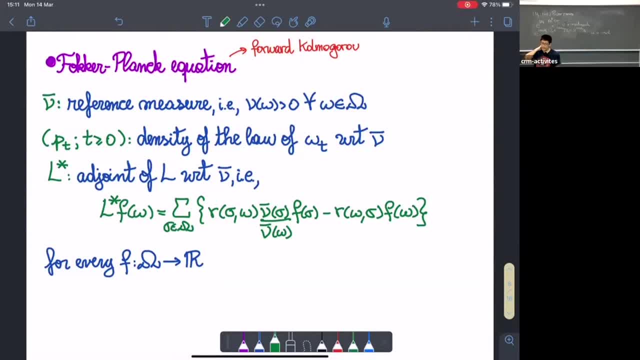 Maybe you are lucky enough that you can normalize it because you're looking at your problem in a finite volume or maybe in periodic boundary conditions. But in general, for general Markov chains there is not a canonical way to do that. So let me just fix one of them. 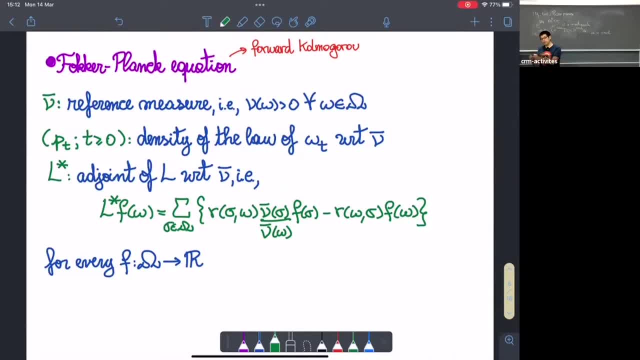 So I'm going to say that a measure in omega is a reference measure if it's positive for all points on the state space. So that's my condition. So there is probably another typo here, Very small typo. Now it's solved. So this is what I'm going to call a reference measure. 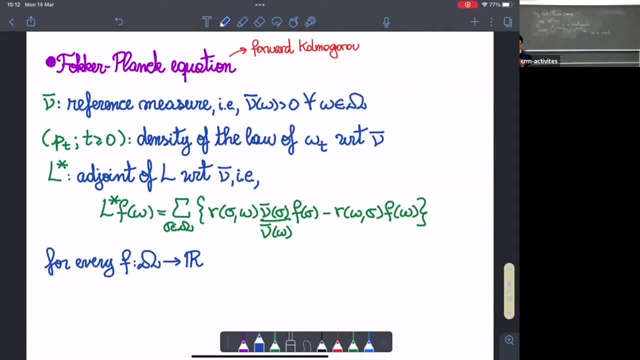 OK. so now remember that I'm calling omega t my Markov chain, So at time t it has some law right, And I'm going to call p of t the density of that law with respect to new bar. That is OK. so what I'm actually doing is just: I'm just defining. 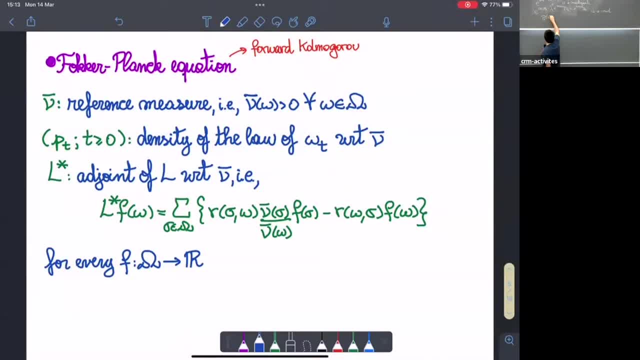 So p t, OK. Omega is just the probability of omega. t equals omega divided by new omega. So here you see, I'm divided by new bar of omega. That's why I'm asking it to be a reference measure. So you may or may not want to put there the initial condition. 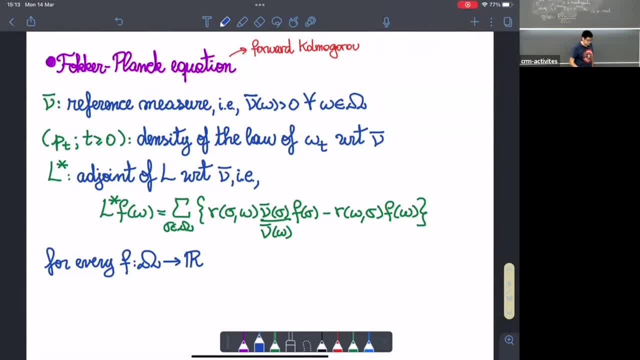 Just to remind you, maybe To add the initial condition into the notation is something that is necessary in some cases, But that's the number. p- t is a sequence of functions depending on t, And the idea is to try to find what is the equation that is satisfied by this p- t. 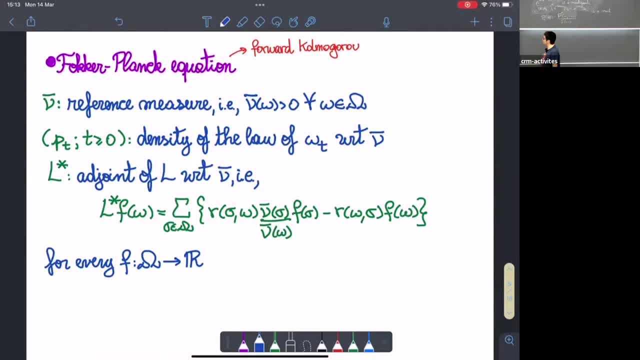 OK, So it turns out that this equation is what is called the Fokker-Planck equation And it involves that joint operator. And what is a joint operator? So this is why the joint operator is complicated, Because the joint operator actually depends on the reference measure you are picking. 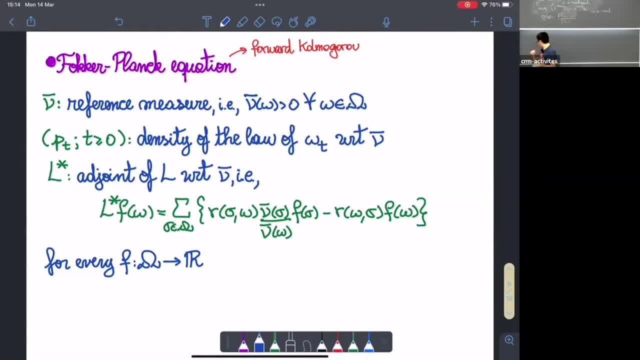 OK, So that joint operator is something that satisfies the following: So it satisfies this relation here. So this is how you define that joint. So it's a little bit annoying because it depends on the reference measure you use, Fortunately enough, since we are working here in finite state spaces, so omega is finite. 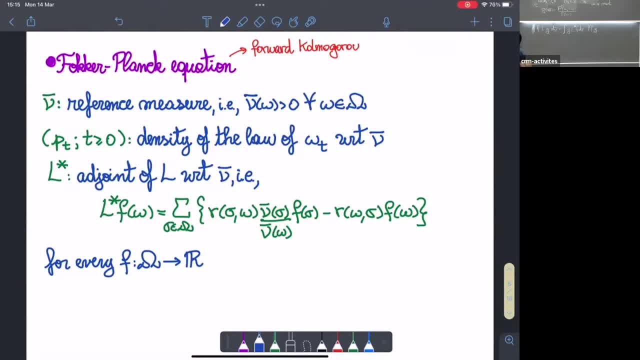 you can actually write this joint in an explicit way. So it's right there. OK, That's the formula, And then You can see that, in particular, from this formula it's not clear that L star is going to be a Markovian generator. 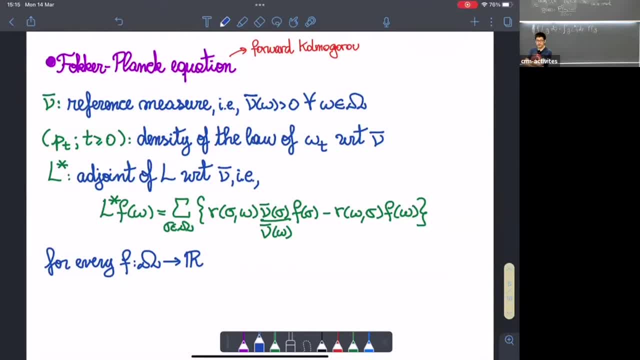 So it's not going to be the generator of a Markov chain, because it's not written in the form of something times the difference of the functions F. You see there's no way to put a difference there in a trivial way, So maybe there are some conditions. 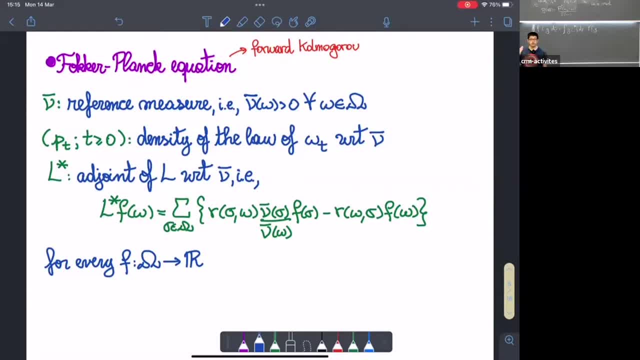 So, for example, if the measure is nu, It's invariant and reversible with respect to the Markov chain, Then this guy here is going to be equal to L just because it satisfies detailed balance. And then you can just combine these two factors to make appear a difference. on the functions F. 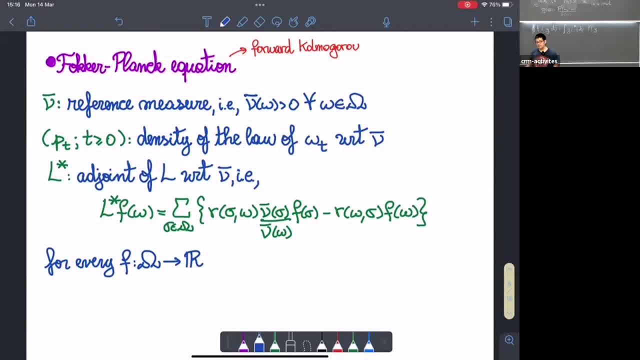 So that's one way to A slightly less trivial way to do that is that if the measure nu bar is only invariant, then L star is going to be a Markovian generator. L star is going to be effectively the generator of a Markovian dynamics. 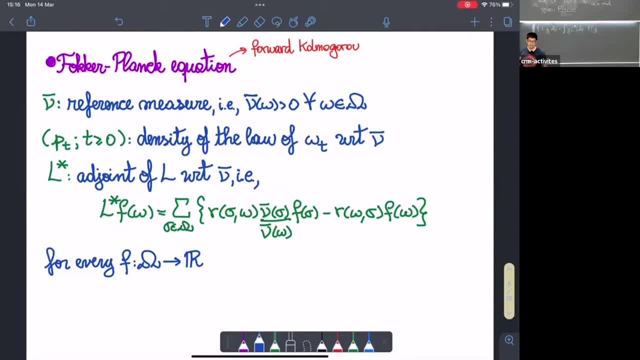 which is actually called the reversed process of the original chain, And there there is an if-only-if condition. So this L star operator is the generator of a Markov chain If, and only if, the reference measure nu bar is an invariant measure. 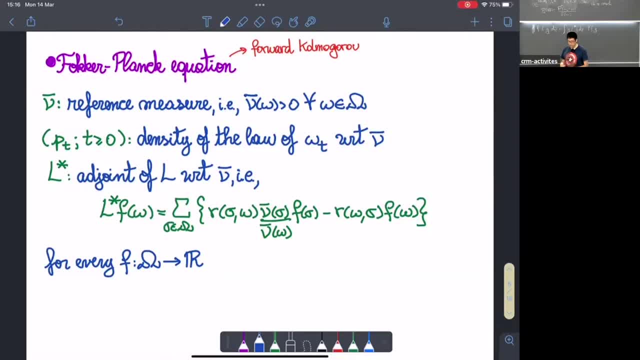 So that's the definition of that joint, And we have Fogel-Planck equation. So Fogel-Planck is the generator. So Frances was asking something that I couldn't catch. So if you could tell me, Alessandra, please, what his? 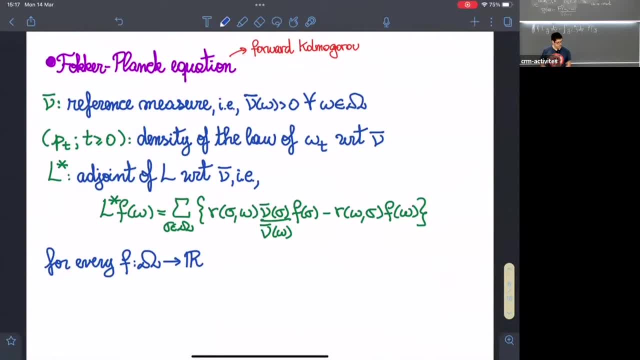 So the question is: is the generator L or L star open on the right in the formula on the blackboard, Open, Open. What does it mean open? Do you mean open, Francesco? Ah, maybe So can you type. If you cannot speak, can you type? 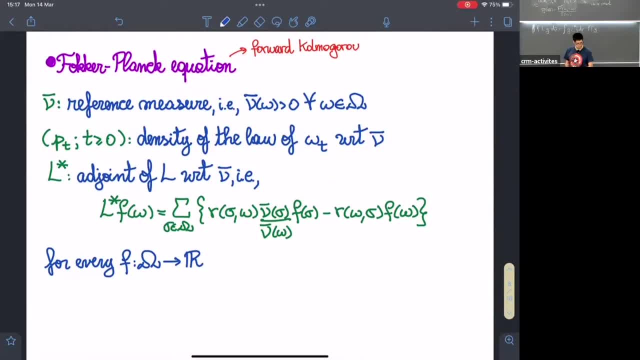 Can you explain, please, the question? Yeah, sorry, Can you hear me? Yes, I can hear you. Yeah, No, sorry, I made a mess in the chat. I think I was chatting directly with Brigitte, Sorry. 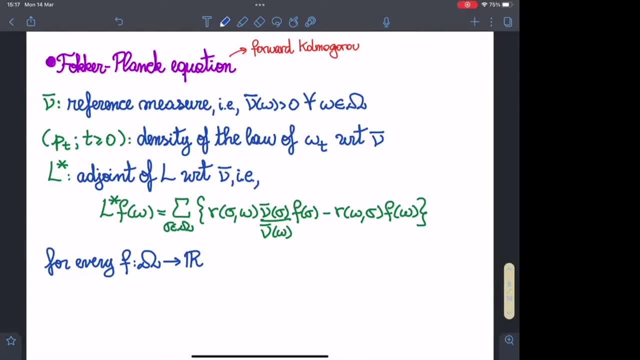 I meant whether it applies on both G and reference measure. Ah, Okay, Yes, I understand. So you mean this. Yeah, Okay, So it means that it only applies on G and F this way, right? Yeah, Okay, So it's perfect. 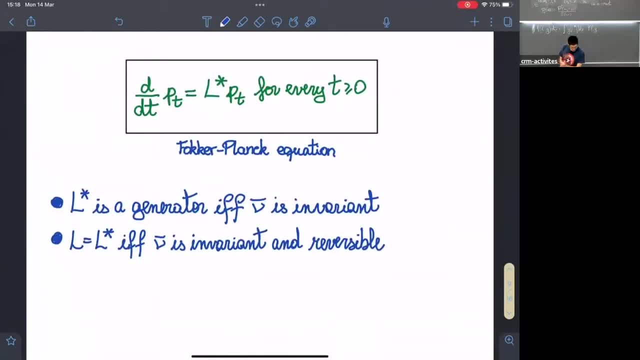 Okay, Thank you, Okay, Thanks Okay. So here I wrote this observation I was telling you before. So L star is a generator if, and only if, nu bar is invariant measure And L is equal to L star if, and only if, nu is invariant and reversible. 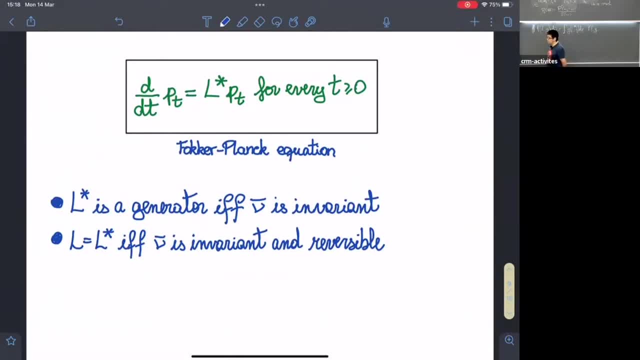 So in the situations we have in mind. So we don't really want to take reversible Markov chains for the moment. I mean, because that's kind of equilibrium Markov chains in some sense, Or maybe you can take anyways, equilibrium Markov chains, but it's not something we want. 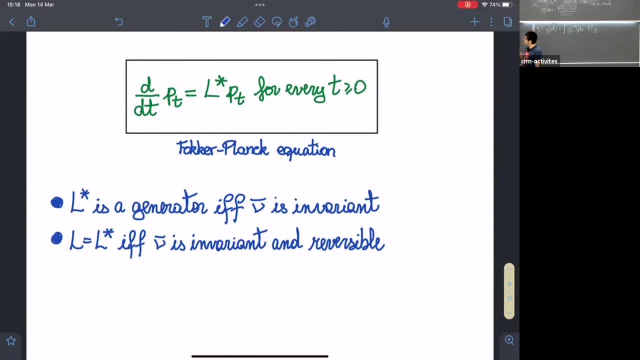 to exploit. Okay, So this is just to tell you that in many situations the operator L star is not going to be a Markov generator And that means that the Fokker-Planck equation is not super nice. Okay, Because if you were a guy from PDE, I will tell you the problem with the Fokker-Planck. 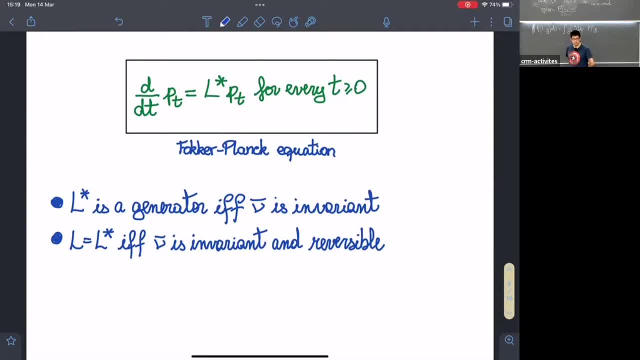 equation is that the L star does not satisfy the maximum principle. So that's the key observation in PDEs. That means that the solution of this equation is not super nice, because without maximum principle, Out of the maximum principle, people in PDEs can get a lot of nice properties for solutions. 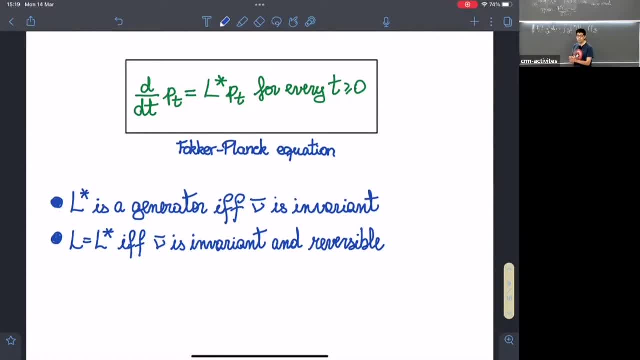 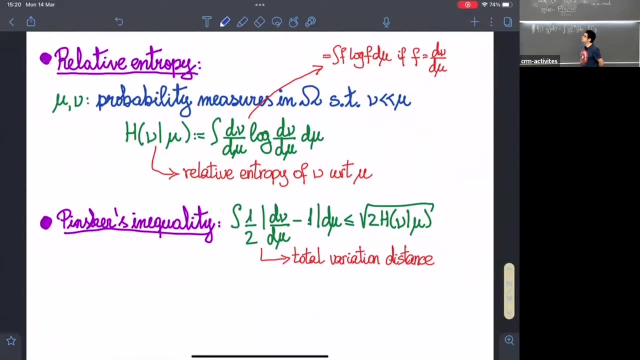 And here you don't have maximum principle. it means that it's complicated, Okay. Anyways, this Fokker-Planck equation allows you to do computations. Okay, So now let me enter into the main thing. So the course is called Anthropy Methods in Markov Chain, so it's pretty much likely that. 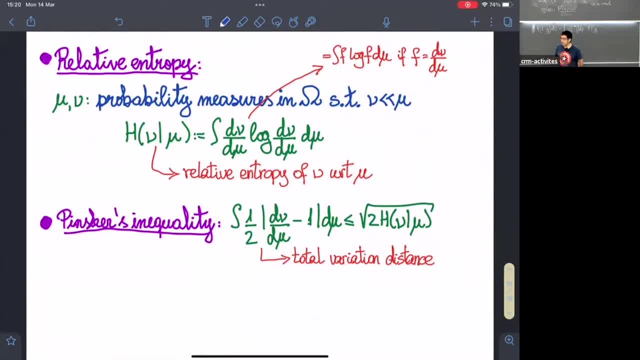 entropy is going to play an important role, And actually the important role here is relative entropy. Okay, So what is relative entropy? So it's a way to measure how different are two probability measures. Okay, So it's just another way to measure the distance between probability measures. 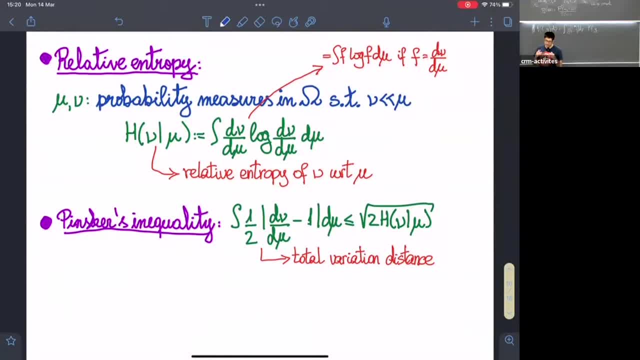 And at first glance, it's very strange to do it in this way, because the relative entropy is not even a distance. Okay, So if you want to measure the distance between two objects, the least you can do is to measure it with the distance. 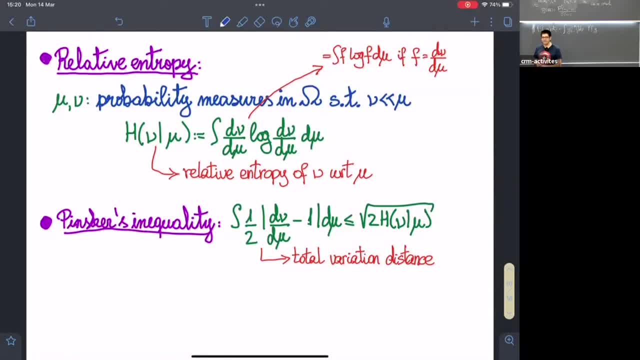 No. And then you say no relative entropy. Well, there must be a reason for that, And the reason is that relative entropy is not a relative entropy. Okay, So relative entropy really works. Okay. So at some point, these guys in the 19th century, Boltzmann and Maxwell, and people and physicists- 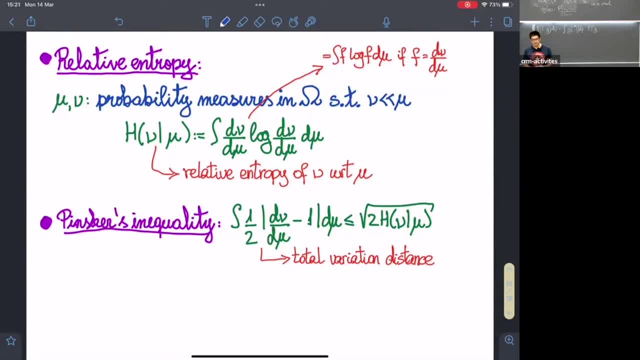 decided that looking at entropy was a good idea, and it was a good idea indeed. Okay, So let's go to the definition. Okay, So how do you find it? It's just the formula there. So it's the integral of F, log F, where F is the density between these two probability. 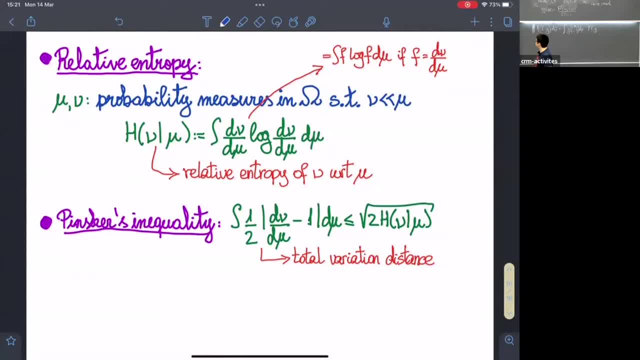 measures. Okay, So here for simplicity, I am assuming that mu is absolutely continuous with respect to mu And in that case this number, the density, is well-defined. and then you can compute this integral, which is finite because our Remember that omega is finite. so everything is well-defined. 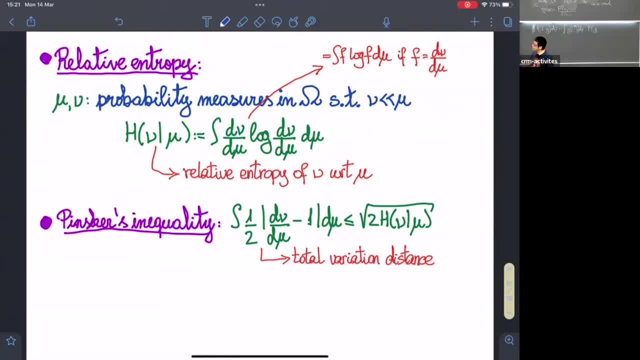 So you usually define the relative entropy equal to plus infinity. if this absolute continuity condition is not satisfied- Because well, it is what makes sense in this theory- makes the relative entropy somehow continuous with respect to the extended topology where infinity is an extra point on the zero. 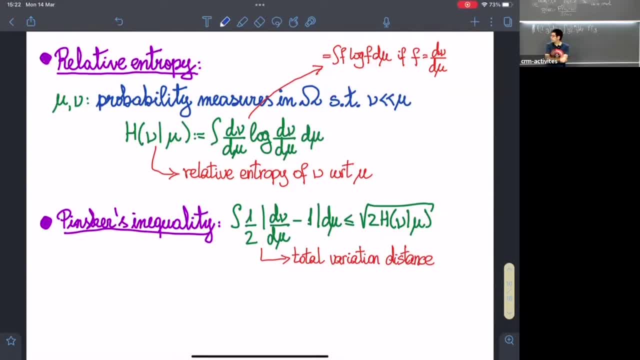 infinity line, And this is what we call the relative entropy between. It's the relative entropy of mu with respect to mu. So it's not between, because it's not commutative. Okay, So It's not between, but it's. 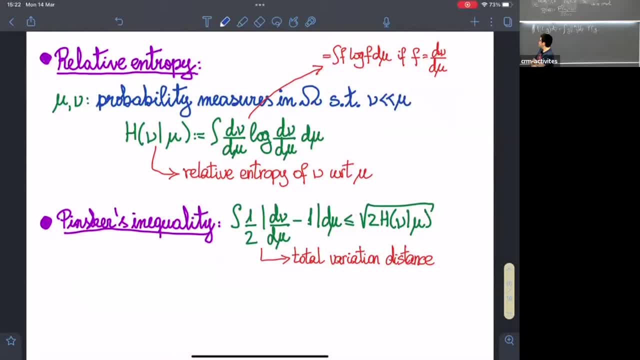 I'm wrong, because it's not something commutative, So it is not a. It's not a distance, It does not satisfy. It's not even symmetric, so it couldn't be a distance. It does not satisfy also, the triangle inequality, so not a distance at all. 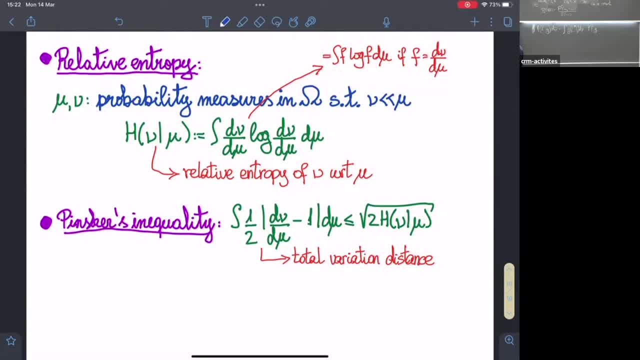 But at least it does satisfy something. no, So it satisfies Ping-scale inequality. Okay, So Ping-scale inequality tells you that you can estimate the total variation distance between two probability measures in terms of the relative entropy. Okay, So this Well, the total variation distance is just one-half of the L1 norm. 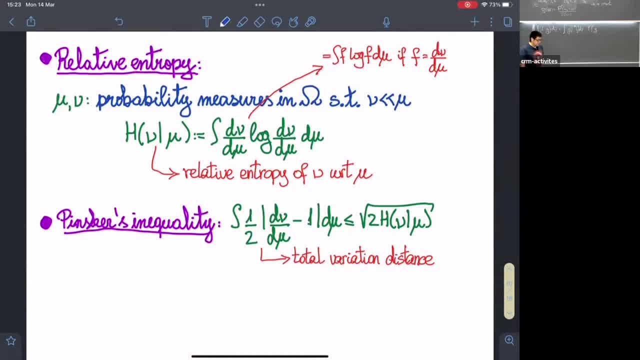 Okay, The L1 distance between these two guys, And of course there are reasons why we define it like that. It's a very meaningful definition from a probabilistic point of view and it has to have the one-half. That makes it even nicer. 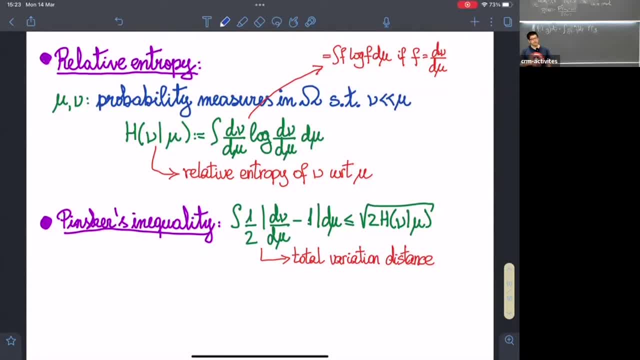 And you have this inequality. So if you are somehow, If you want to know whether two measures are close or not, one possible way to do is to prove that the relative entropy is small. If the relative entropy is small, then the total variation is small, which means that 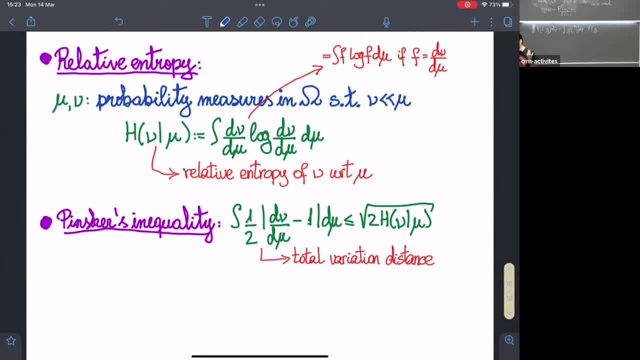 the measures are close in a very meaningful sense. Okay, So the reverse inequality is not true. So it's not true that It's not true that if two measures are close in total variation, then the relative entropy is small. Okay, So you can cook up examples. 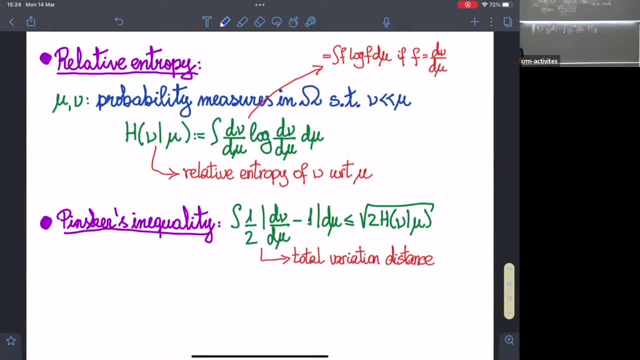 There are some logs involved, but in general it's not true. Okay, So if you know something a little bit more about your measures, then you can get reverse inequalities. But I don't find it particularly illuminating, so I don't think it's worth to discuss the 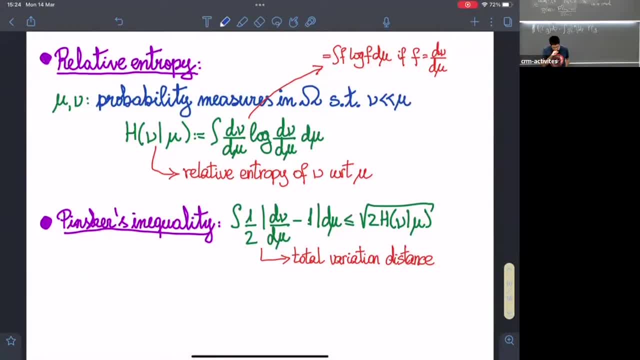 reverse inequality. Okay, So well, something I forgot to say. Okay, of course, this is a mini course. This is for students, So, in principle, students should make questions if they have any. Okay, So I will make a small pause to see whether you have questions about what we are talking. 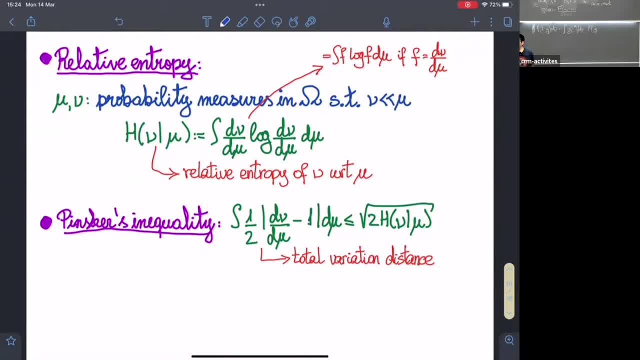 here You want to ask clarifications or something, Something I didn't tell but you may have figured out. On the website I put the slides of the talk of today so you can take a look at them if you are missing something, if you want to catch up with some definition, et cetera. 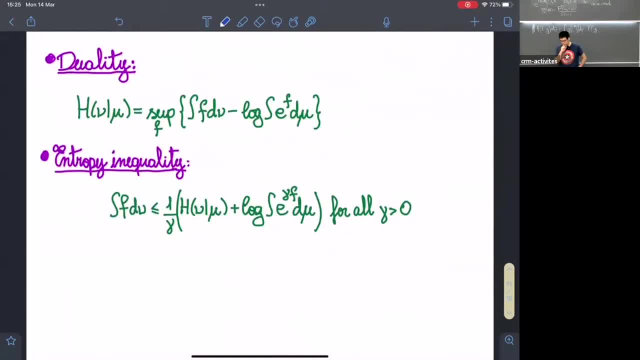 Okay, So another: properties of relative entropy. So relative entropy satisfies a duality definition. Okay, So some variational definition if you want to. So it can be written as a variational formula. Okay, So it's the supremum of the functions f of that quantity there. 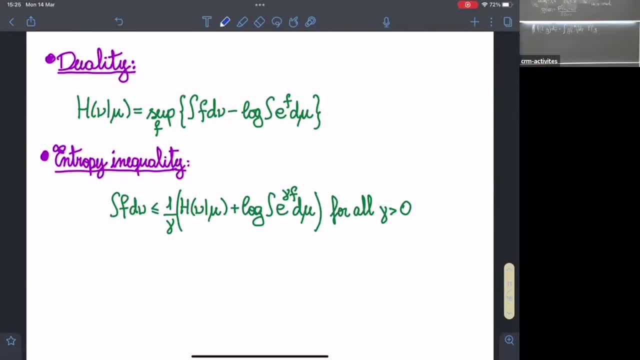 Okay. So if you are familiar with Legendre transforms, you can check more or less easily that this is indeed the case starting from the formula f log f. So f log f has a Legendre transform. Then you can write it as the supremum of something. 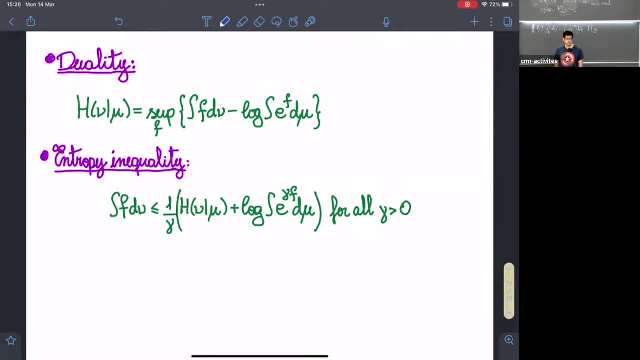 And if you do that, you end up with this formula here. Okay, So it's not a big mystery, But in somehow, in analysis and in, let's say, an analytical approach to probability, it's always good to have variational formulas. 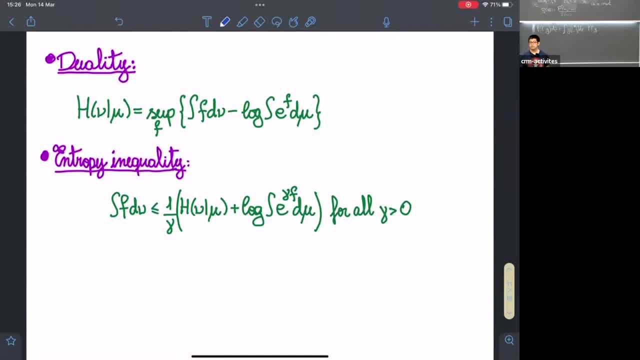 Because they give you meaningful information about different things. So in one hand, they give you one concrete way to estimate things and also gives you a concrete way to take information out of your estimates. Okay, For example here let's say that you know that your entropy is small for some reason. 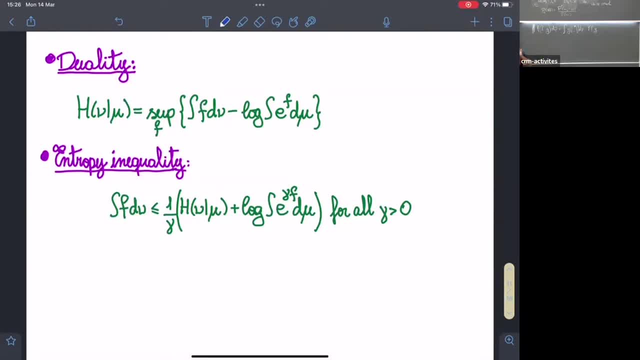 So you know that the relative entropy between mu and mu is small, And you also happen to know the measure mu very well. So the measure mu is something that you don't really know. It could be, for example, the law of your Markov chain at time t. 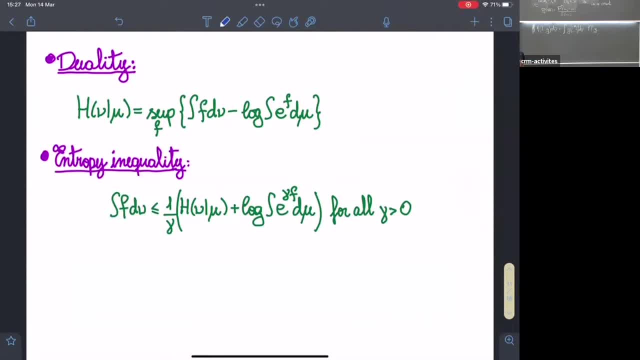 And the measure mu could be the invariant measure, for example. And then you know that these guys are close in relative entropy, And then you want to take information out of that And a variational formula allows you to do that because, of course, h is the supremum. 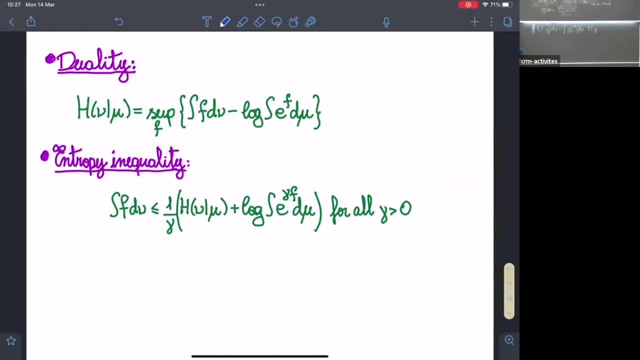 of that quantity there over all functions f. It means that for every function f you have to take information out of that. So for every function f, what is inside the supremum is smaller than the other. Okay, And so that tells you that the integral of fd mu is less or equal than the entropy plus. 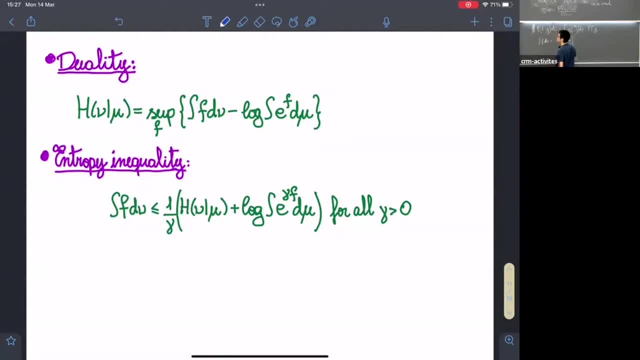 the log of the integral of e to the fd mu. Okay, So that gives rise to the entropy inequality, which is what I wrote down there. To get to that inequality, what you actually do here is that you put a gamma here. no, 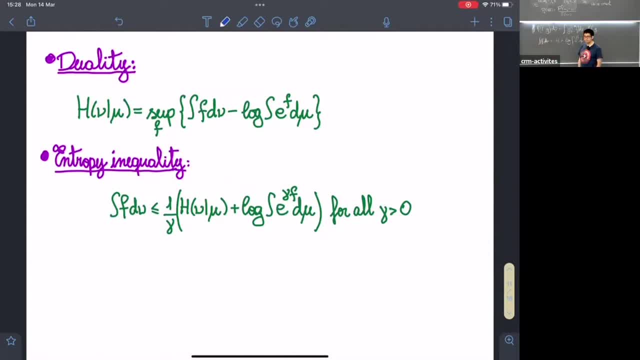 And if you put a gamma here, you get a gamma here. That's it. And it turns out that this form of the entropy inequality is very useful because in many situations you can really tune the gamma in a proper way to get the estimates you want. 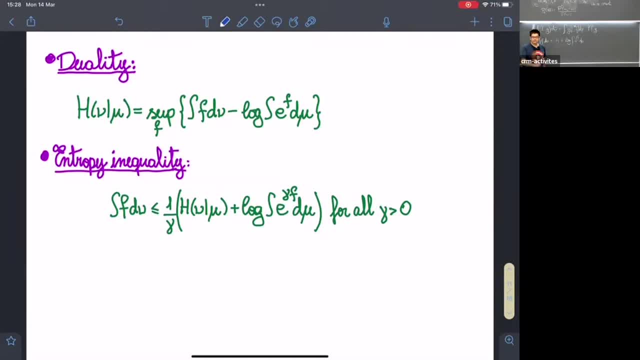 And these gammas that you tune make sense in many situations. Okay, So this is why it can be good to estimate the relative entropy between two different probability measures. Okay, You see, maybe computing this integral here with respect to mu is much easier than to. 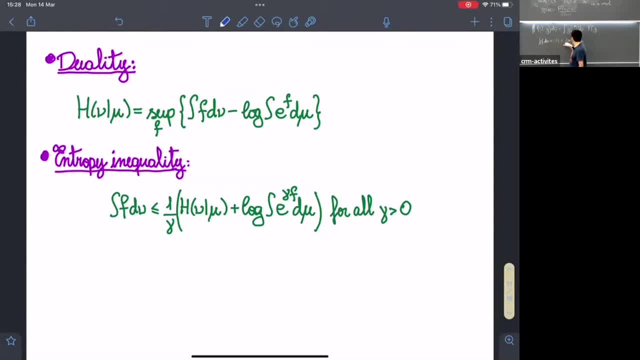 compute it with respect to nu because, for example, you know mu and you don't know nu. So that would be a good way. But if you want to do that, then you need to estimate the entropy. So you want to estimate this relative entropy in some way. 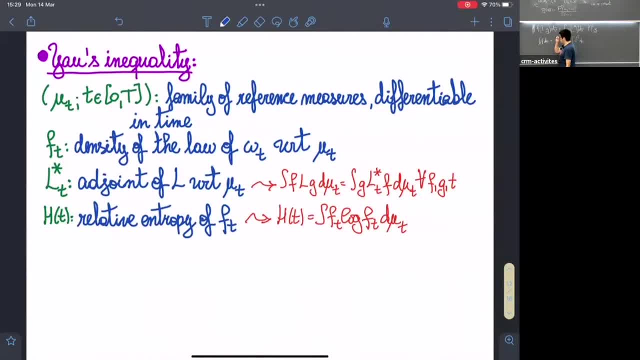 Okay, So what can you do? Now we enter into the kickstart of our approach, which is the so-called Yaw's inequality. Okay, So, what is Yaw's inequality? So the proposal is the following: You have a complicated Markov chain. 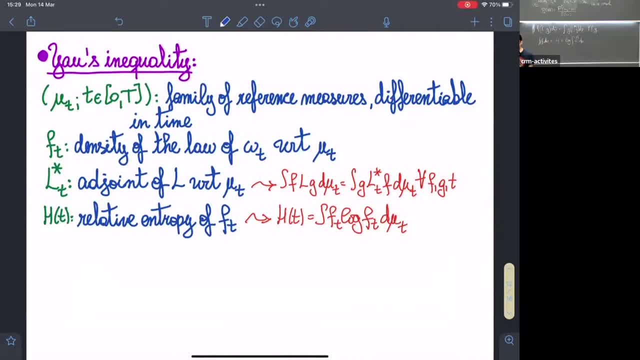 Okay, And you want to prove something about this Markov chain? Okay. So like, for example, some meaningful Loessner's numbers, some meaningful central limit theorem, And something you may or may not accomplish is to say there is a problem. 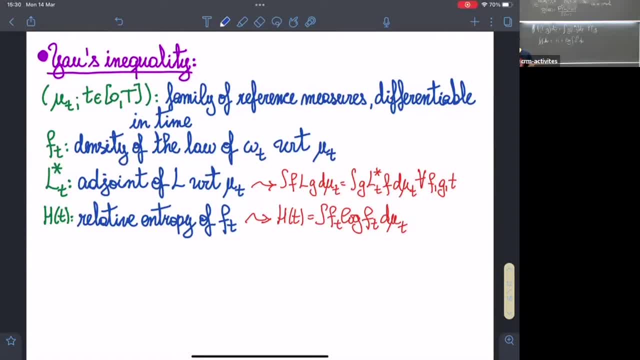 There is another, there is a family of measures- muti in this case I'm going to call it muti- which for some reason I have the impression that could be close to the law of my Markov chain at time t. 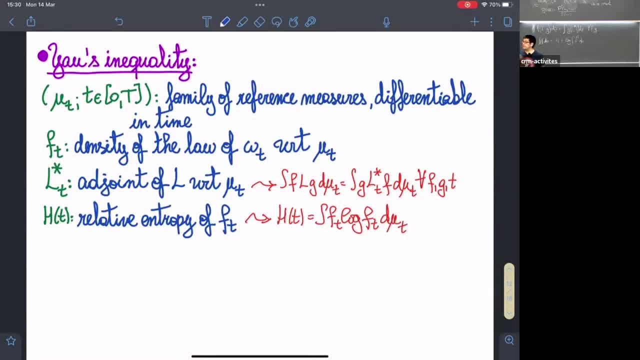 Okay, Because of, for example, when you are looking at a large scale limit, because you're looking at a perturbation of a known object- There could be some reasons for that- because, well, you need some computations and you can guess the limit of your Markov chain. 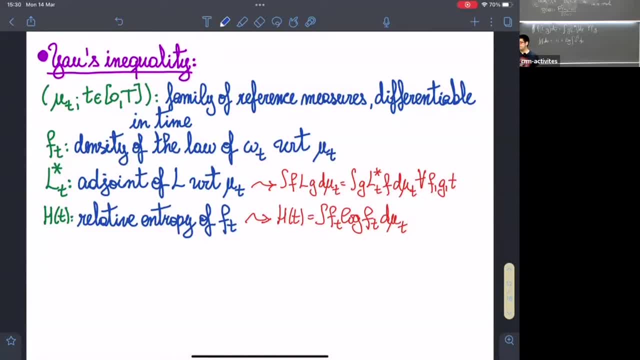 And you want to prove that guessing in some way. So what you do, one way to do that is to so your answer somehow. your try is going to be this: reference measures muti. Okay, Then the idea is to compare the relative entropy between the law of your process of. 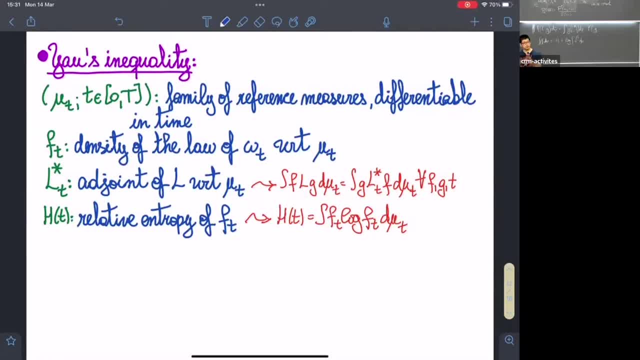 your Markov chain at time t and the reference measure muti. But the reference measure muti moves with t, So there's going to be some interplay there, Okay, And that thing there is accomplished by what is called the interplay. 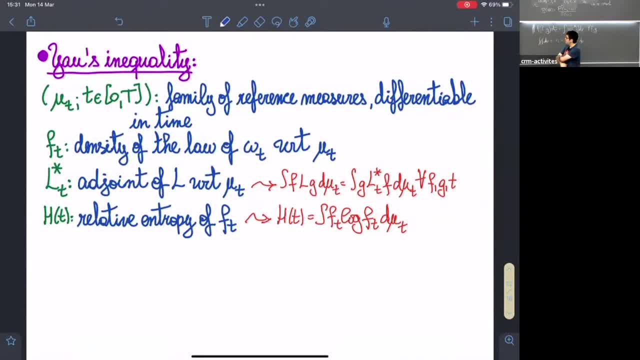 But what is called the inequality. Okay, So let me explain you the elements of this inequality, how this inequality works. So let me call Ft. So I need some definitions. Ft is going to be the density of the law of omega t with respect to the measure muti. 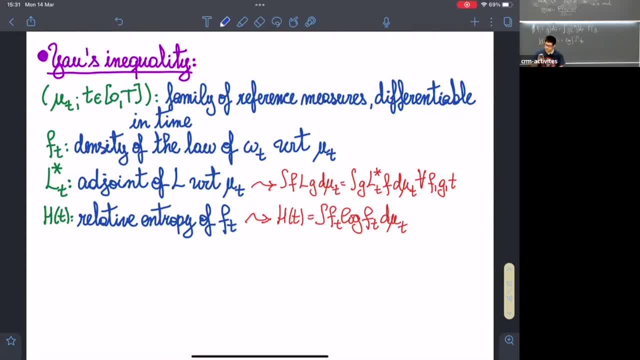 So notice that this is important, that in this setting the reference measure changes with time. So now I'm going to call L star of t, that joint of L with respect to muti. Let's remember that That joint operator depends on the reference measure you're using. 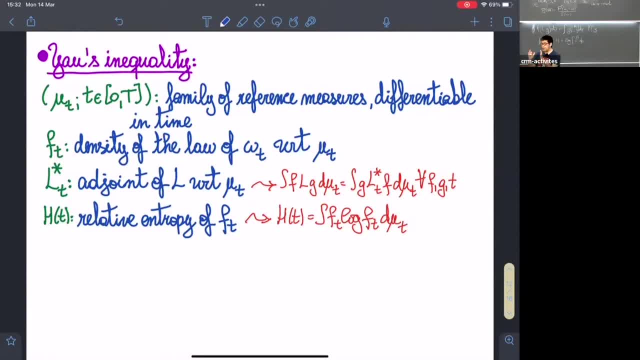 So here, when you take the joint of the generator L, you get something that depends on t, because the reference measure depends on t. So I'm going to call it L of t, star Okay, And I'm going to call H of t the relative entropy of F of t. 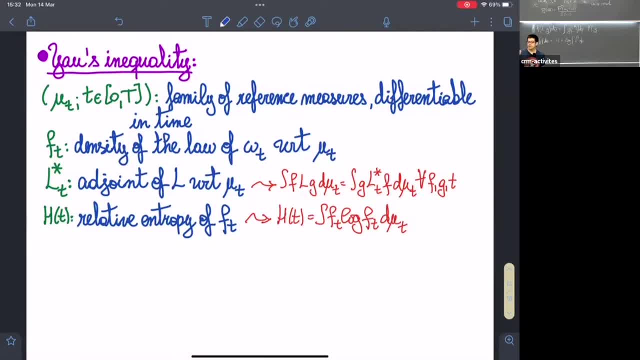 Okay, Or which is the same thing as saying it's the relative entropy of the law, of the process at time t With respect to the measure muti. Okay, So it's given by that formula there. Okay. So the idea now is: if for some reason we managed to find a family of reference measure, 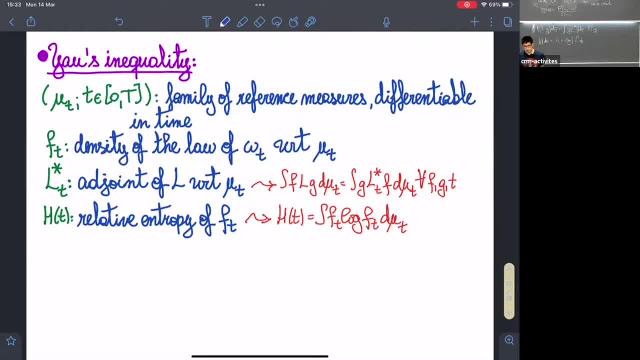 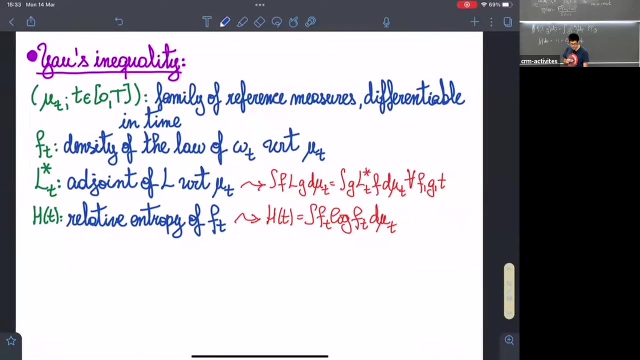 muti, such that the relative entropy is small and computations are kind of easy in some ways. With respect to the measure muti, Then we're in good shape to say something meaningful about our original Markov chain omega t. And what is nice about Yaw's inequality is that it puts that intuition into a concrete 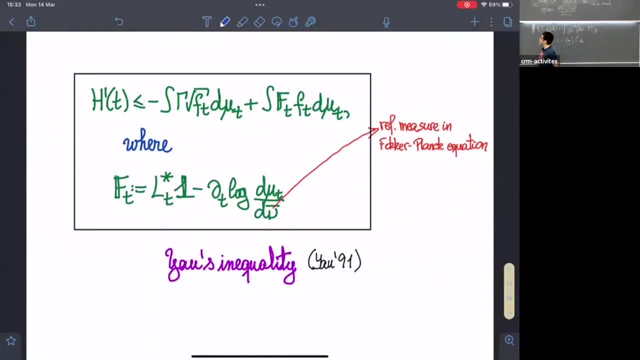 ground. Okay, So this is my Yaw's inequality. So The derivative of the relative entropy is smaller or equal than minus the integral of the Carré-Duchamp evaluated at the square root of F, t. So that's something that came out from the computations. 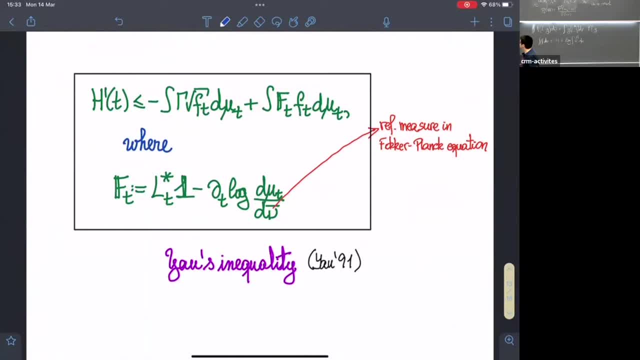 Plus another thing. Okay So, F t, F t, the muti Where F t is given by this formula there. Okay So, let's just analyze a little bit this formula here. Okay So, for a moment let us imagine that. 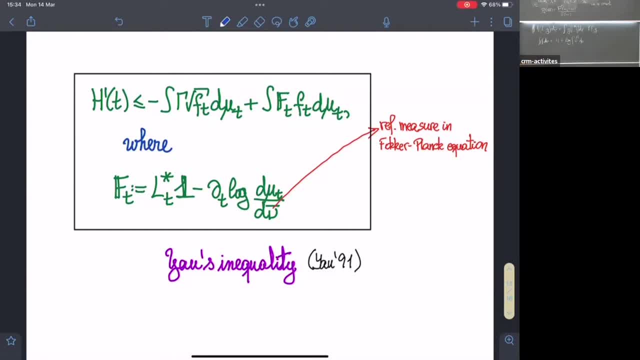 Let us take the case on which the invariant measure, The reference measure, muti, does not depend on time, So it's a fixed measure of mu. Okay, So there is no time dependence on the reference measure. Let's see what. So let's imagine that mu- t is equal to mu does not depend on t. 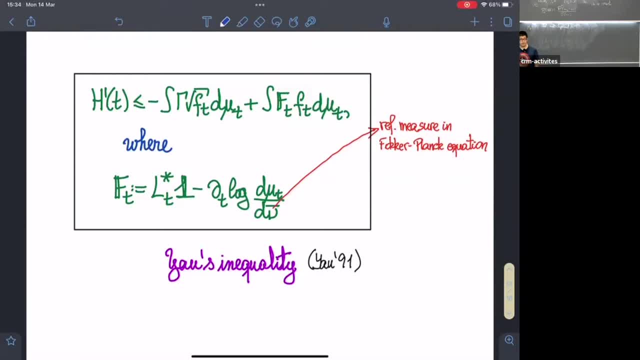 Okay, If this is the case, then this function F of t is just equal to L star of one. One here means the constant function equal to one. Okay, And what do we know about L star of one? So remember that I told you L star is the generator of a Markov chain. if, and only if, 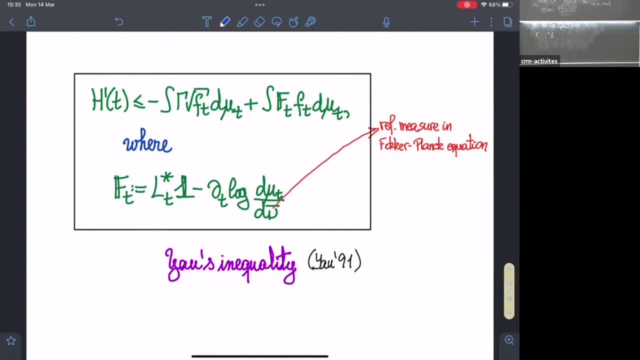 the measure mu Is invariant. Okay, So if the measure mu is invariant, is the invariant measure of the Markov chain, then L star of one is identically equal to zero, because L star is a generator Right. So this difference that appears in the definition of the generator gives you zero. 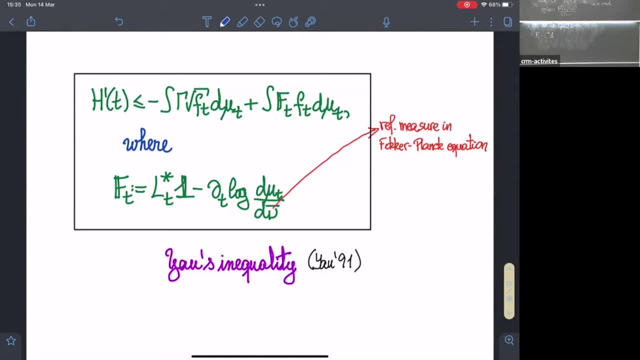 So F of sigma minus F of omega is equal to zero for any sigma and omega. Therefore you don't have plus term. You have anything there, Right? So you get that H prime is less or equal than minus that guy there, which is something negative. 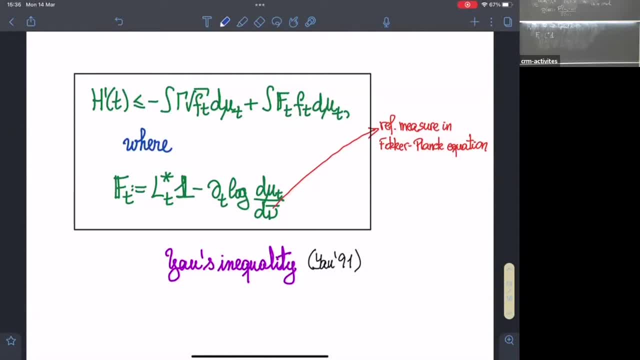 Okay, This is the. So we recover something which probably you heard about many times, which is that relative entropy is increasing in time. Sorry, Decreasing in time. Yeah, It always depends on the sign that you use to define the thing. no, 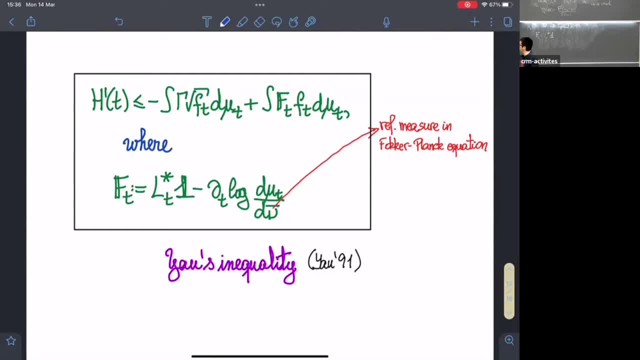 But it's truly monotone So it's decreasing in time. So you really go. So entropy is one way to measure how you go to the stationary measure, to the invariant measure of a Markov chain. So we recover that very well known fact. 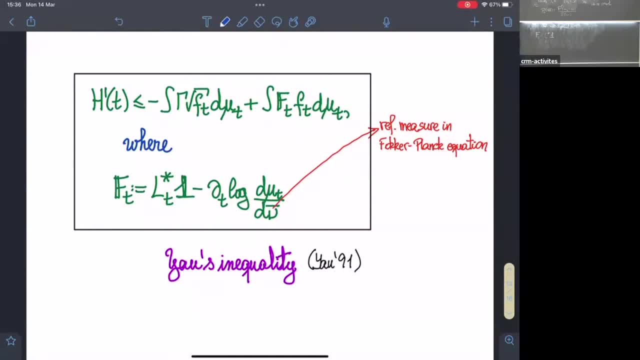 Okay So, And moreover, we have some information about how this indicates: No, So this, That guy there, The integral of, So this gamma square root of 50, is what people sometimes call the Fischer information. no, So the derivative of the relative entropy is minus the Fischer information. 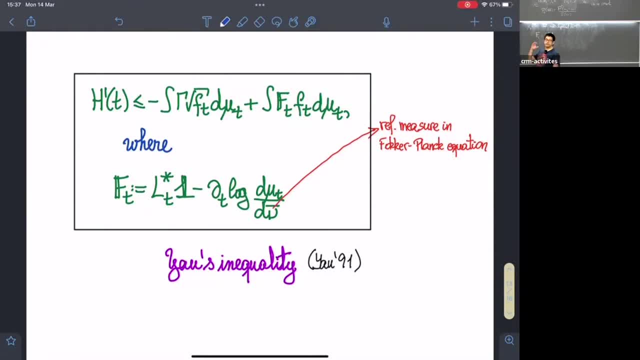 And of course this will be very well known for people that works in diffusion in stochastic calculus. They do that a lot. In the realm of Markov chains it's a little bit less known, But still It's still kind of standard. 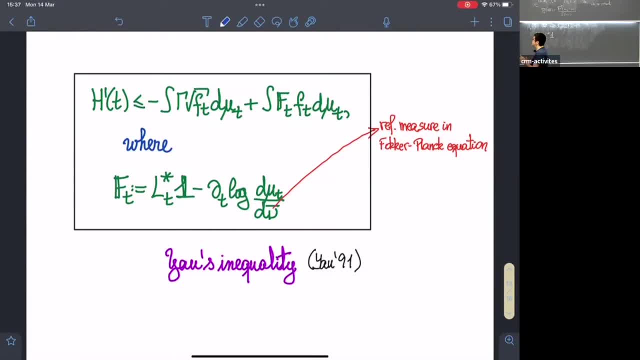 So the entropy decreases in time. And here there are some variational approach to equilibrium that goes by the name of Locke-Soverleif inequalities, that you can use to show how fast your chain converges to the stationary state Once you get here. in the case of 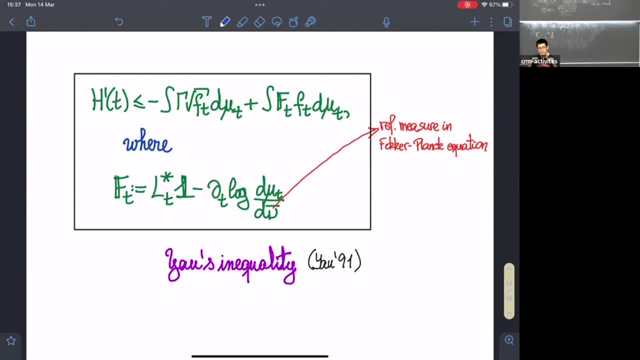 This is always Remember. For the moment I'm talking about the case on which the measure mu t, this reference measure, is constant in time and it's the invariant measure And the, So we recover that. So this joust inequality looks, at least in that sense looks to point in the right direction. 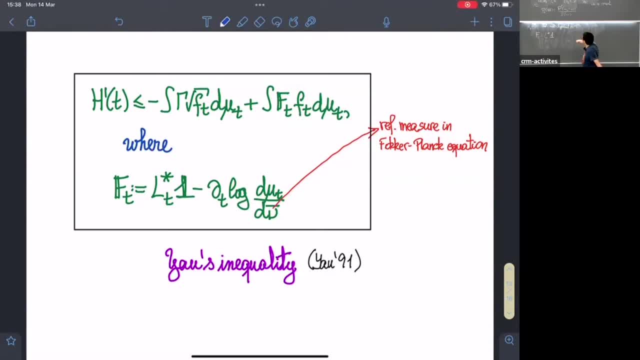 If the measure mu Still. let's think about this case here, where the measure mu t does not depend on t. So if the measure mu t does not depend on t, If the measure mu t does not depend on t, 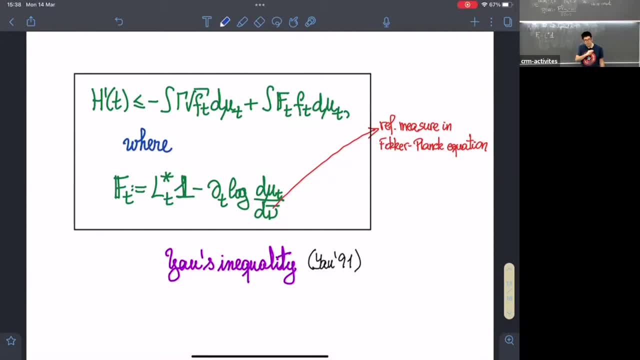 If the measure mu, t, does not depend on t, If the measure mu is not the invariant measure, this number there H of t, cannot go to 0. Because after a long time t, you are very close to the invariant measure. 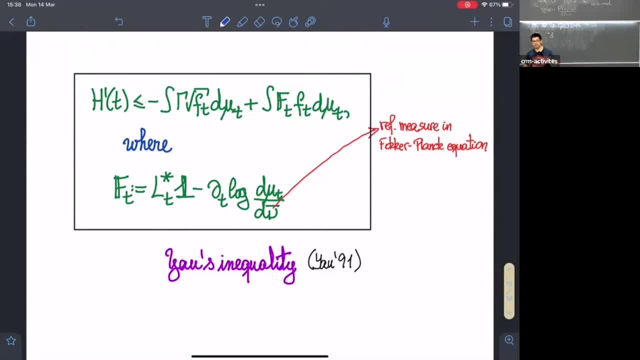 So the H? t has to converge to what? To the relative entropy between the invariant measure and the reference measure, which is different from 0,, because they are not the same. Okay, So then it is good that you have plus sums in there, right? 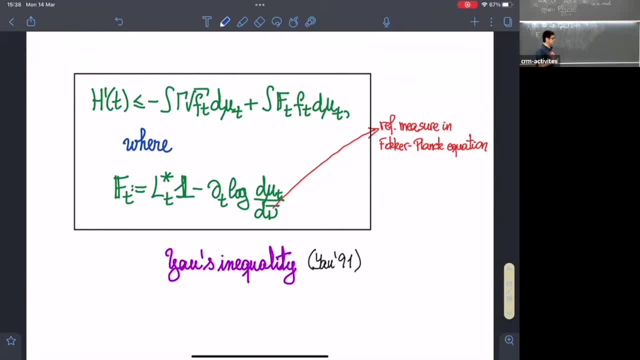 because that really takes into account that fact that in this formula the measure mu T is not necessarily the invariant measure. So sometimes this is something that I think I don't remember. it was Christina, was Hendrik, that mentioned that today. 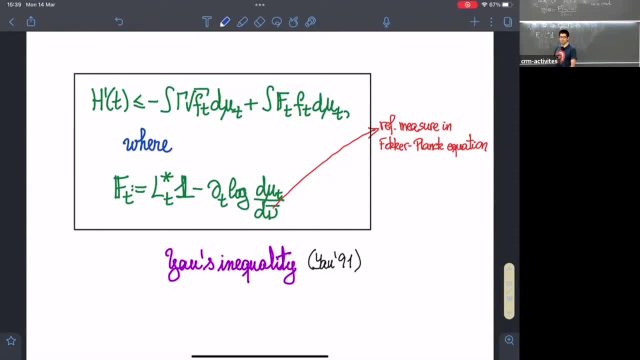 or maybe both. this thing about the energy entropy competition. So I like to see this formula here like as energy and entropy competition. So the first term the efficient information. it's akin to an energy, So it's negative. it pushes in the right direction. 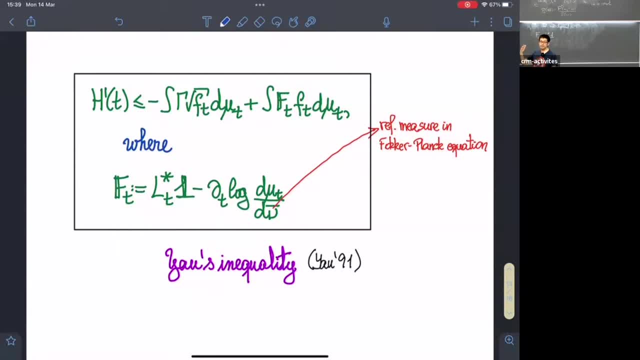 And the second term is akin to an entropy, So it puts you away of the region, The region of lower energy, somehow. And so what is really, really, really nice about this joust inequality is that the function F is explicitly computable, in the sense that here we have the freedom. 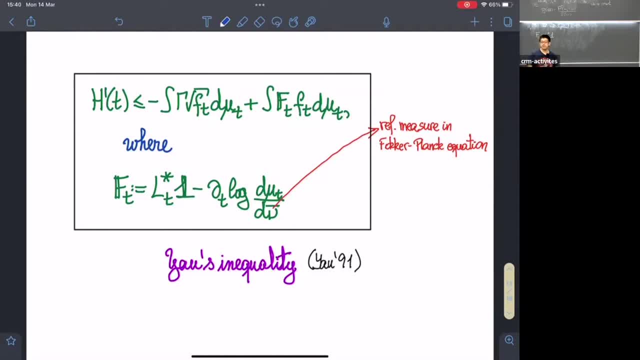 to choose mu T as we wish. So, in particular, we can choose nice measures, mu T for some reason. If you are in the realm of interacting particle system, maybe you take product measures because product measures are nice. Maybe they don't work or they are not the right ones. 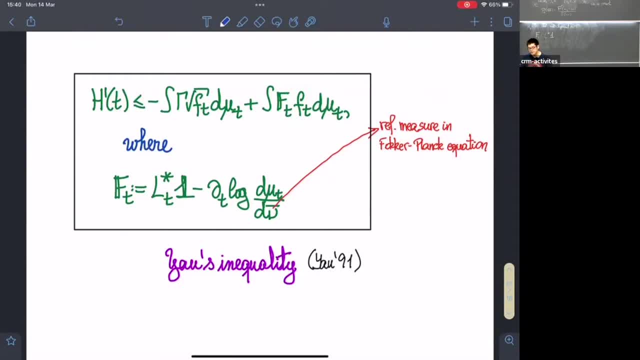 but at least they're nice. So if these measures are nice, it means that we can do the computation. So we can compute L star, We can compute L star of one, We can compute this derivative, extra derivatives, So there has to be some time derivative. 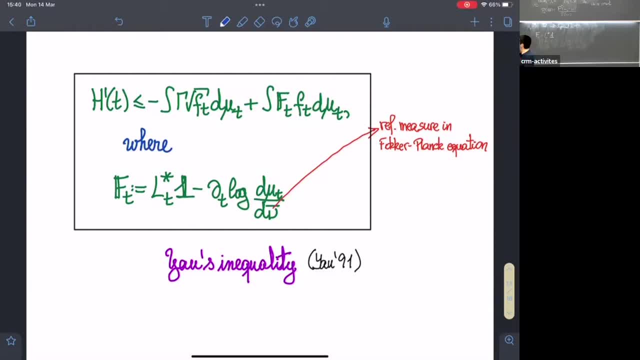 because the measure mu can depend on time, right. So it makes a lot of sense all of that. So in these aspects, joust inequality is a really nice inequality, because the function F is explicitly computable If you are put it as an input. 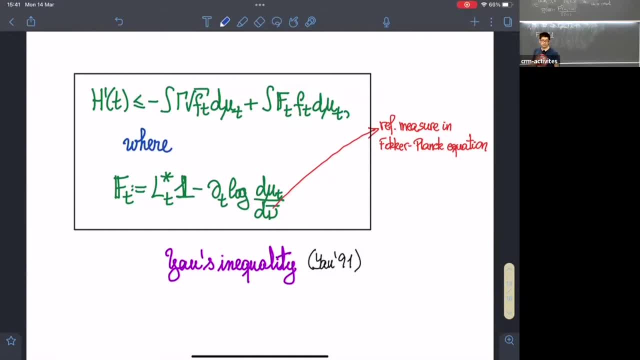 measures mu T, which are also explicitly computable. And this is: is there any relation between mu T and bad mu? Okay, so that is actually a very good question. So in this formula, bad mu has no importance at all, in the sense that the function F T 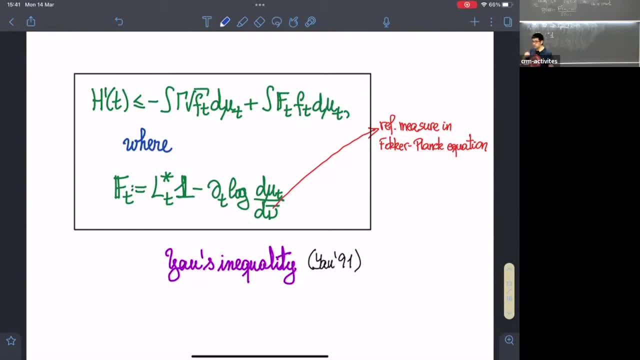 does not depend on bad mu. Okay, so what's going to happen? is that so if you take another reference measure, mu tilde, this radon encoding derivative that appears in the time derivative is going to be multiplied by an extra that radon encoding derivative. 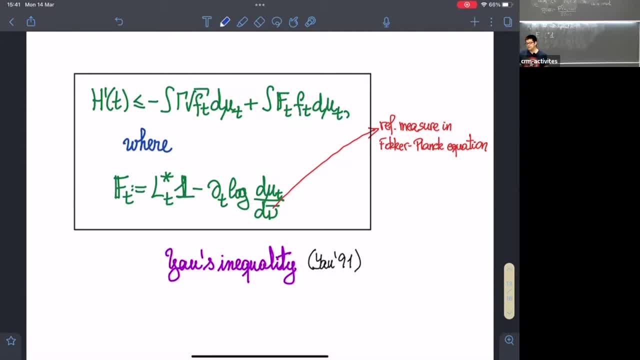 You take the log, then you have sums, And one of the sums- this this, this, this this this this- the radon encoding derivative between the new reference measure and the old reference measure has time derivative zero. Okay so, and that in that part. 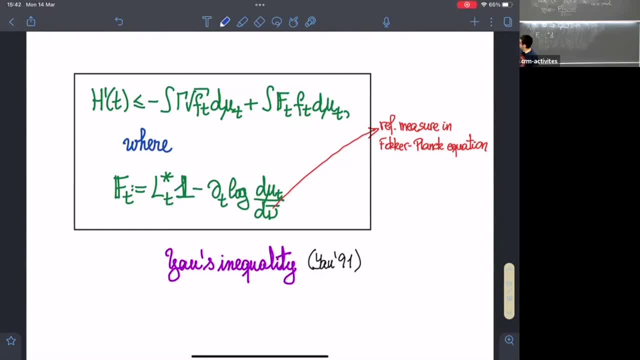 it doesn't really matter In the other guy. so L star T of one actually does not depends on new bar. Okay, so new bar is just a. it's a sort of artifice to make the function F, T, FT computable, right. 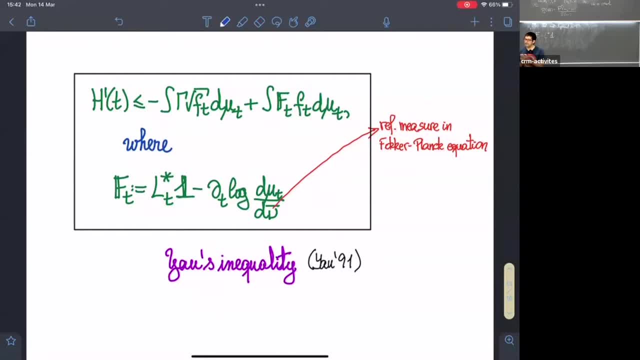 Because in many situations, what is easy to do is to say, for example, let's take diffusion on the real line. So what I'm going to do, how I'm going to describe the measure of muting, I'm going to give you its density. 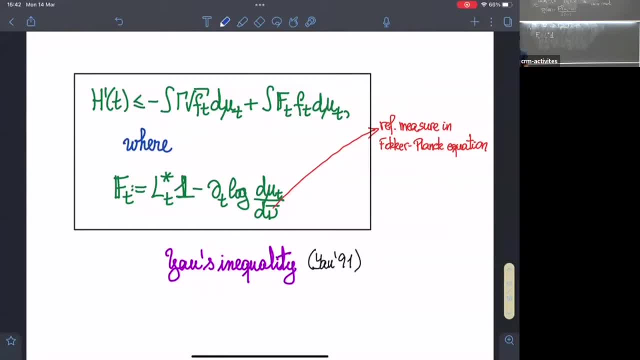 with respect to the 11 measure. That's a very reasonable way to define a family of reference measures. So this is what I want to do, And afterwards, when you do all the computations and you go and you compute the function FT, you discover that it didn't really depend on the fact. 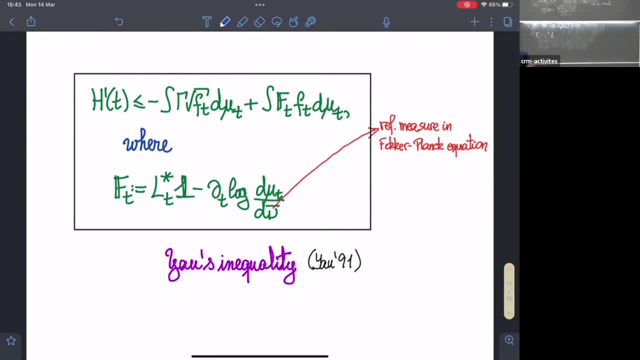 that you put Lebesgue measure there. You could have put something else, but if you put something else the computations are harder and the end canceled out. So it didn't really matter. So that's the role of the measured new bar. 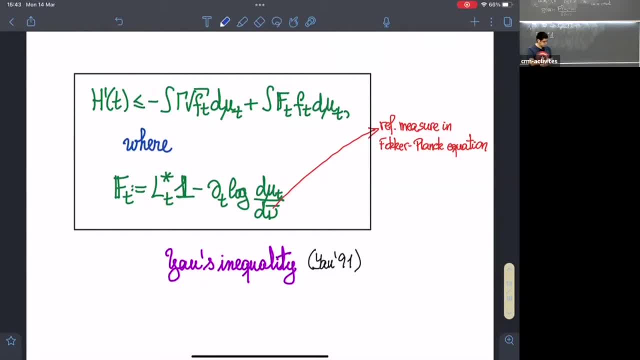 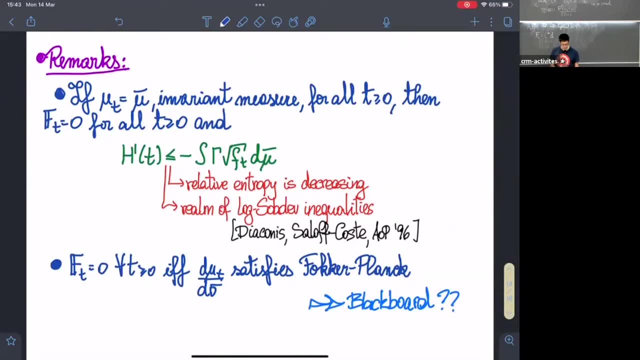 So that answer your question. Okay, so this is about the just inequality, So it's a really nice inequality. Some remarks, So this is just by basically a little bit of repetition of what I just told you. is that okay? so there's another question by Francesco. 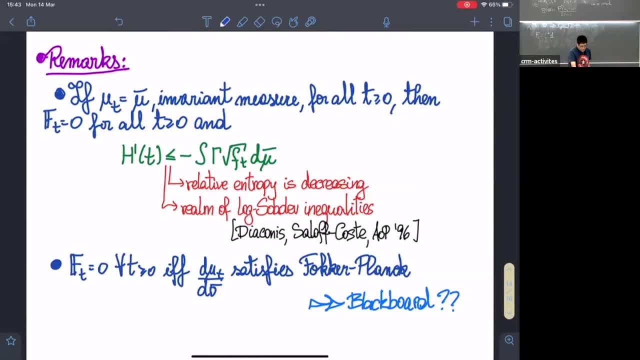 Let me see what Francesco is saying. So, when it is physically interesting to consider a family of reference measures, depending on time, do you have a concrete example? I do have a concrete example, And in fact I have various concrete examples, but so let me tell you the following. 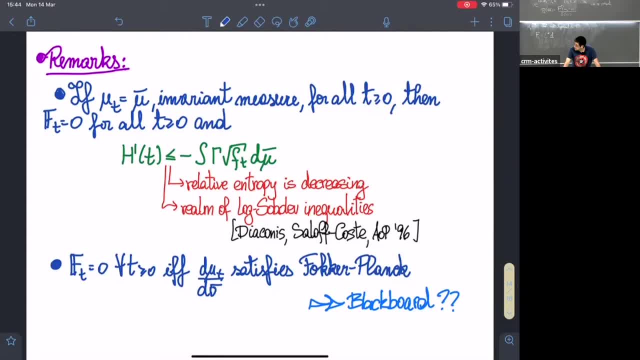 So let me think on a very, very quick example. Yeah, I think you have to wait, Francesco, until I do the examples, because I'm going to give examples of that And in the corresponding context, it's going to be very clear. 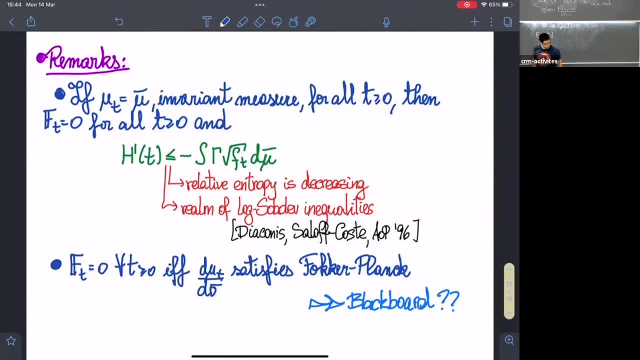 that they are physically relevant. Okay, so we can see that. So I was telling. so entropy is decreasing A little bit of a repetition of what I was saying. And so when you take as a reference measure there the invariant measure of your Markov chain, 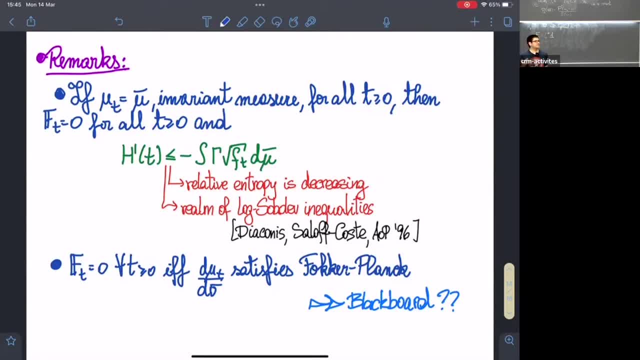 you get into the realm of lots of life inequalities. Okay, so there is a very nice survey paper by Diaconis and Salof Koste in analysis of probability of 96, on which they explain all of this. Okay, so it's a very nice paper. 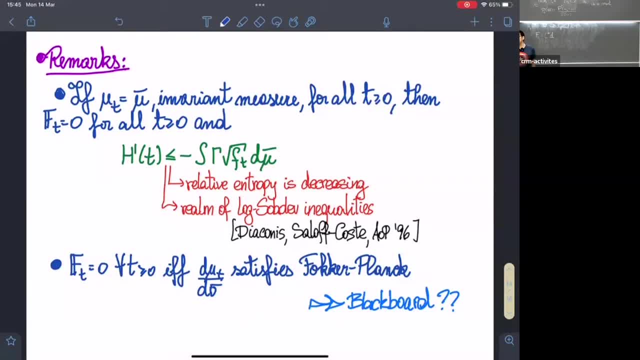 because they explain very well why, how you can use lots of life inequalities to get the estimates on the convergence to the stationary state of finite state Markov chains in that case. So for between finite state and continuous state Markov chains, when you look at that large scale limits, 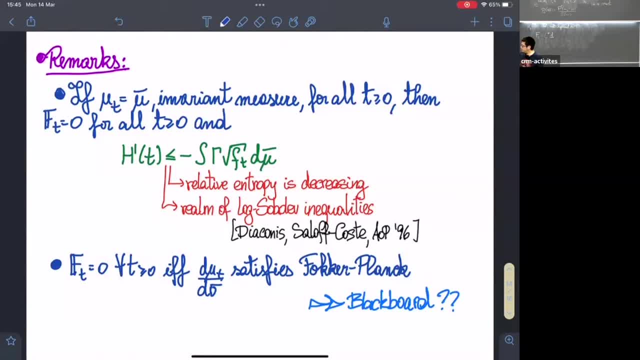 there's no difference, basically because you know there's a CLT for the Poisson process relating both, and then it's the same thing basically. So there in this paper you can get a lot more information and also pointers to the right references. 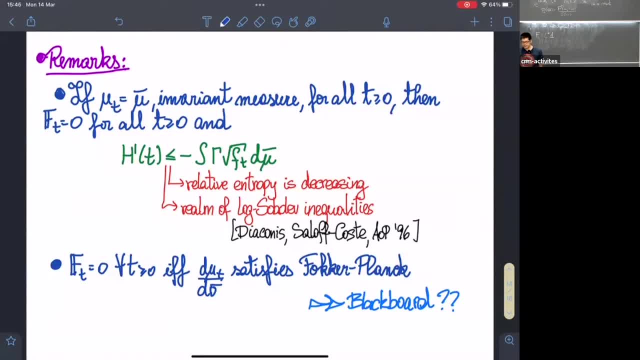 Now there are lots of names here, scattered names I can give you: Bakri, Emery, Ledoux, Laurent, Miquelot, et cetera. There are many guys that haven't proved lots and lots, lots of stuff about convergence to stationary states. 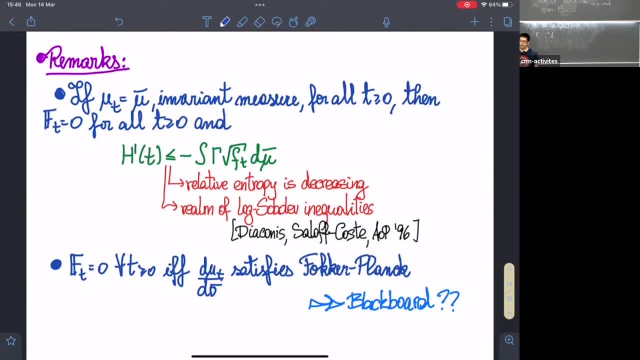 using this Locke-Sovlet inequalities or this type of idea. So we go by in a whole different community. they go by Fischer, information, inequalities, variation in inequalities, et cetera. Okay so, and and a very interesting remark is that 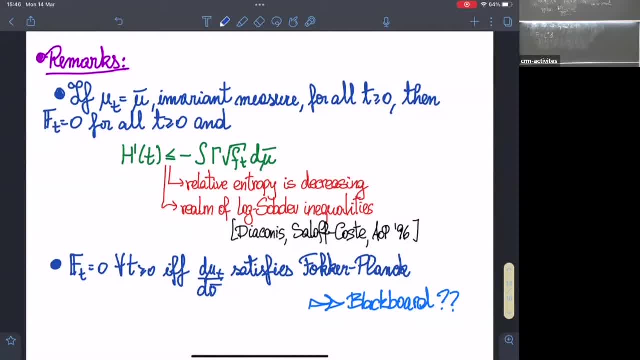 this function, Ft is equal to zero for every t. So now we are taking mu t which depends on time, If, and only if, this measure that this family's mu t satisfies Fokker-Planck equation. So Cedric is asking something. 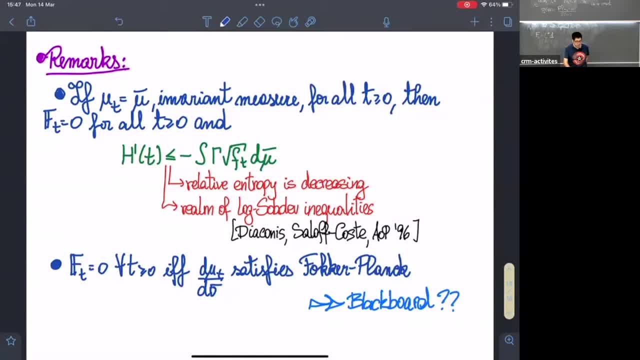 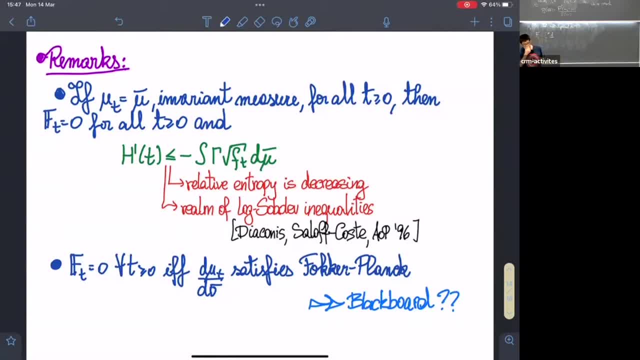 Why other convex conjugates pairs are not so interesting here. So this is actually a very good question. The answer is completely unclear to me. So, as an exercise, this is something you can do, You can, you can take, so you can define, maybe I of t. 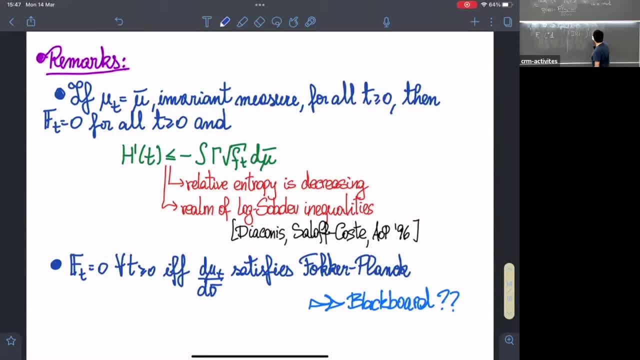 equals to the integral of F of t minus one squared equals to the integral of F of t minus one squared equals to the integral of F of t minus one squared, And then you get a completely equivalent. And then you get a completely equivalent. 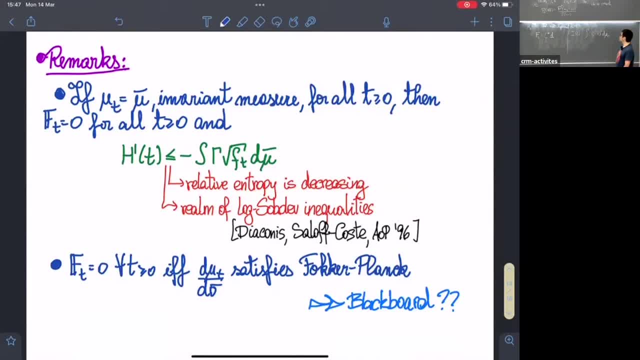 So you can hook up the equality in that case. So you can hook up the inequality, in that case, you will get something like this. you will get something like this: So it's minus maybe twice gamma of F of t. So it's minus maybe twice gamma of F of t. 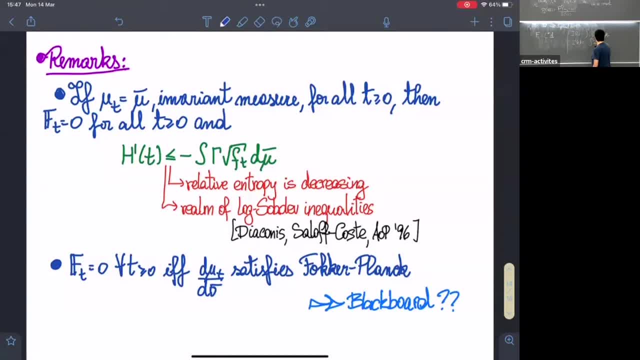 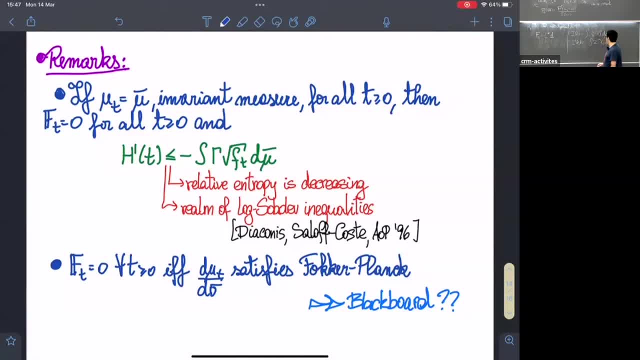 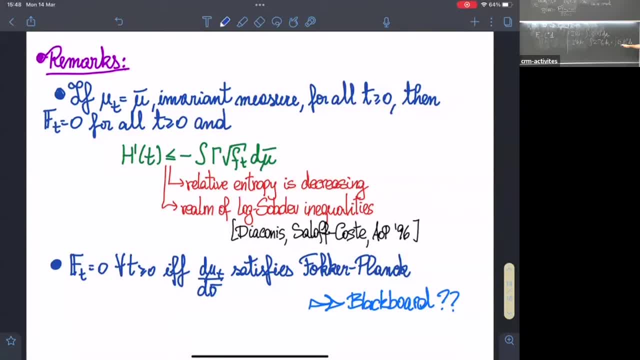 And here in the something you will see, you will see, you will see. so this is what happens when you take. so this is what happens when you take. so this is what happens when you take this thing here, this thing here, this thing here. 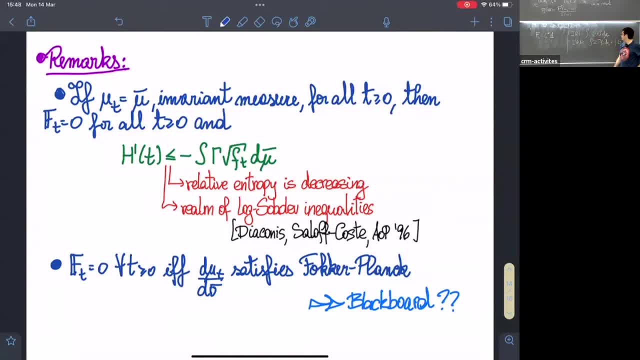 This is very natural today. This is very natural today. this is very natural today. the L2 norm: the L2 norm because it's always good to take. because it's always good to take the L2 norm, because we all know that. 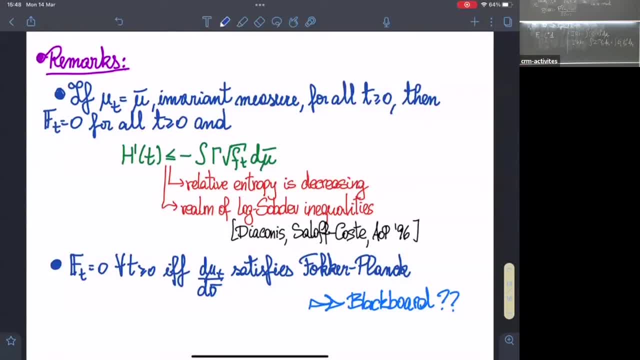 because we all know that, because we all know that there's some magic about. there's some magic about, there's some magic about the L2 norm, the variance, the variance, the variance. And what is the point here? And what is the point here? 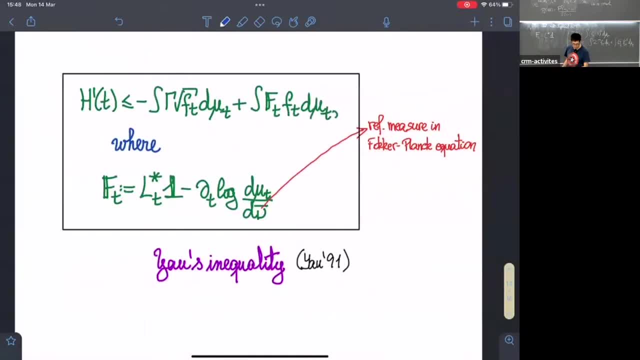 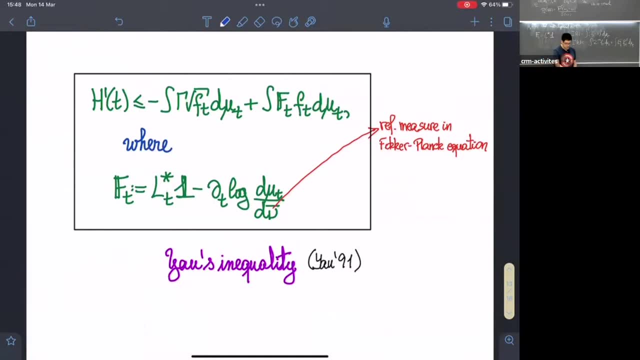 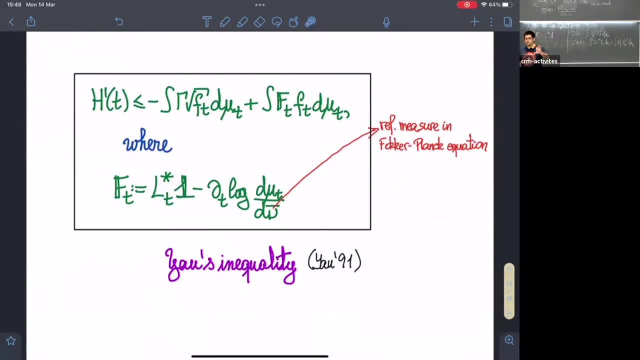 In Jou's inequality, In Jou's inequality in the error term, in the error term, in the error term, so in this term here, so in this term here, you get your function, you get your function, you get your function. 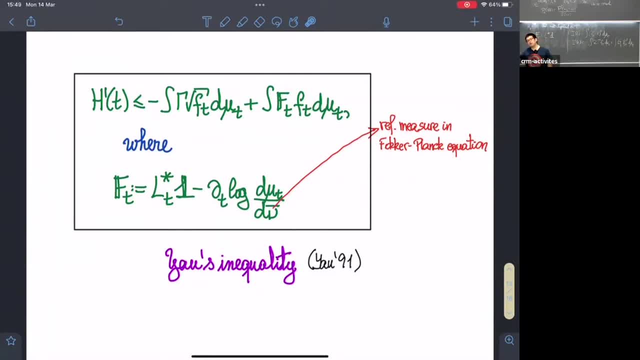 your error function. your error function: big F, big F. integrated again, integrated again, integrated again. is you don't get that, is you don't get that because? because, because you get, you get, you get the. the fe square here, the fe square here. 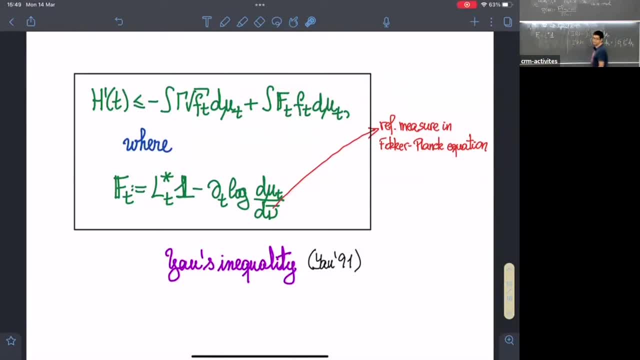 the fe square here. So So, so you cannot bound that guy. you cannot bound that guy by something, by something times the times, the this guy here functions- and maybe you're more clever than me. I tried to do that and the only one that. 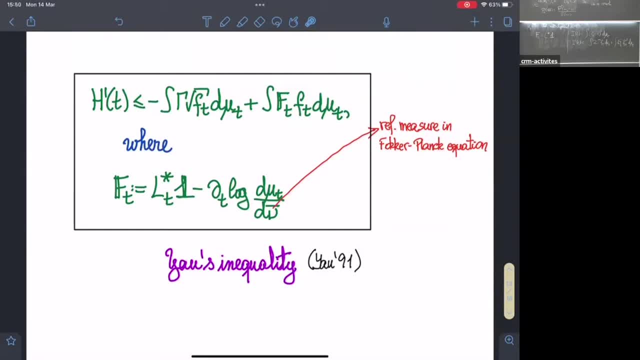 gives you room is the entropy. It gives you a lot of room, but a lot of room is a lot more than no room at all. It's really a lot more. Okay, so Cedric is satisfied. Okay, that's good. And so maybe in some situations- maybe you have additional estimates that allows- 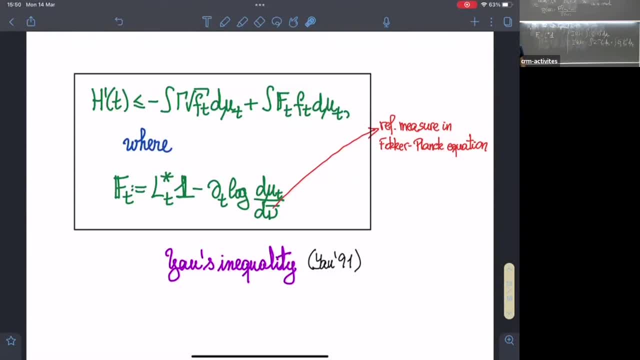 you to make better estimates. Okay so, this is So in PDEs. people do that They get a priori bounds from other methods and because of that they can use better feature information. So you can use better bounds, better norms here, Okay so. 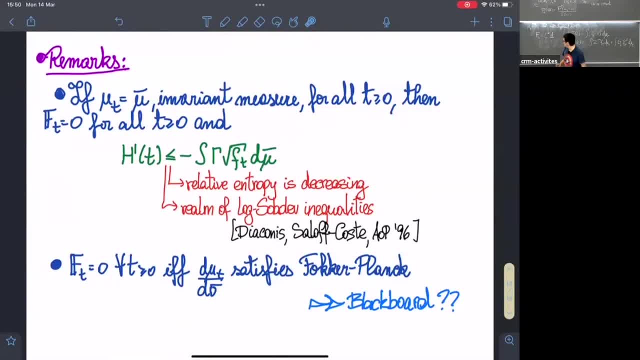 Ah, okay, so this is the end of my slides. What did I say? Ah yeah, blackboard, Blackboard. Ah, okay, so I was just about to. So now, I was just about to do this very same computation. 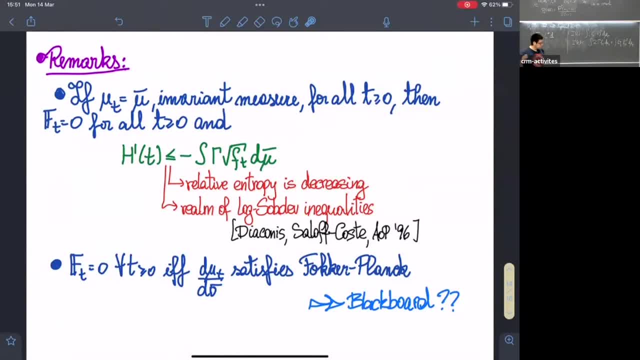 that Cedric told me. so that's good, because I already did it. So I have still like nine minutes left. so I think I'm going to stop here for the moment, because, well, I don't know you. but 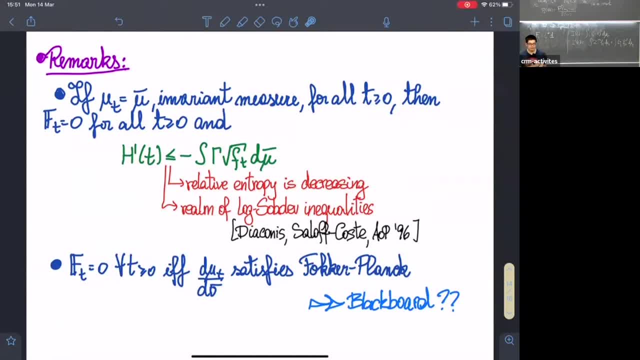 But I think it's also three one hour and a half mini-courses. It's a lot, So I'm going to. So what I want to do now is to make a poll, okay, Because? So the slides for tomorrow, as you see, are not written yet, so this is the first slide for tomorrow. So 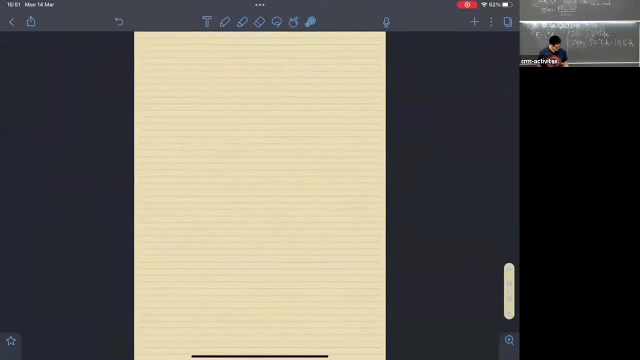 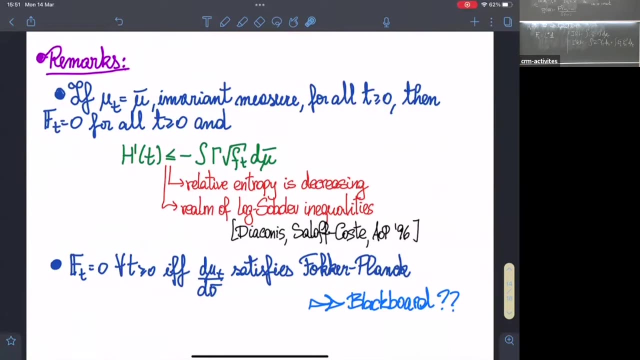 I haven't even formatted into the right format, no, Okay. so, Starting from tomorrow, I'm going to do, I'm going to focus on one particular example to tell you how these ideas work. So today, I really wanted to give you this. I know. 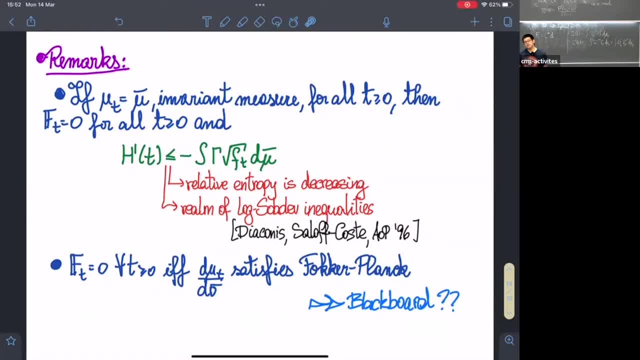 it was fast, but everything I just told you is completely elementary, in the sense that there is nothing fancy. All that you need to do here to do, For example, if you want to prove the inequality by Okay, On your own- well, there are some tricks that you need to know, but there is nothing difficult. 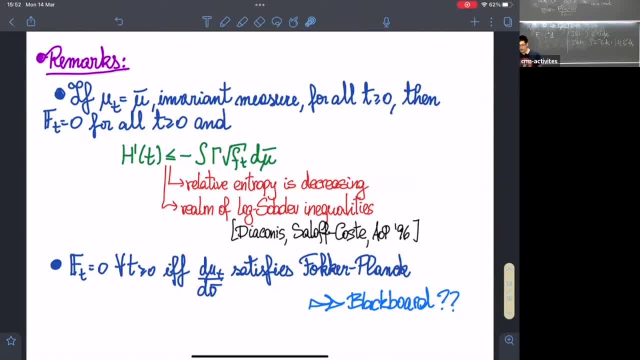 about it. It's just a very long exercise in calculus one. So you have to use Fokker-Planck to take some derivatives, and then you arrange terms, do the usual tricks and at the end of the day you get this estimate. 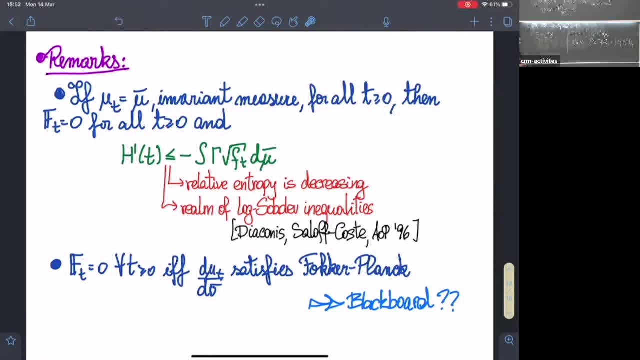 Okay, And so the audience is very heterogeneous. so we have students from many places of the world. So I really want to ask you guys, what would you prefer for tomorrow? Okay, So, let me tell you what is on the menu for tomorrow. Okay, So, what's So for tomorrow? I have 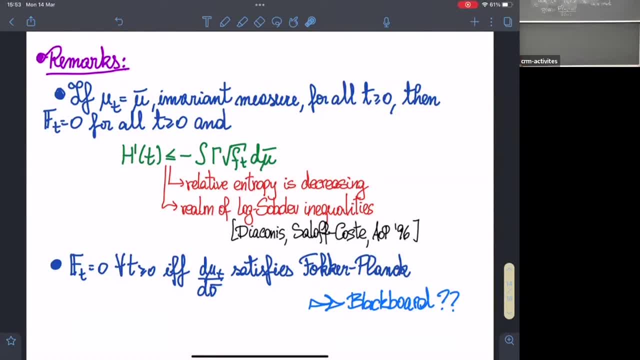 solved. I mean not for tomorrow, but for the rest of the NIC also. So the idea is that to focus on one particular example and try to develop it as far as possible. So we have three options, okay, Option one, a Curie-Weiss model. So in Curie-Weiss model there are 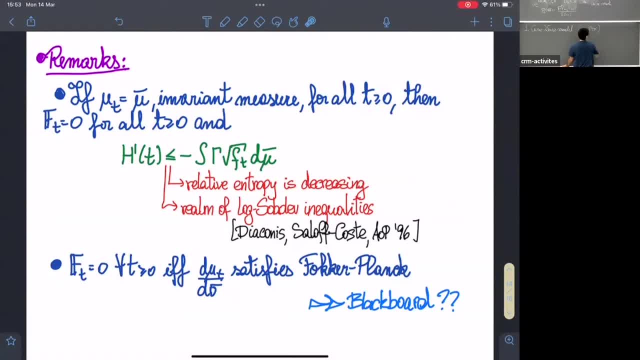 no PDEs. Okay, Well, actually some PDEs, Little Okay. So option two is a reaction diffusion model. So this guy has some SPDEs. Okay, Okay, Okay, Okay, Okay, All right. 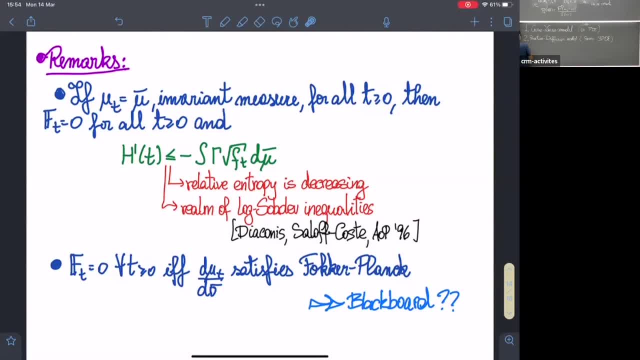 Okay, Okay, Okay, all right, But not that much. And the second one is so-called boundary driven, And this guy here has more SPDEs, Okay. So there are these three examples that they. So the idea is that the first one keeps technicalities. 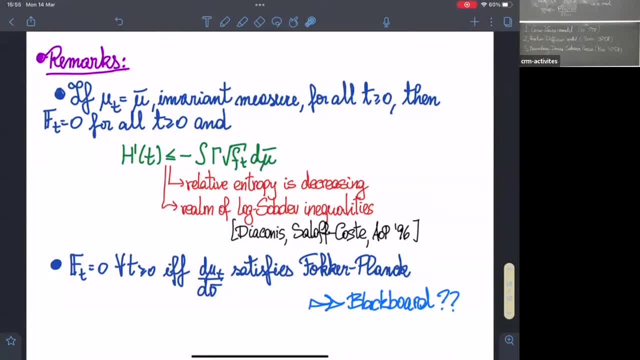 to a bare minimum. so it's basically So. you were already introduced to Curie-Weiss model what Hendrik explained today. So it would be like a more extended version of what Hendrik did today, more detailed. So the second one it's. so I don't know if you- probably you were here. 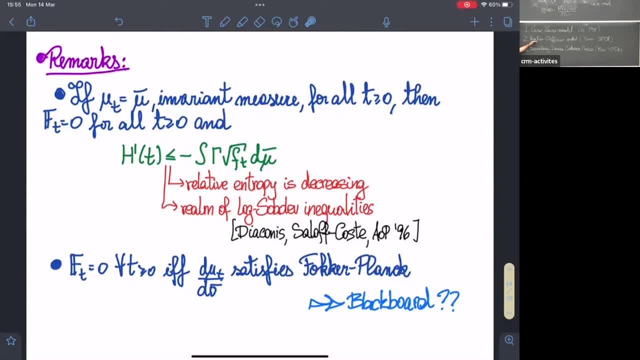 I gave a seminar a few weeks ago about this reaction diffusion model here at the CRM, And so the main idea is that we want to understand the scaling limits And, as you've seen in Cedric's talk, when you look at the Curie-Weiss model, what you're obtaining- 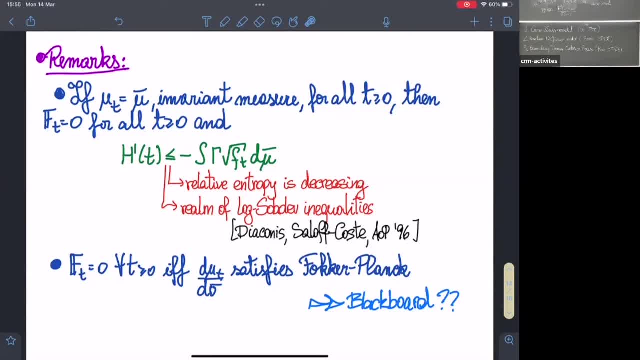 in the right scale is a stochastic differential equation And you have to analyze this stochastic differential equation somewhere. If you look at the reaction diffusion model, so there are actually diffusion models. now there is a space, okay, But there is a PDE. but the point is that the stationary state of that PDE is constant in space. 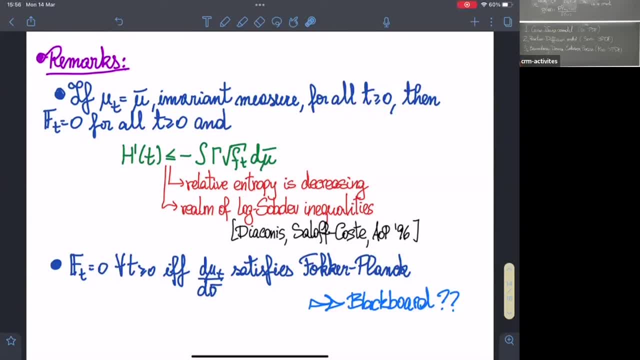 So using that- the stationary state of the PDE is constant in space- you can get rid of the spatial dependence somehow. So this is still a model where the space plays a role, but many of the technicalities can be hidden by the fact that the stationary state is. 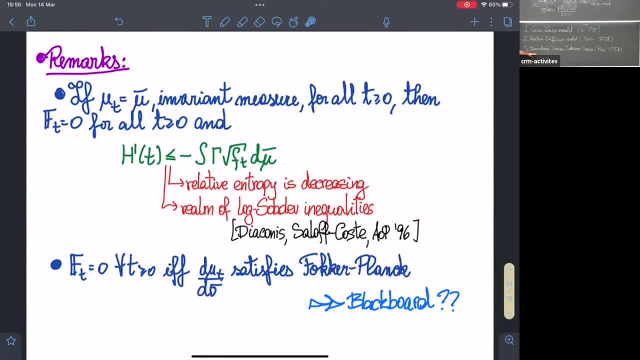 it has to be translation-embedded. And then boundar delivery, distribution process. it's so you heard that I think about, maybe maybe you know about. distribution process is well, if you don't know, it doesn't matter, I just tell you very quickly. I say it's a model for this. 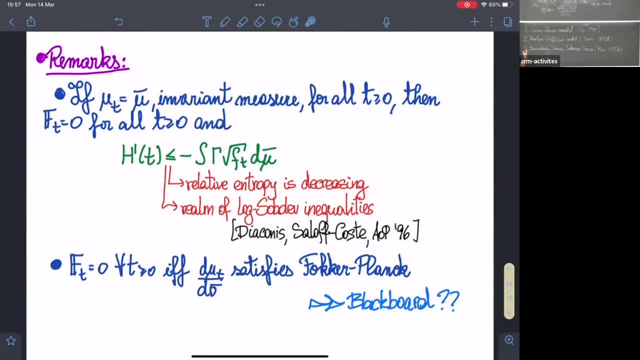 is this heat transfer between two heat dots. that was mentioned before. So you have more than here. heat means density of particles. You have more density of particles on one side of an interval of discrete interval, less particles on the other side, and particles can enter and they move inside. 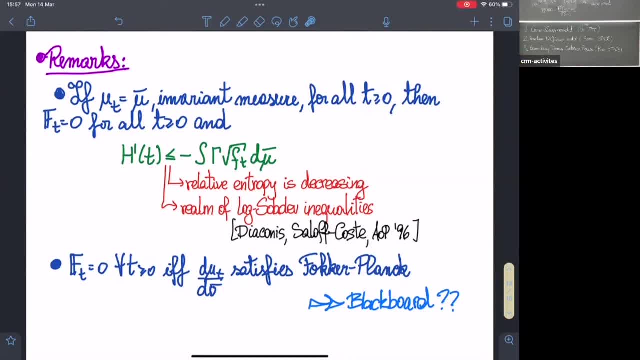 doing some sort of random work with interaction. In that case, the stationary profile of the associated partial differential equation is not constant in space. So then there you have to go to the full strength of the theory we're trying to develop. So those are the options for tomorrow. 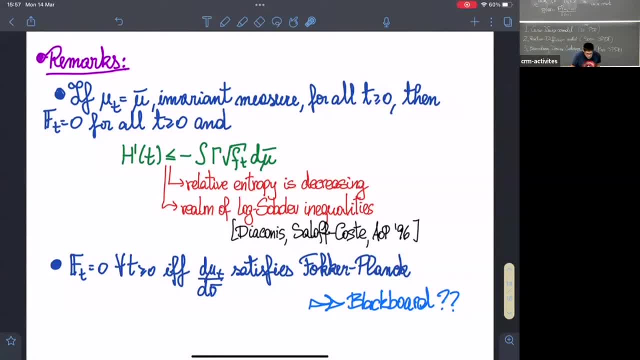 And so. So for people online there is the possibility to vote. So C for Curie bias, type R for reaction diffusion models, a type E if you prefer, boundary driven exclusion processes, Okay. And C also for people in the room. 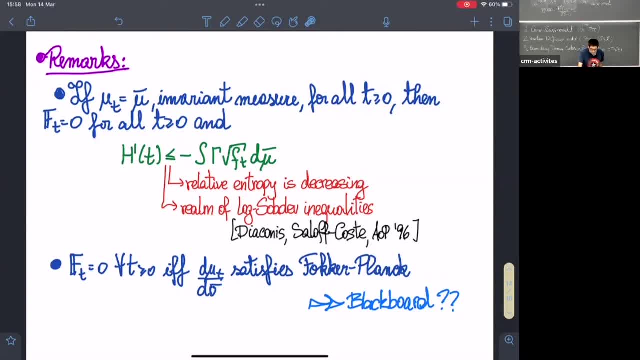 So we can count the people here. So who is for the Curie-Bice model, One Curie-Bice. So. who is in favor of the reaction diffusion model- Very good. And who is in favor of the boundary driven exclusion processes and the Curie-Bice model? 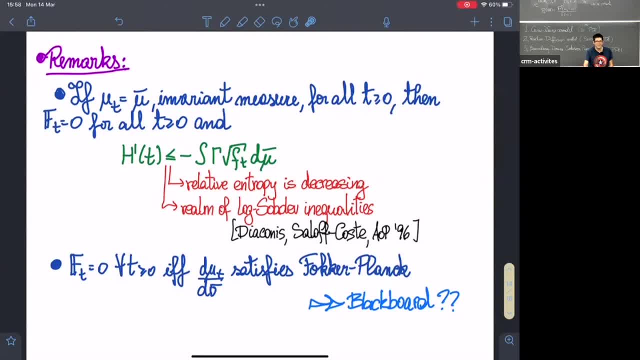 Okay, You can vote also twice, probably. I think Okay, And it seems to me the majority here is prefers the reaction diffusion model and maybe Richard can update us about the online. So For online it's 10 for reaction diffusion. 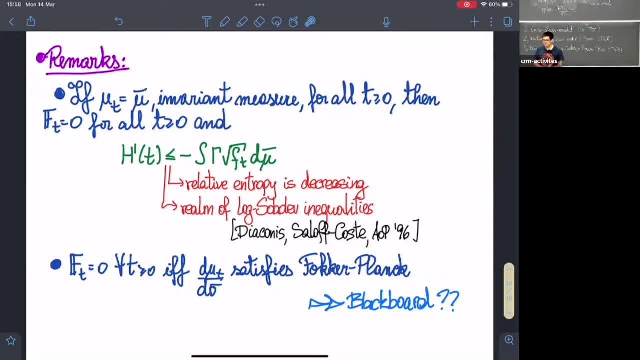 six, five for Curie-Bice and four for sorry, 10 for Curie-Bice and four for Curie-Bice And for the boundary driven exclusion processes, and they're about five each for the most, one to-. 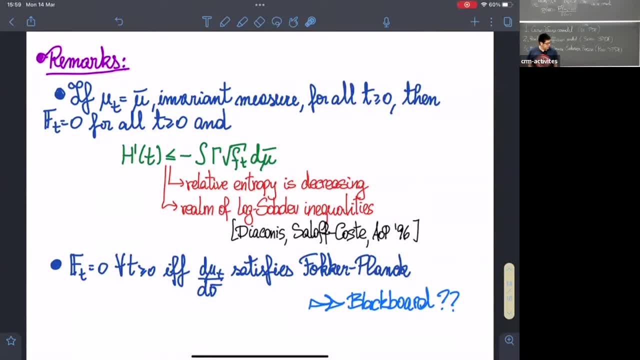 Okay, That's good. So well, of course. So how is that called? It's a. how is the name? how do we call it? It's a non-vinculant plebiscite. no, So how do you call that in English? 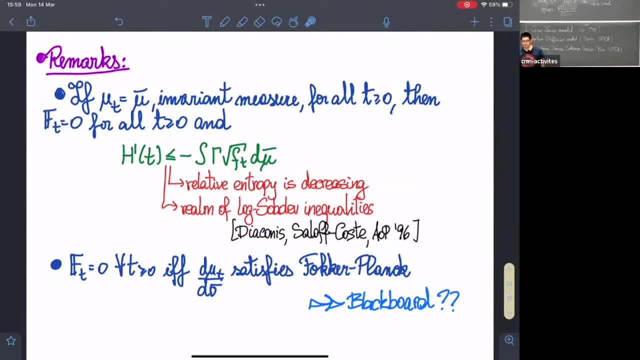 I don't know this plebiscite that you do. what is it? I don't know. My name is Gavane. my name is Gavane. I don't know, My name is Gavane. My name is Gavane.